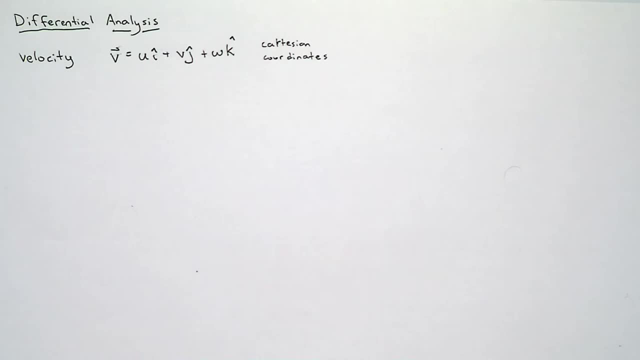 we're going to focus on on Cartesian coordinates for now and then, depending on how our problems are arranged, we may choose to use any other coordinate system. We also reviewed the material derivative And, if you remember, the material derivative was a rate of change. 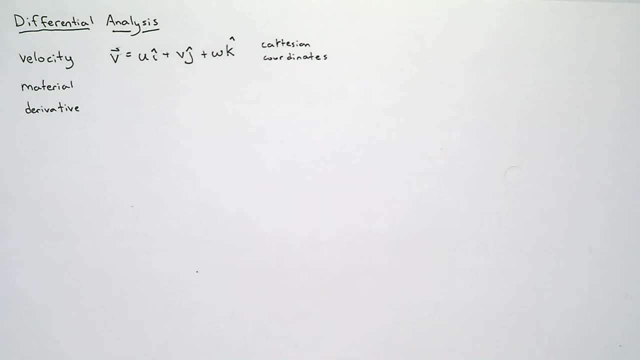 a rate of change that followed a Lagrangian particle through an Eulerian space. In other words, the material derivative is kind of the derivative that looks at a particle from a Lagrangian perspective but as if it were moving through an Eulerian space, kind of combines both and 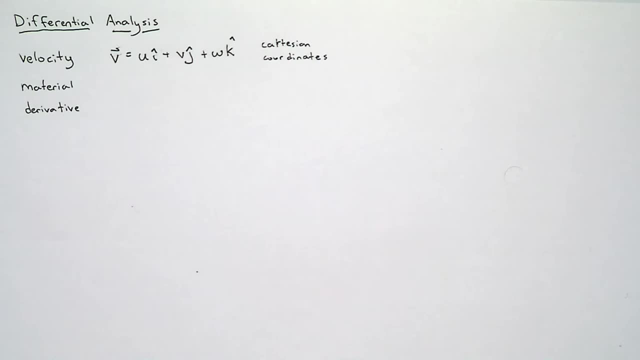 you notice, because in this derivative which we find by applying the chain rule, we look at changes not just with respect to time but also with respect to space. so that derivative- we can write it right here- was simply equal to a change with respect to time. This is what we call the temporal derivative. 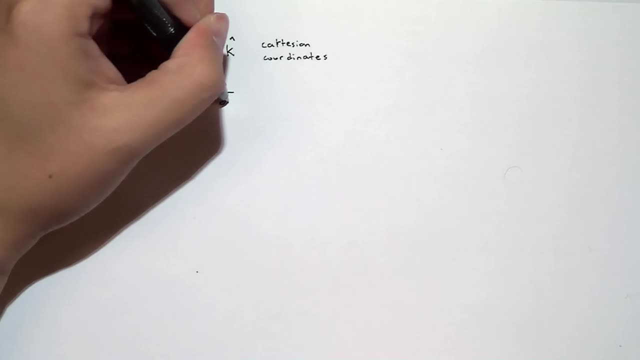 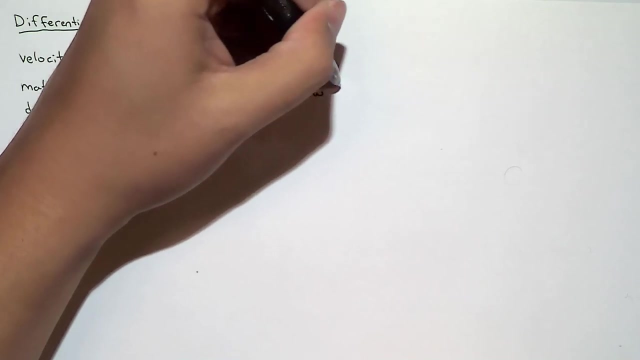 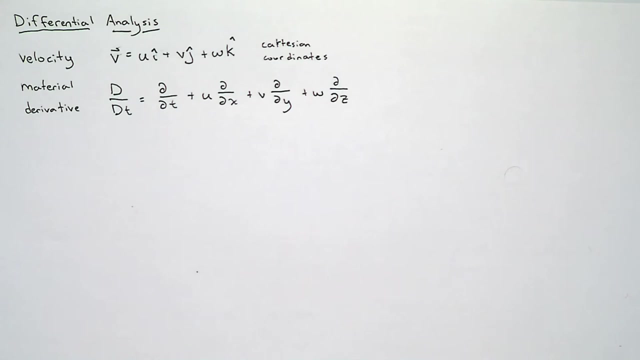 plus the flux or change of a property with respect to space. So I'm going to write down these spatial coordinate changes. Remember this is all Cartesian coordinate system, So this was the material derivative. And remember that this is an operator And because this is an operator, we need to apply it to some sort of vector or 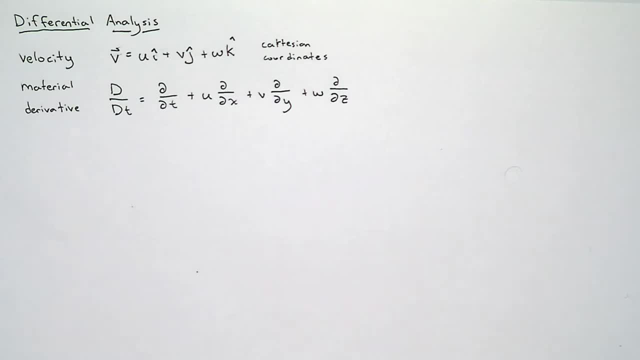 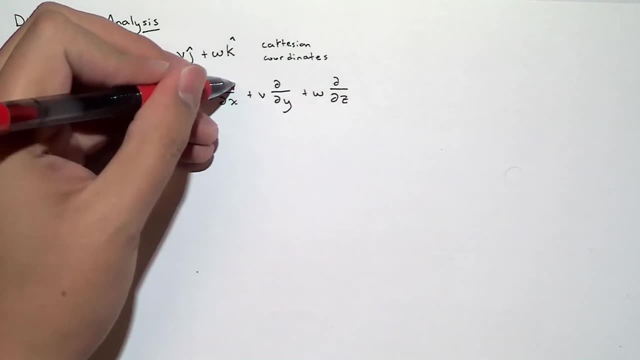 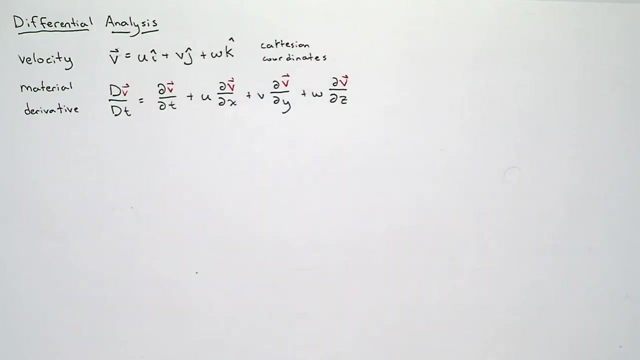 scalar field. One example we looked at was applying the material derivative to the velocity field, And when we applied the material derivative to the velocity field, we can essentially see how velocity changes with respect to time and with respect to space. Do you know what we called? 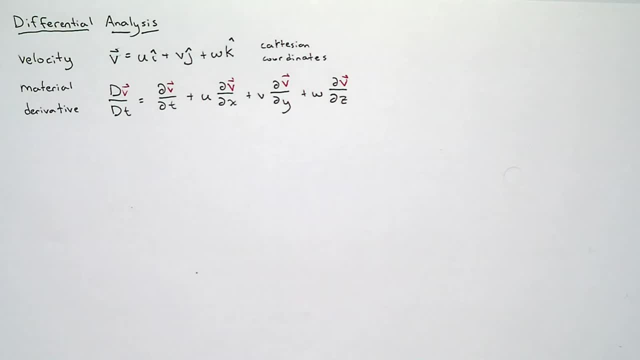 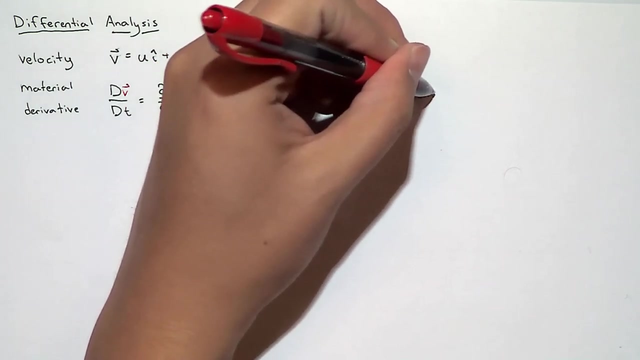 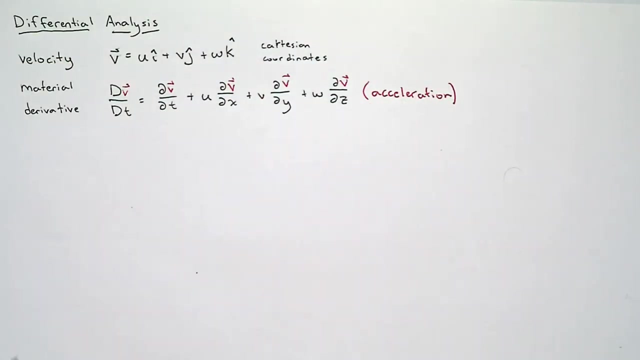 this derivative, The material derivative of velocity with respect to time, The acceleration, Thank you. So the material derivative of velocity with respect to time is simply acceleration. Now, the reason I'm distinguishing these two colors is because this is an operator. These black letters are operators that we can. 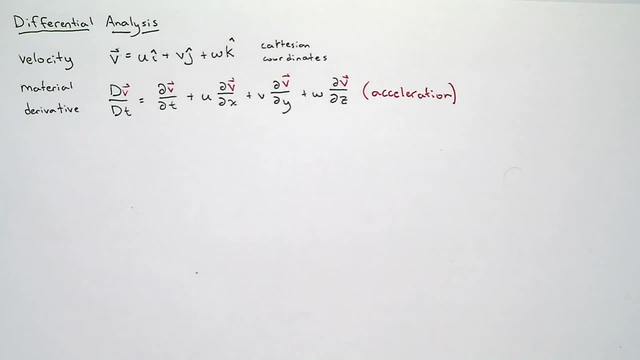 apply to any property. So you can take, for example, the material derivative of velocity, my vector in red, or you could pick any other property and find its material derivative When you pick any other property and essentially the only thing you have to change are the red. 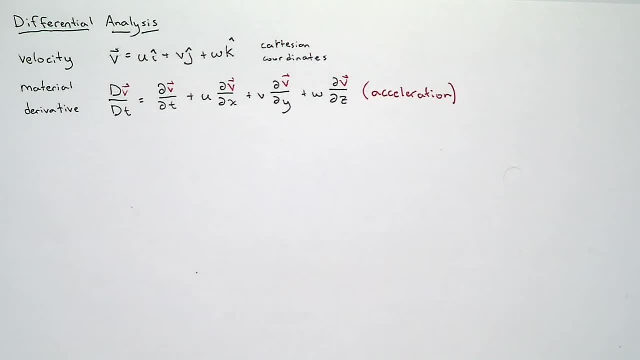 parts, because you're applying this operator into any property. So we looked at the gradient and we defined the gradient as the change of a property with respect to space across a spatial field. And we found that we can calculate the gradient of any property with an operator called the del operator. Now the del operator, which again 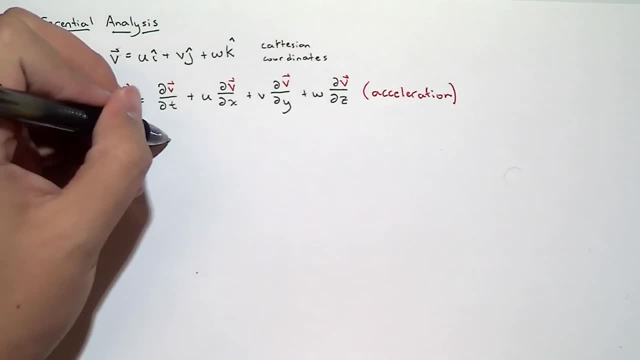 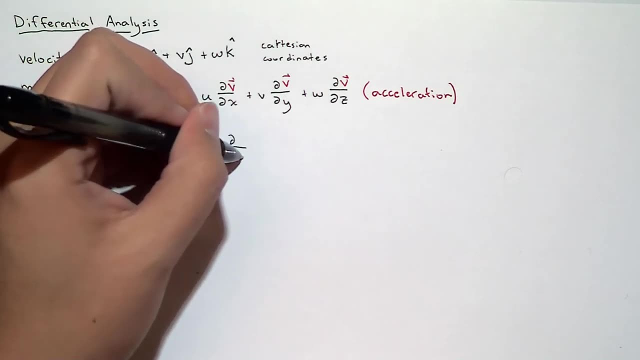 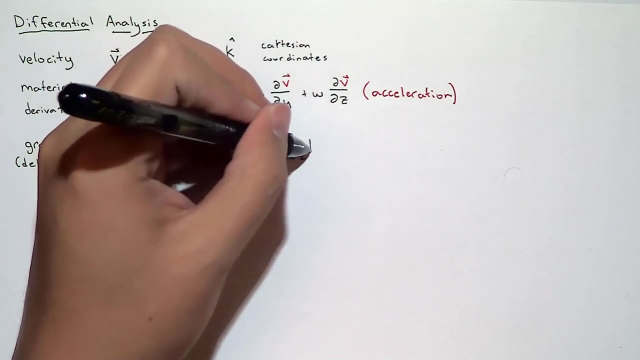 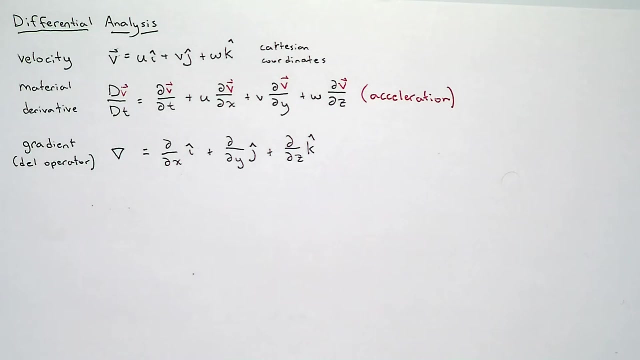 it's an operator, Not a property, was defined as simply a partial change with respect to x in the x direction, plus the partial change with respect to y in the y direction, plus the partial change with respect to z in the z direction And, like we mentioned earlier, this del operator can be applied to any 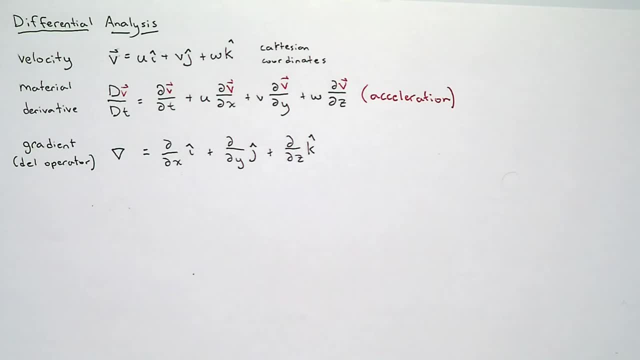 scalar field. Now, in Monday's class we did one example of a scalar field. So what we see here is we had a scalar field which was a pressure field. So if we applied the del operator to the pressure field, then we get the partial change of pressure with respect to x in the x direction, plus the partial change of pressure with respect to y in the y direction. 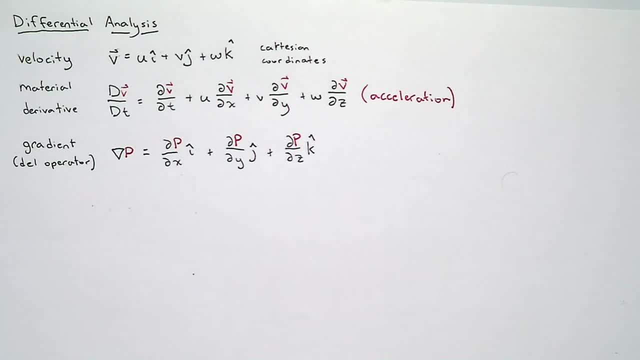 plus the partial change of pressure with respect to z in the z direction. So this particular example, not necessarily important that you memorize it, but just in case, when you apply the del operator to any function, you get the gradient of that function. 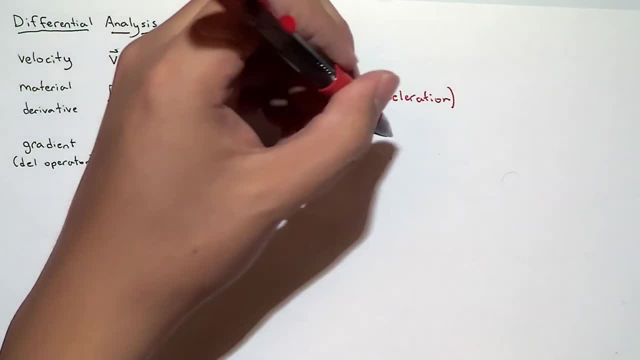 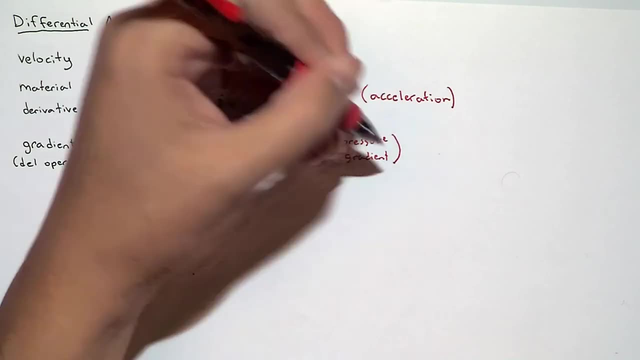 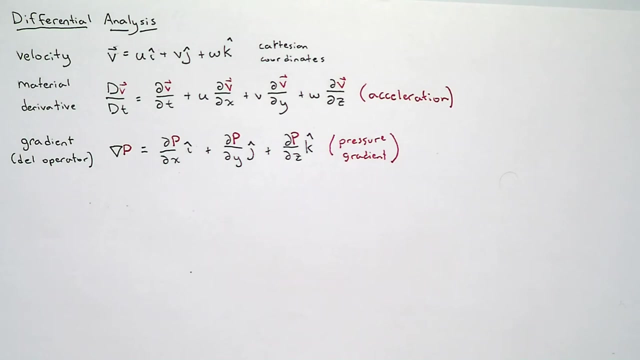 In this case, because we applied the del operator to the pressure field. then we get what's called the pressure gradient. So the only difference between the gradient and the material derivative is that gradient is space and material is space and time. Yes and no. 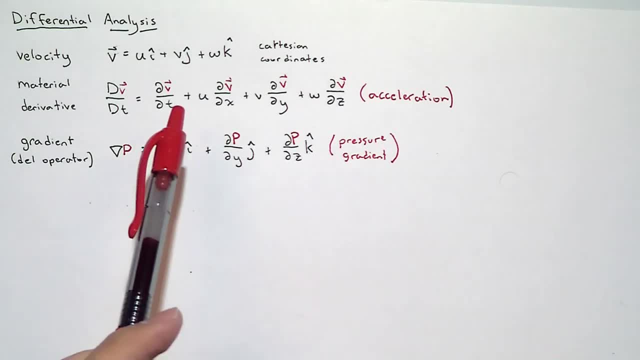 So, yes, that's one of the differences. The other difference: remember that in the spatial derivative, here in the material derivative, we're also considering the fluxes, right, Because we have velocity terms as well. We do not have velocity terms here. 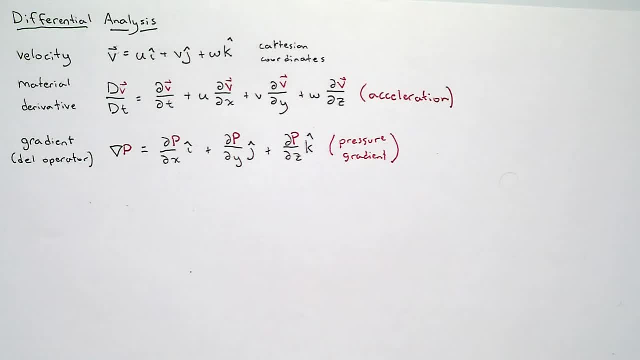 Now it's OK because you bring a good question and we're going to jump into it. We're going to see how we can relate the gradient operator to the material derivative in just a second. So good question, Drew. We mentioned that this del operator is a very, very powerful operator. 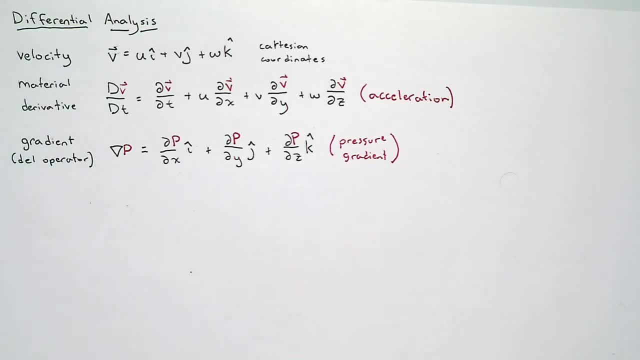 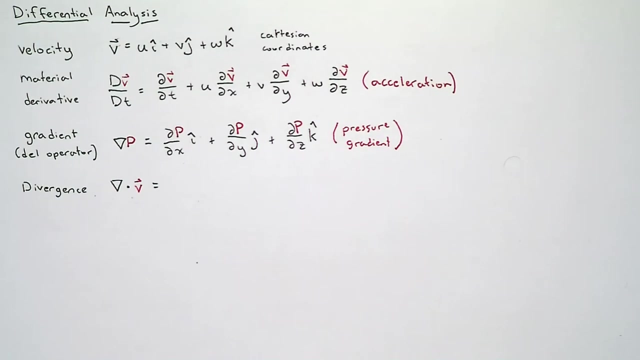 mathematical operator. For example, we can use this del operator to find the divergence of a vector field, And the divergence of a vector field was simply found by taking the dot product of del and some vector field. In most examples that we were going to look at and, frankly, 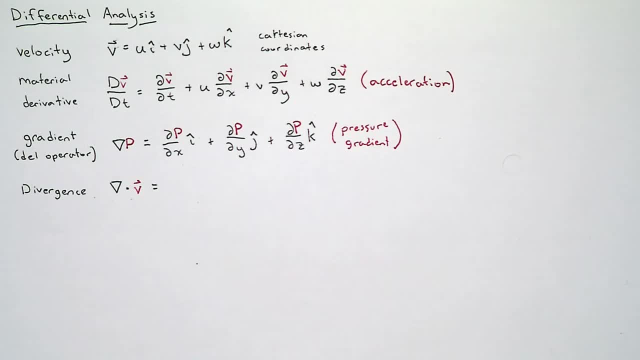 most examples that we're going to do in this class. we will be looking at the divergence of the velocity field. Now, what does that look like? Well, you know, the dot product of two vectors is simply the x component of one times the x component of the other. 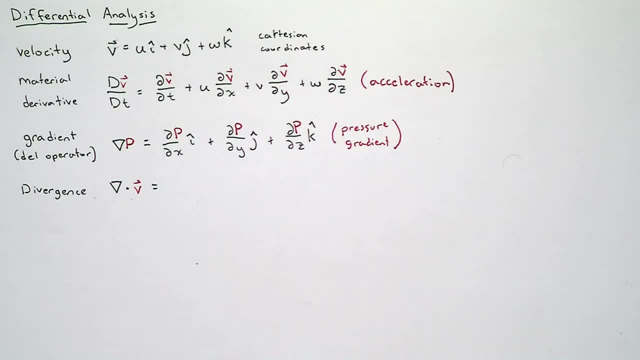 Plus the y component of one times the y component of the other, plus the z component of one times the z component of the other. And that's the same thing here When we take the dot product of the gradient operator, the del operator. 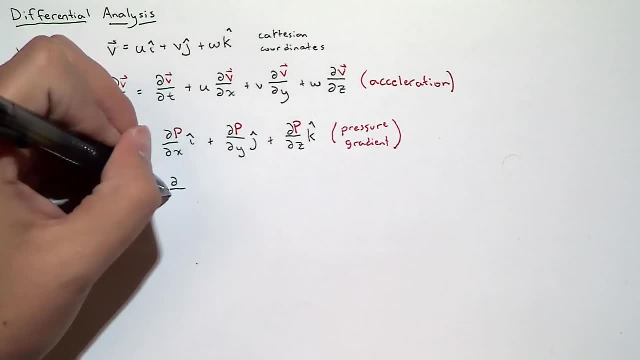 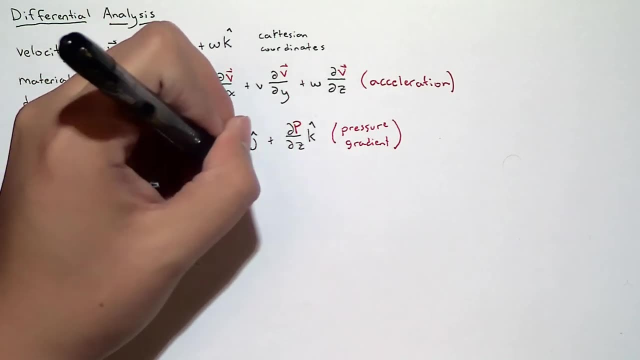 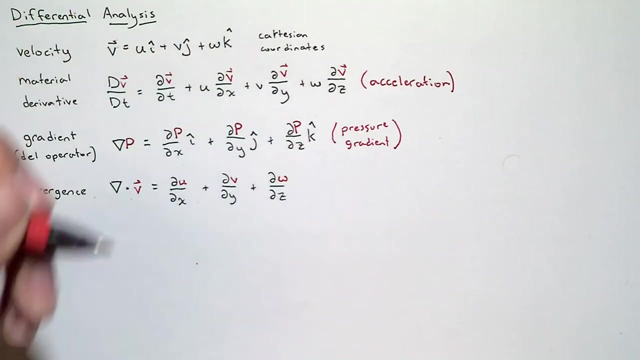 and any vector field. essentially we get the partial derivative of the x component of the vector field with respect to x, plus the partial derivative of the y component of the vector field with respect to y, plus the partial derivative of the z component of the vector field with respect to z. 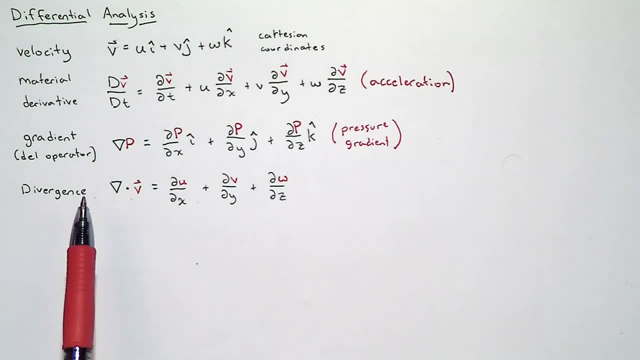 In this example, because we're taking the divergence of the velocity field. we express it in terms of the x-component, which we know is u, the y-component, which we call v, and the z-component, which we call w. So one of the key differences between these two is that the gradient operator is applied to a scalar, as you can see here, but the divergence is taken for a vector. 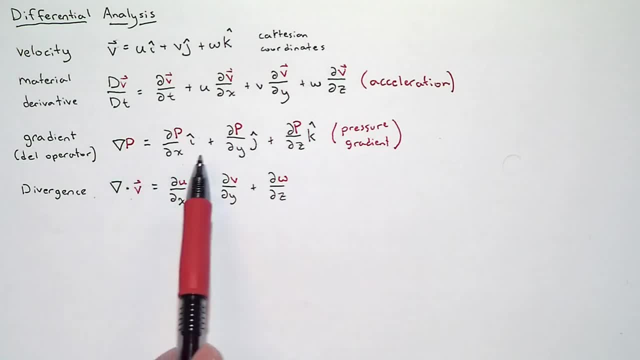 Now the result of the gradient is a vector, but the result of the divergence is a scalar. So you see how these terms are inverted here. You input a scalar, you output a vector. But when it comes to divergence, you input a vector but you output a scalar. 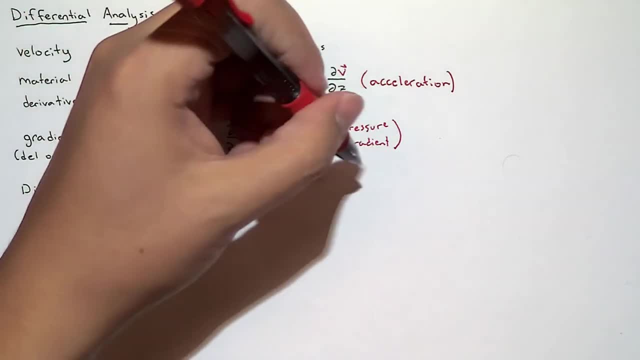 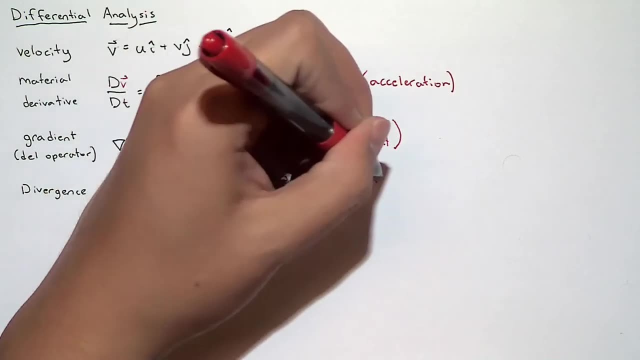 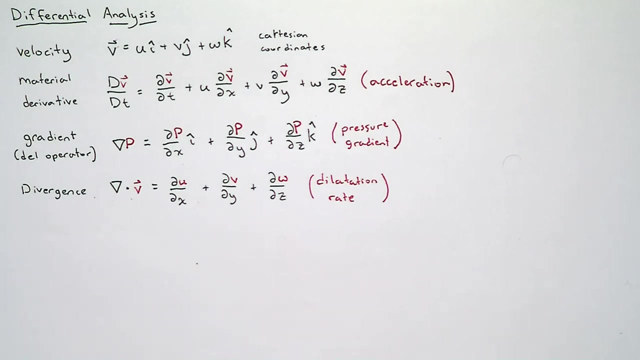 Now, in the case of velocity, the divergence of the velocity field is called the dilatation rate And we can see mathematically This dilatation rate essentially is telling us whether the fluid particle that we're studying is expanding or contracting. 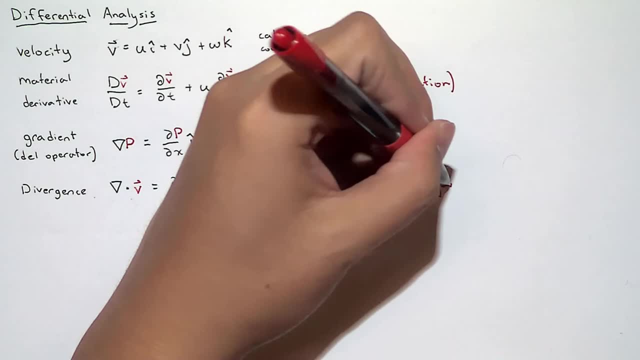 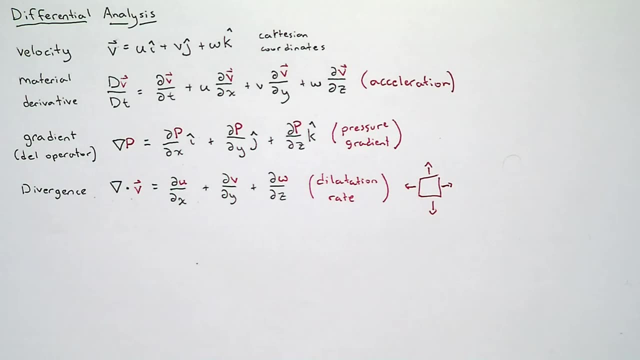 So dilatation rate will tell us about the deformation of a fluid particle. Now, based on that information, knowing that the dilatation rate gives us the deformation of a fluid particle, then I can say: if my fluid Is incompressible. 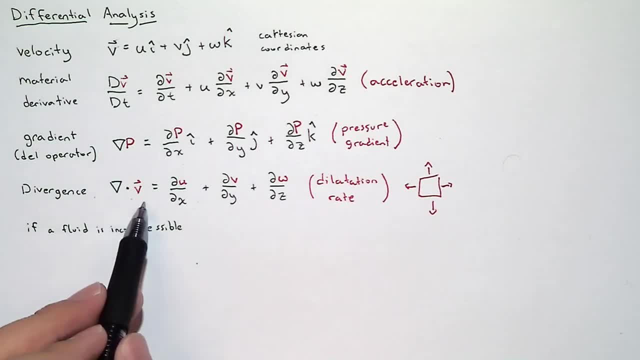 Right, If a fluid is incompressible and we know that the dilatation rate tells us the growth or the shrinkage of a fluid particle, then what do you think the dilatation rate of a fluid that's incompressible has to be? 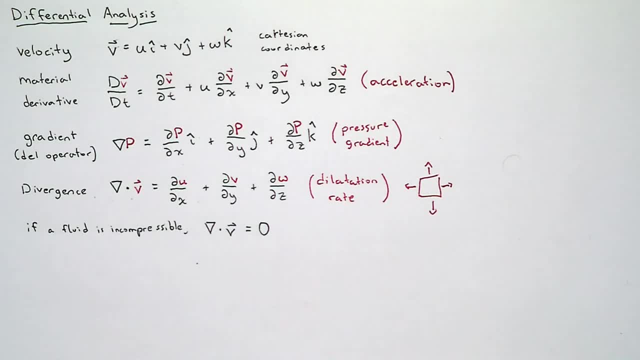 Zero right. Because if the dilatation rate is the growth right, the expansion or the contraction, and we know that an incompressible fluid does not expand nor contract, then that means the dilatation rate of an incompressible fluid will be zero. 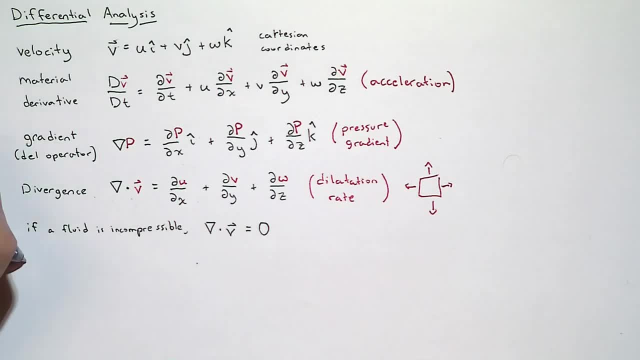 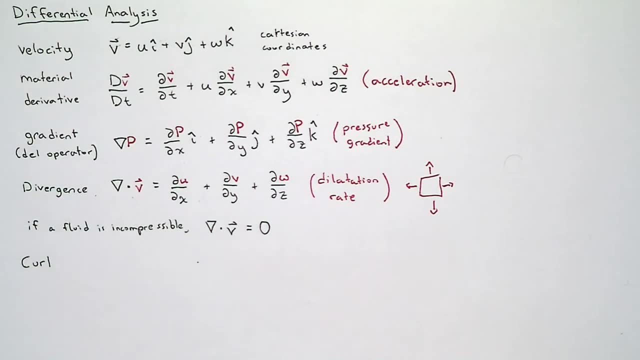 Finally, we looked at curl. We said that the del operator can also be used to find the curl of a vector field. We know that curl can be found by taking the cross product of the del operator and any vector field. Now, if you don't remember how to find the cross product of a del operator, 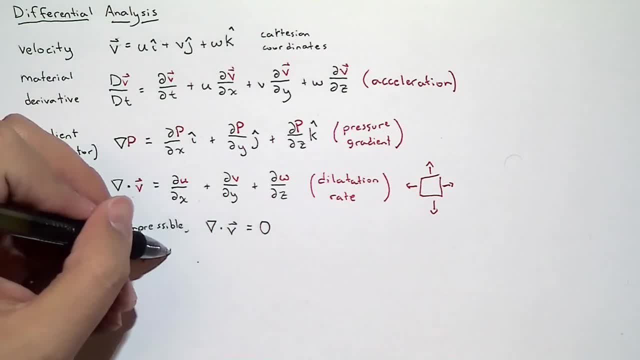 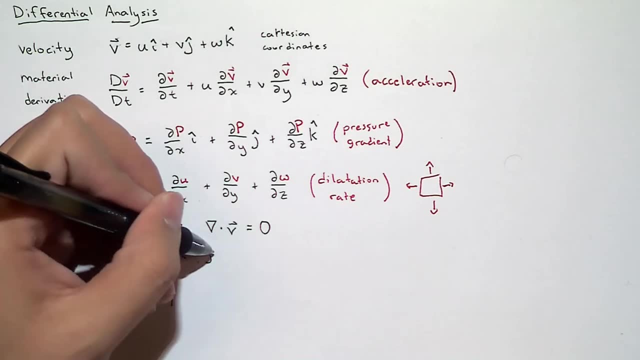 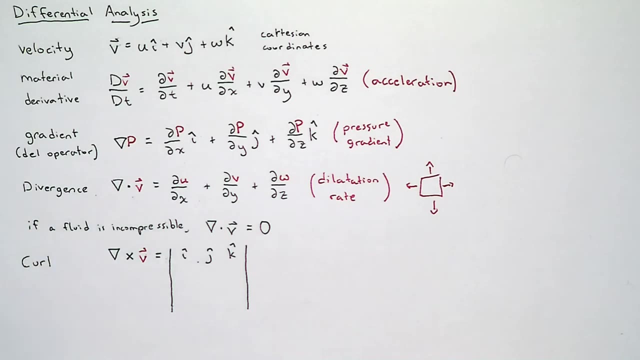 and a vector field, then you can draw the matrix, the resultant matrix of these two vector fields, and then find the determinant of that matrix. Now, of course, we don't have time to review how to find determinants. However, I would always say that it's helpful if we at least have them here. 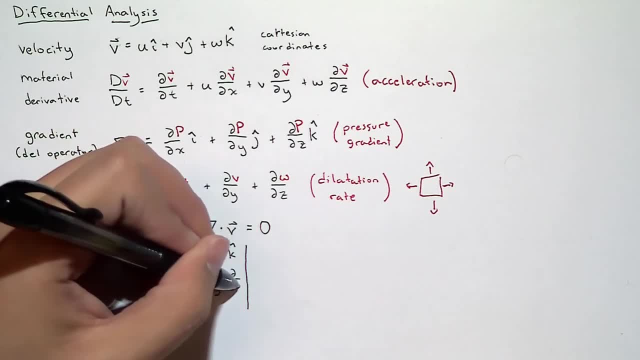 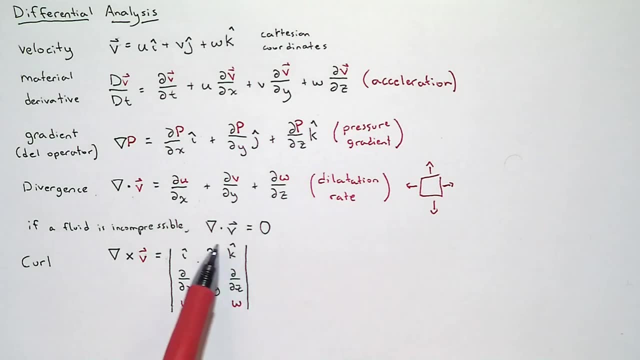 so that we can at least visualize what this curl looks like And remember that- And I'm trying to distinguish the parts of the equation that belong to the operator, which are in black, and the parts of the equation that belong to the vector in question- 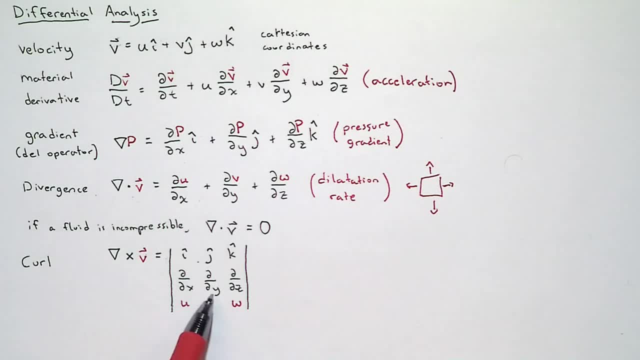 which are in red. These red parts can be applied to any other vector, which means that this doesn't have to be velocity. If it's in red, it can be any other vector field. However, in the material derivative, because this is a black part- 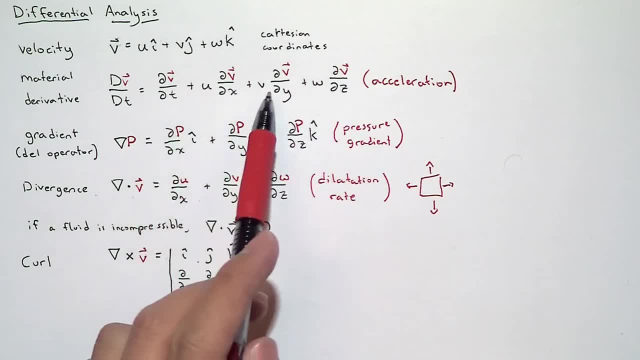 this actually has to be velocity u, b and w, right, these three black terms. So let's try to make that distinction. The black, The black ink represents the operator right, the stuff that cannot change, But then the red ink will represent the vector or the scalar. 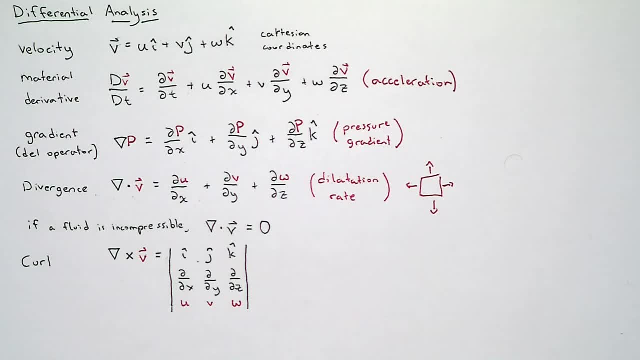 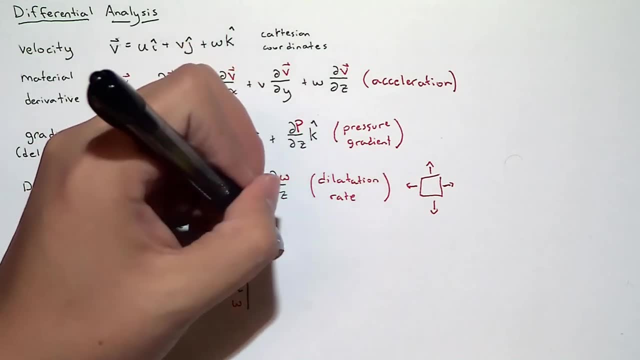 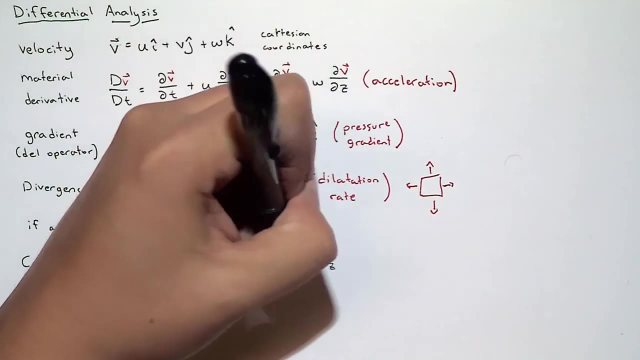 to which I'm applying my operator, which can change if necessary. So if we were to find the curl of a vector field, remember that we're going to have the following expression, And I know that you know how to find this: 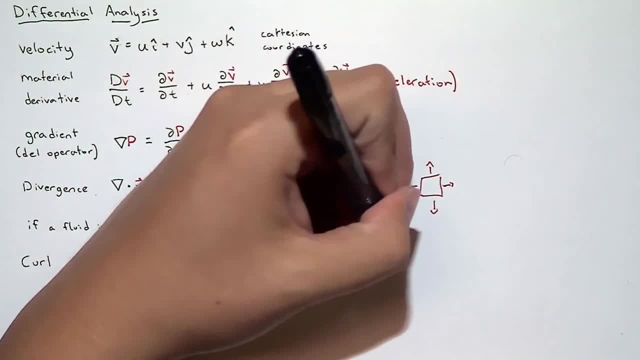 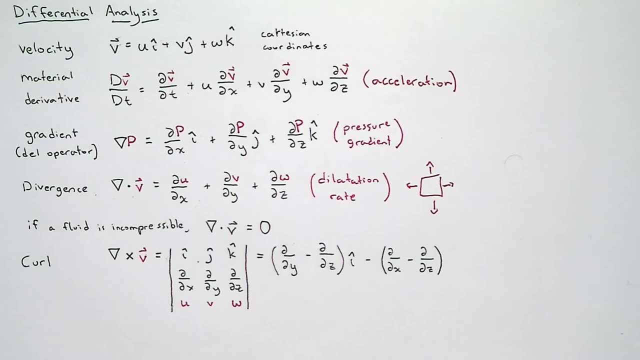 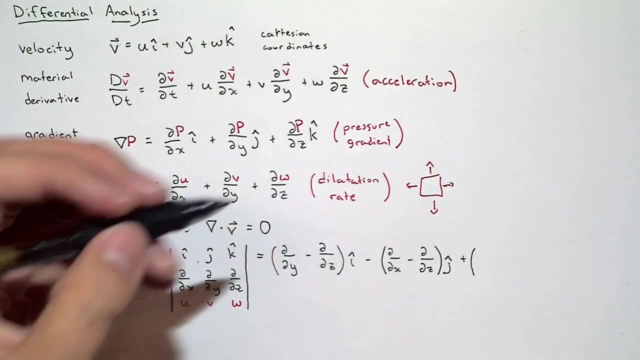 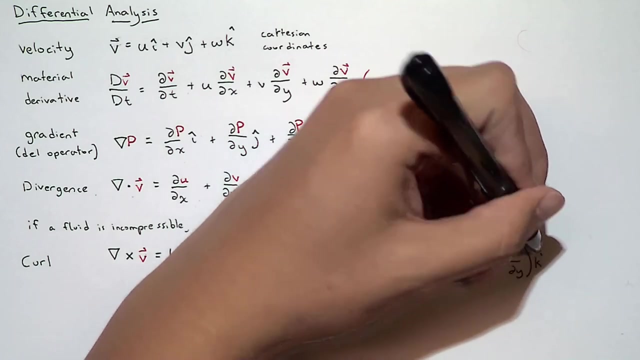 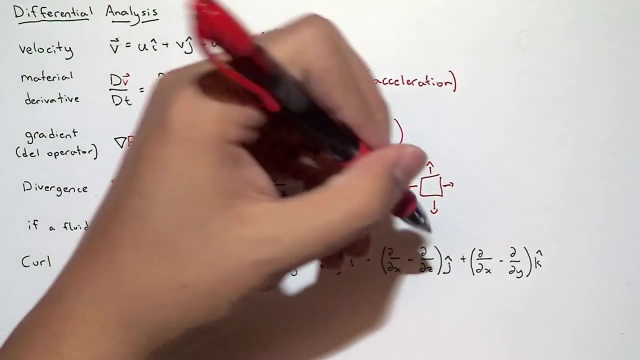 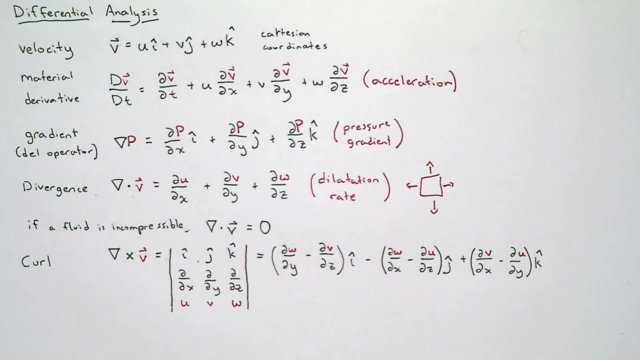 so we won't go into too much detail about it, But I do want to write it down so that we can at least have it here and use it as a reference when we solve some example problems. So this is the curl of a vector field. 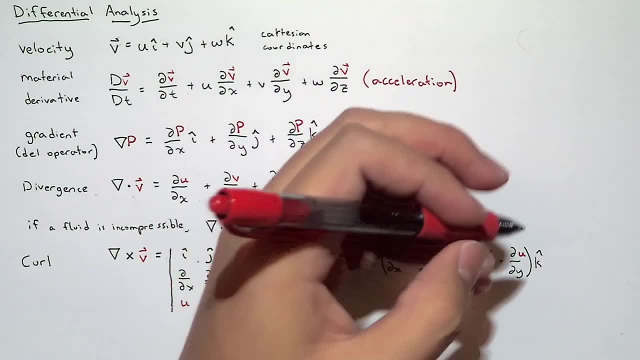 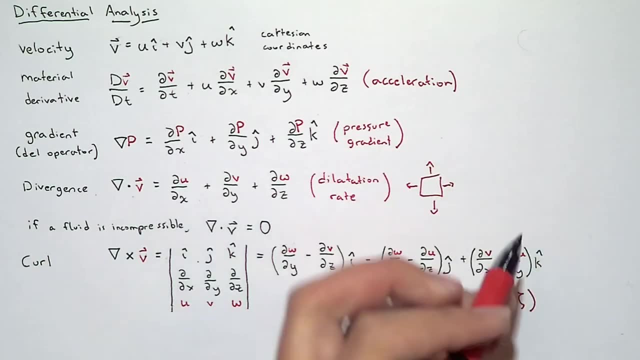 Now, if you find the curl of the velocity field, we call this the vorticity. Sometimes you use the Greek letter. which one is it? zeta, right, The Greek letter zeta- to calculate or to express the vorticity. 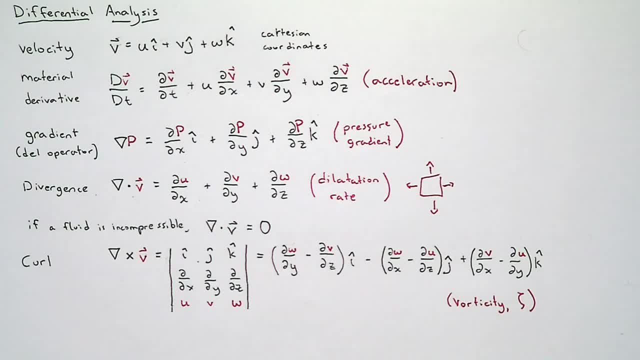 Now there's a couple of clues just on this math and on the names themselves that may give you an idea of what curl represents. First off, we're looking at a cross product, And we know that a cross product right looks at differences. 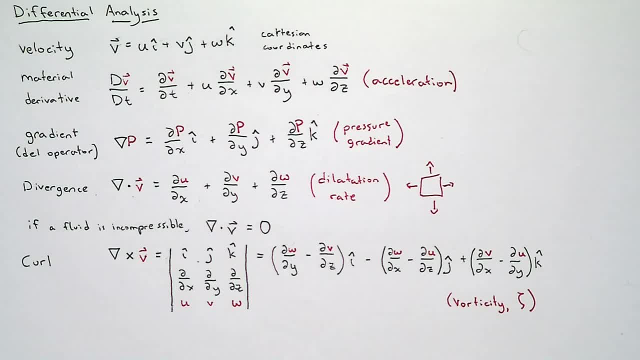 in direction and potentials for rotation. So, based on that idea, if we're looking at a cross product of a derivative and a vector field, we're essentially looking at the rotation of that vector field. Now, what that means is that the curl 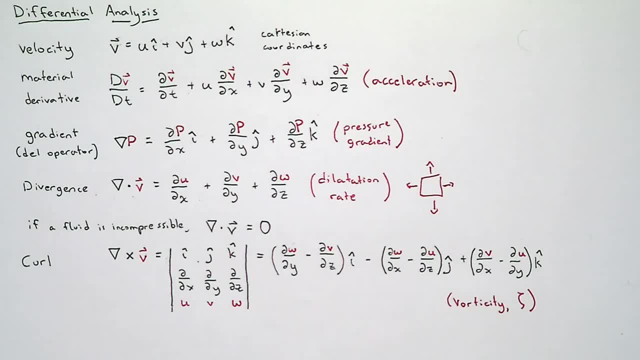 of the velocity field gives us the rotation of a fluid particle, And that rotation is what we call vorticity. So it's just trying to measure how much that you know is going to be. So it's just trying to measure how much that you know. 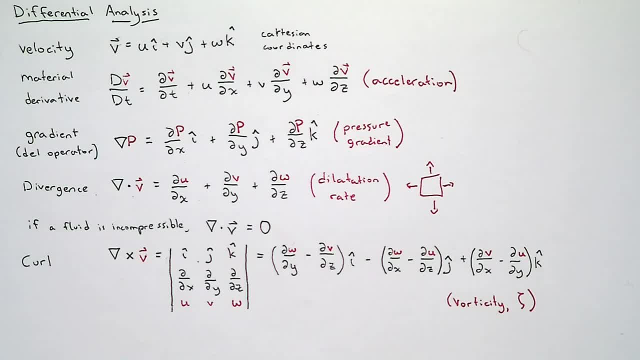 is going to be So. it's just trying to measure how much that you know is going to be So. it's just trying to measure how much that you know vector is changing, turning How much it's rotating. yes, 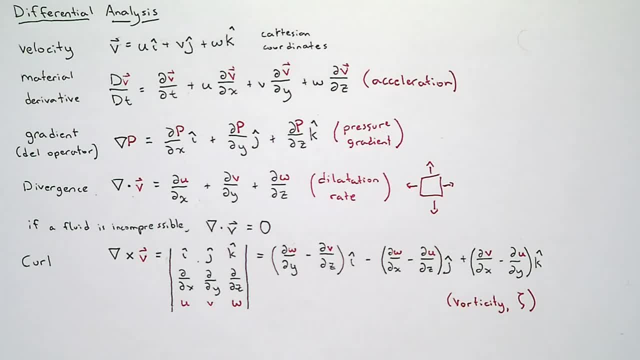 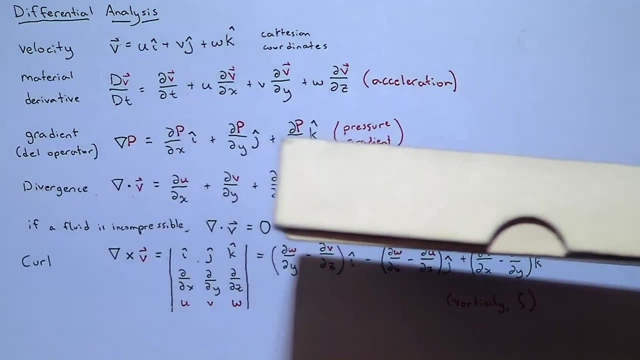 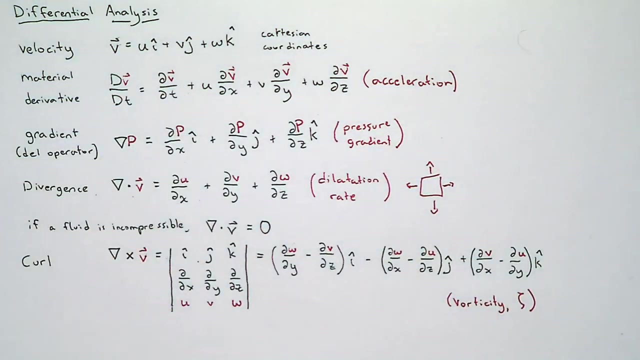 Like changing direction, Not necessarily changing the direction of flow. Think of it exactly. Think of, yeah, think of this as my vector field. right, My vector could move in one direction, but it could also rotate along that axis. So this rotation is what we call the vorticity. 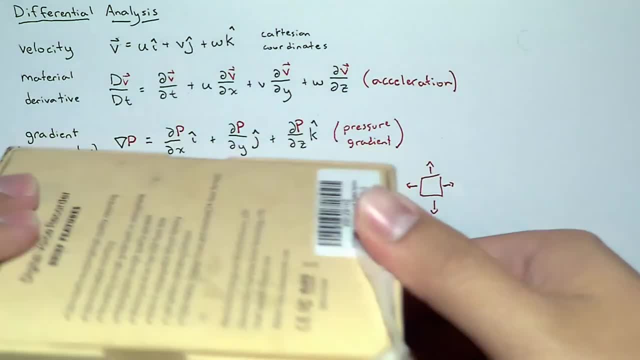 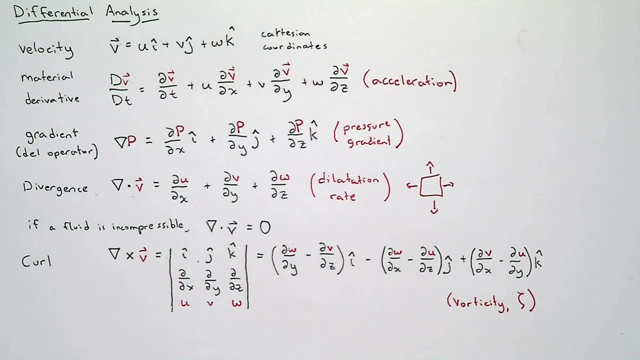 So notice that even though my vector doesn't change the direction of movement, it still rotates right. So that's what I mean when I say vorticity. It's that rotation among an axis that doesn't necessarily relate to its displacement. 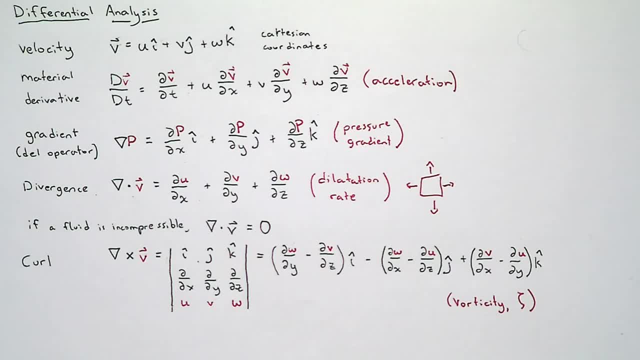 Okay And good question. Thank you, Casey. Spin, That's a good idea. Yeah, that's a better way of putting it. spin. Yeah, that's good, Based on what we know, if a fluid is a vector. 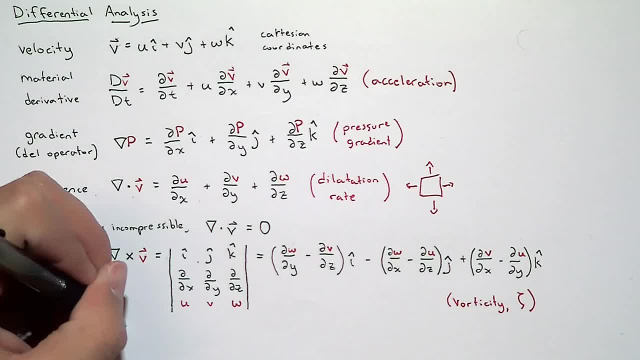 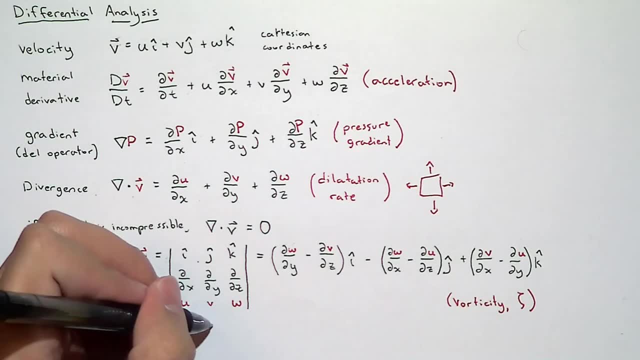 it's going to rotate along that axis, It's irrotational. In other words, if a fluid particle has no spin, what do you think is the vorticity of that fluid particle? Zero, Zero. If there's no spin, there's no vorticity. 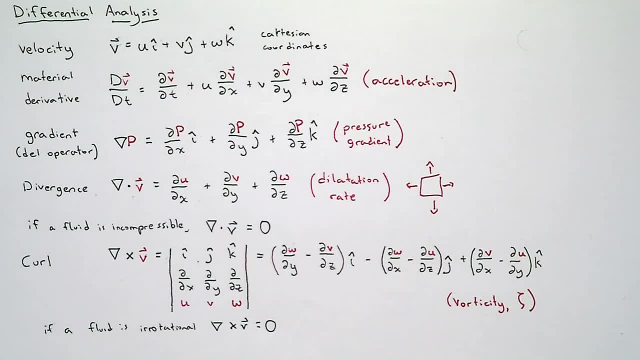 We will learn that when we derive expressions for angular velocity in differential form, we'll find that angular velocity is actually very, very related to the curl. In fact, angular velocity, once we derive an expression, it's going to be very, very related to the curl. 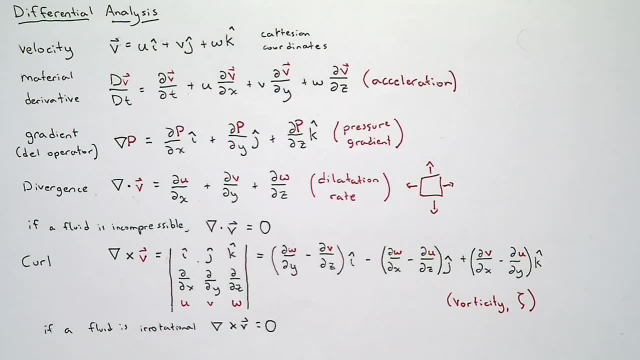 So we'll find that angular velocity is actually very, very related to the curl. That constant crítons and theness is our expression for it will be just one half of the curl. That further solidifies our explanation of the curl. 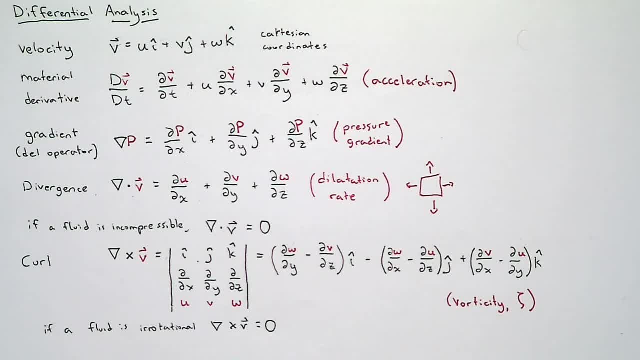 as the rotation or spin of a fluid particle. So this is a bit of a review of what we covered on Monday, Now before we start with newer materials. are there any questions with this material? All right, So if there are no questions, make sure you take your notes. We're going to refer back to these definitions in a second, But let's go ahead and start with the semantics over here. We're going to start with somes. So this analysis we've heard about is based on northeastidamente And some of these judgments that these equations produce. 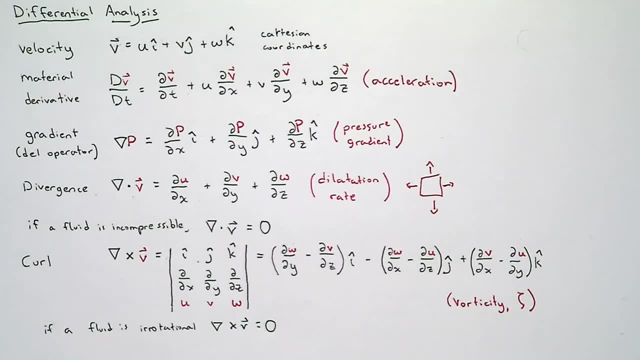 we talk about present Olympics. you know the license. But we also heard about other student thermometers, examination any kind, and above that with an example of divergence. so in Monday's class we looked at a curl example. so now I would like to look at a divergence example. 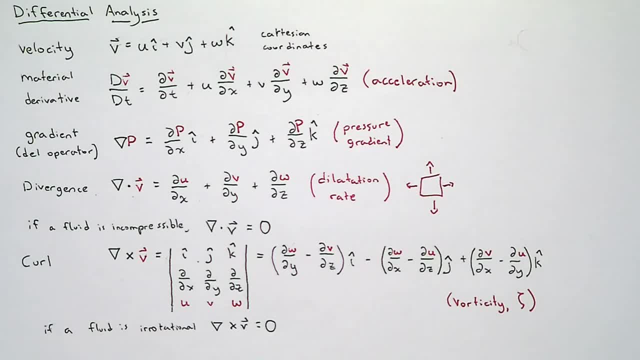 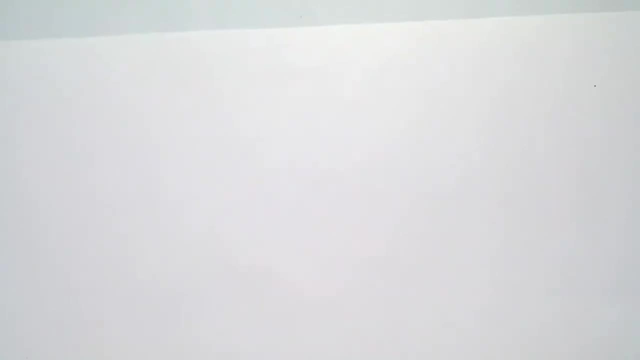 all right, this is example 5.5 from David Chin's book. it's not your textbook, so make sure you take notes if you don't have Chin's book with you, which is not really a good book, but it's a good book. so I would like to look at a divergence. 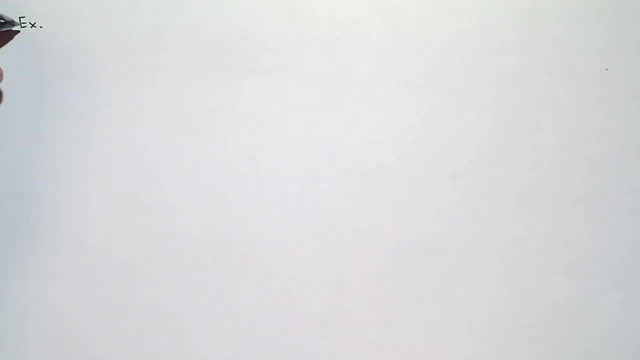 example. so in this example we are given a velocity field that's defined by the following terms: we have 6xyzi plus 2 times x squared plus y squared j plus 3y zk. now I mentioned Monday. I'm going to try to refrain from using units. 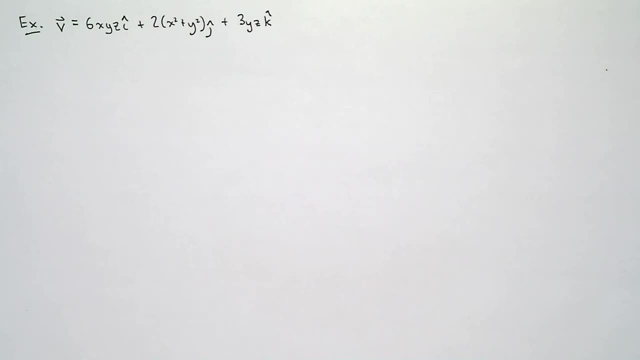 for this week, not because they're not there or not because they're not important, but I just don't want you confused with so many variables, because we're going to be dealing with a lot of variables, so let's just assume that this is. this has its own units of length over time, whatever that is, and we're going to. 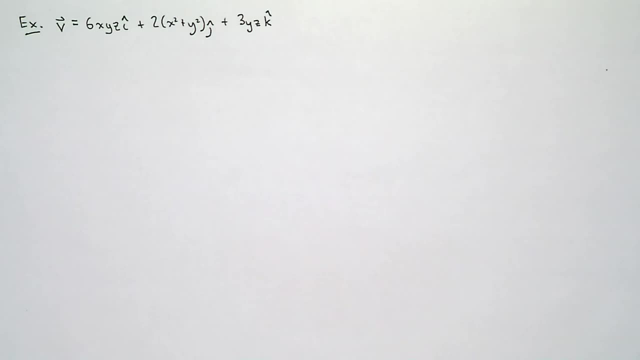 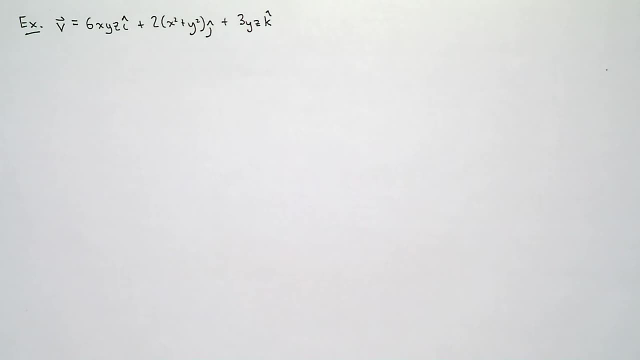 component of the velocity field? just a y component. what would that Y component be good? so remember that the velocity vector consists of an X component, Y, x, y and z directions respectively. So you can use those as your clues to tell you which one's the x component. 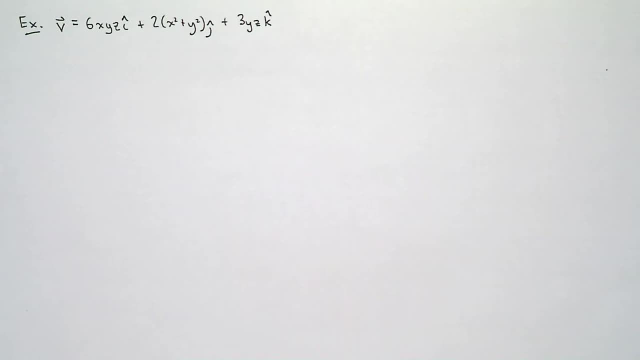 which one's the y component, which one's the z component. So now my question will be: for this velocity field, I would like to know what is the dilatation rate, In other words, what's the divergence of the velocity field? 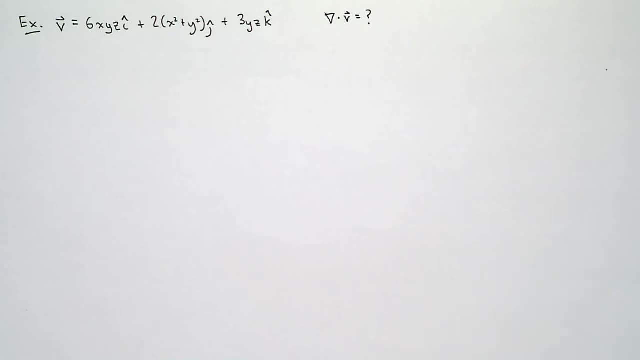 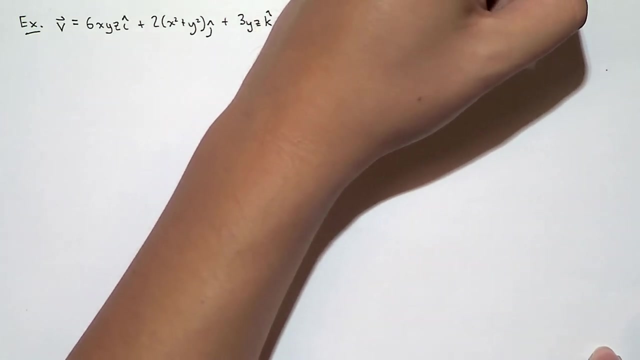 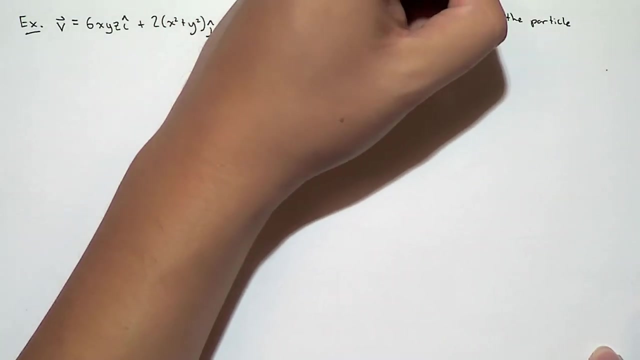 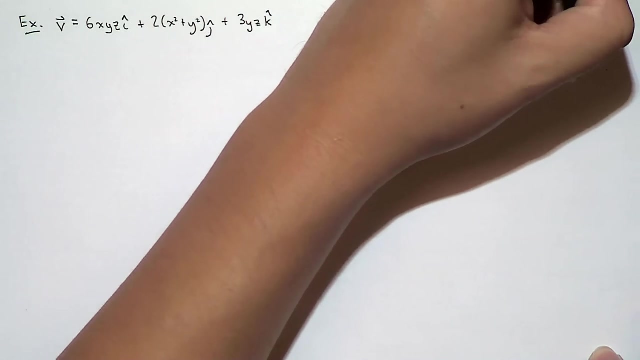 And I would also like to know at coordinates 1,, 1,, 3, so at 1,, 1, 3, those are Cartesian coordinates- is this fluid particle expanding or contracting, Or neither? Okay, so those are my two questions. 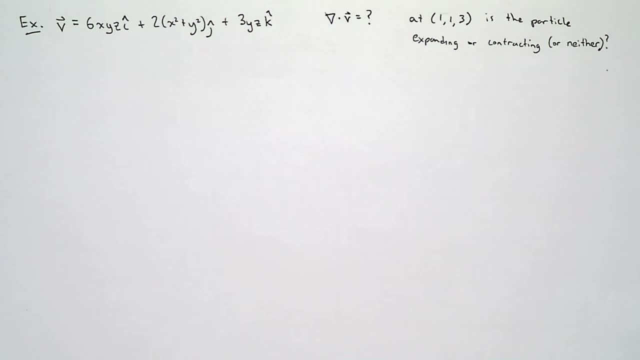 How do you think we can start? Well, we're asked to find the dilatation rate, that's the divergence of the velocity field. So how can we find the divergence of the velocity field Exactly? Take the dot product of the del operator and the velocity vector. 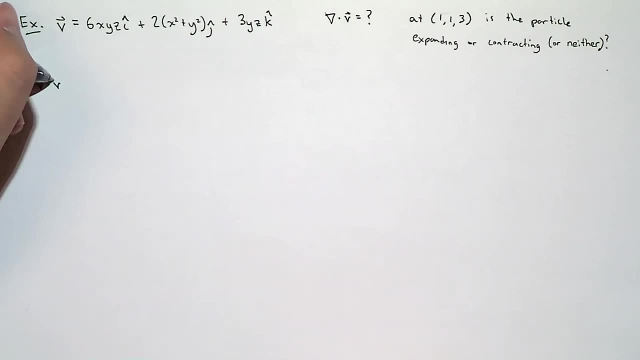 So the divergence of the velocity field should be equal to the partial change of the x component of velocity with respect to x, plus the partial change of the y component of velocity with respect to y, plus the partial change of the z component of velocity with respect to z. 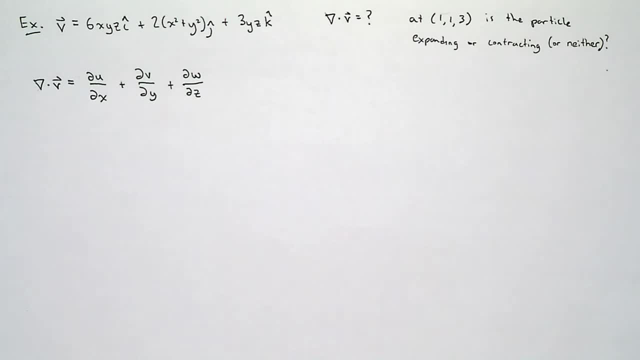 So let's go ahead and try to find this dilatation rate or this divergence of my velocity field. In this case, we want the partial change of x with respect to x, So we only care about the x component, that's the u. 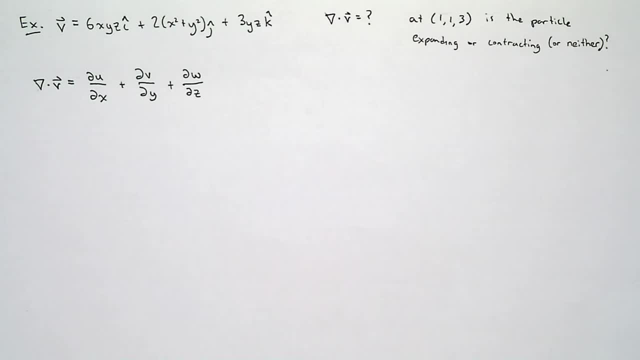 the x component of velocity. So, Dallas, what's the partial change of my x component with respect to x? That's correct. So we get 6yz. Likewise, we need the partial change of the y component with respect to y, JJ. 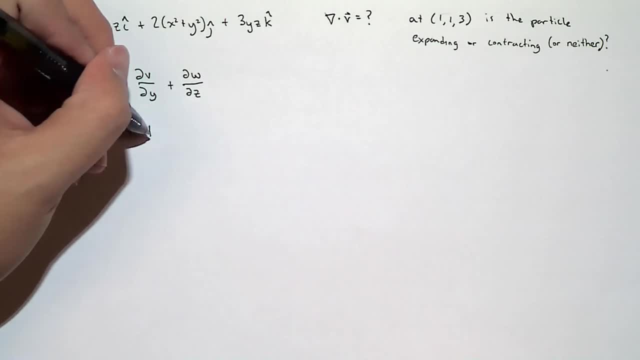 4y, Thank you, And we need the partial change of the z component with respect to z Mayur, Mayur 3y Yep, And we found the dilatation rate. Is it that easy? Yes, it is that easy. 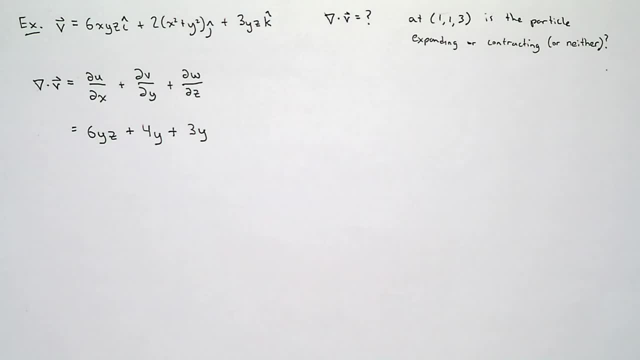 As long as you know how to find the derivative of the correct components, we should be fine. Of course, if you want to perhaps organize this a little bit, I can write something like y times 6z plus 7. Perhaps I could do that, and that's good. 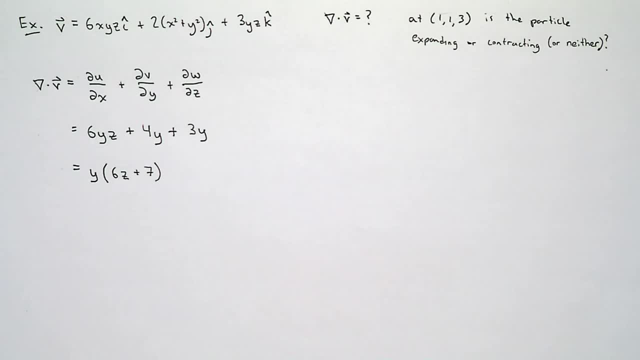 Now here's my question. And notice that for this question, just looking at this answer, when you take a dot product, the i, j and k vectors go away, because i dot i is just 1.. Now notice that we don't really need to do any calculations. 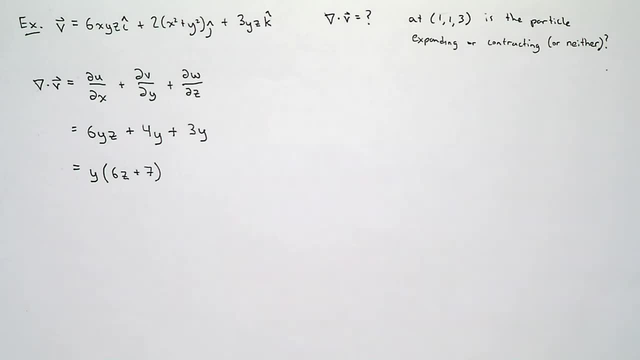 The question is: at 0.113, is the particle expanding or contracting? and why, If you look at just this expression, without having to calculate anything, is this particle expanding or contracting? Exactly, it's expanding because it's a positive value, positive dilatation. 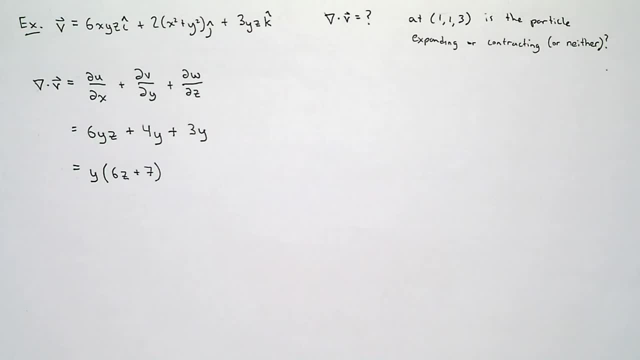 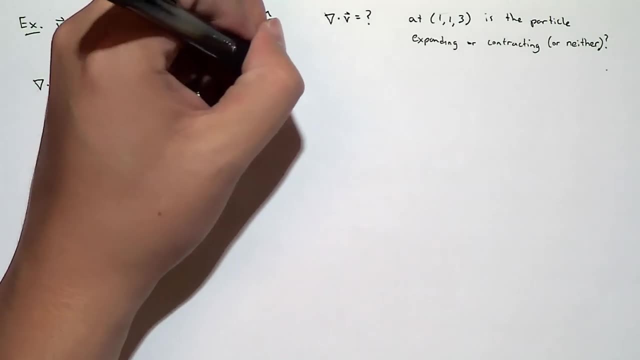 That means it's expanding. Of course, if that was not satisfactory enough, we could always find the divergence of the vector field, the dilatation rate, at 1.113.. And in that case, all we have to do is replace these variables. 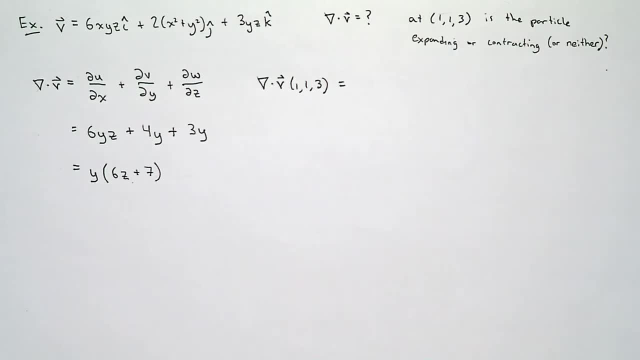 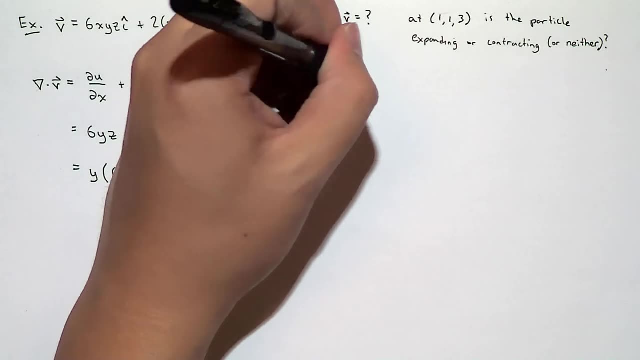 with my Cartesian coordinates. Of course there's no x-coordinate here, which means that my dilatation doesn't change in x-coordinate. But we do know that y equals 1 and z equals 3.. So this is just 1 times 6 times 3 plus 7.. 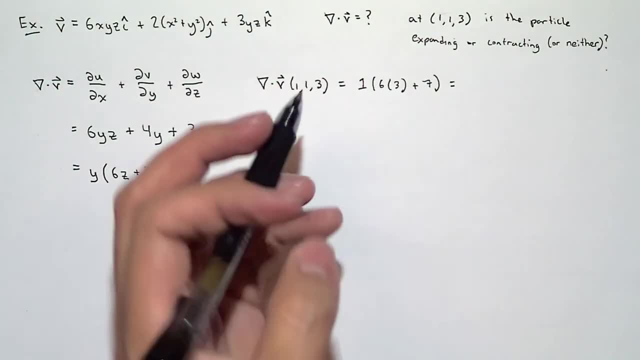 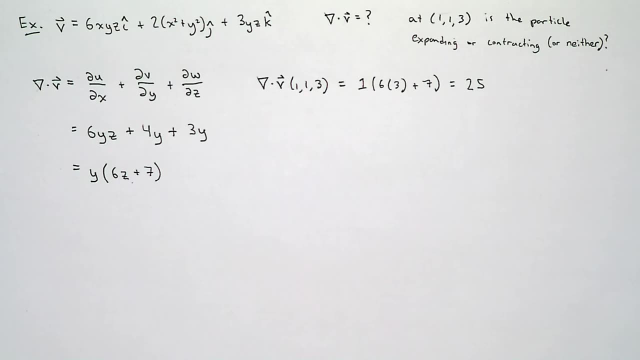 And of course we know that this will be a positive number. How much is 18 plus 7? 25?? OK, So we have concluded that at 1.113, this particle is expanding. In fact, notice that as long as this particle is. 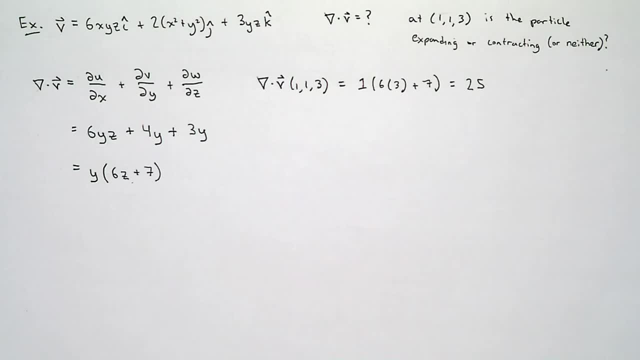 on the positive side of y and the positive side of z, it will be expanding. If the particle is on the negative side of y and the positive side of z, it will be contracting, And then there's some nuance with the remaining spaces. 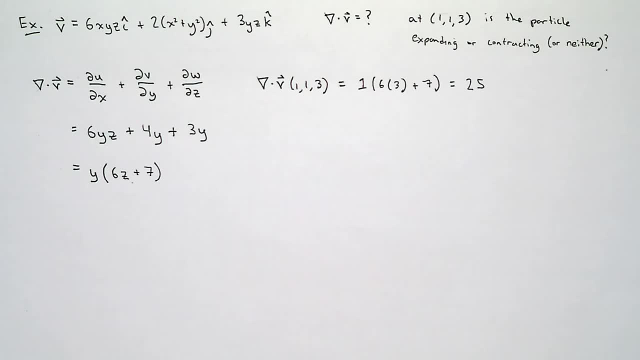 So that's the dilatation rate And that's how we know whether a particle is expanding or contracting, based on the answer or the domain of that dilatation rate. At this point, are there any questions? No, OK, So we're going to go ahead and start the del-and-del. 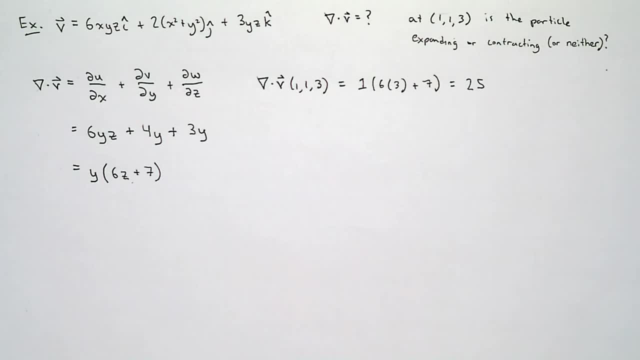 operator. We're going to continue our invention with this del-and-del operator, And then we're going to do any other things. So first I'm going to go ahead and put up my name. So what I'm actually going to do is I'm going to start this del-and-del. 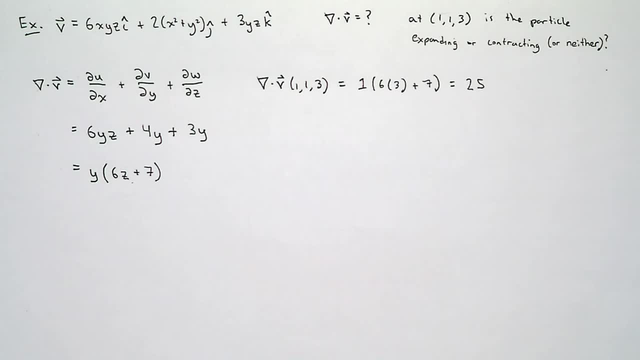 operator right here, And then I'm going to get out the name of the vector and I'm going to use this del operator in order to end the del-and-del vector. So back here I'm going to put up my name, this distance. 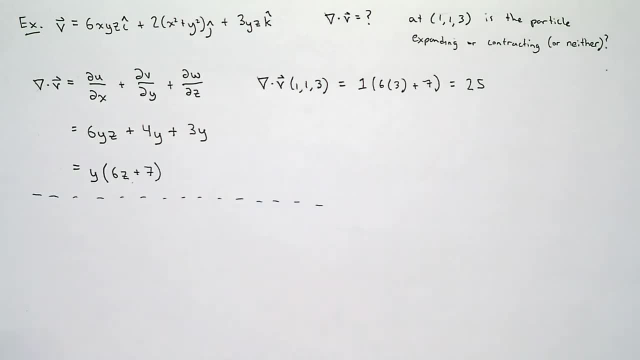 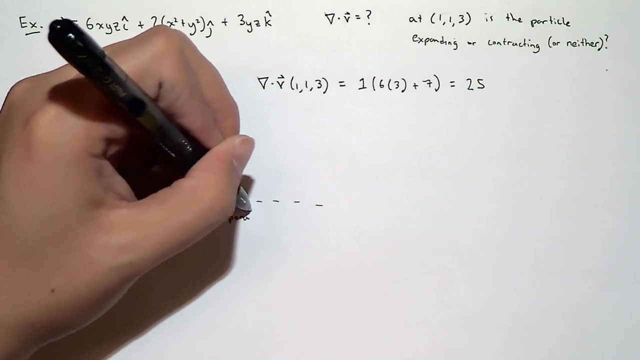 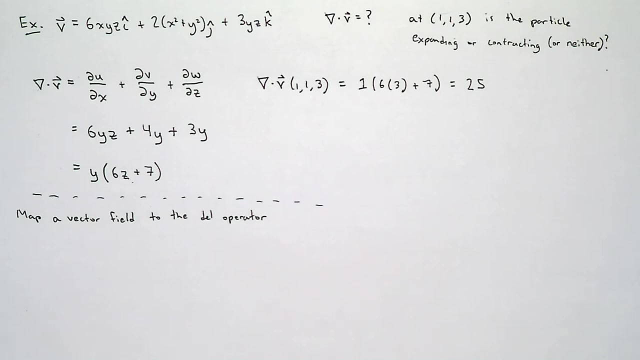 I'm going to put it in here, OK- of the del operator. one thing we can do with the del operator is we can map a vector field to the del operator, and we'll see what that means now, before we start showing the math behind mapping vector. 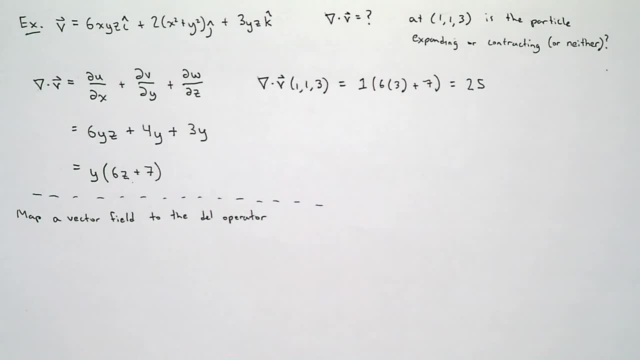 fields to the del operator. i do want to give a bit of a review about the dot product. when we're dealing with vectors and when those vectors simply represent physical properties, we know that the dot product is commutative right. so a dot b equals b dot a. is that correct right? 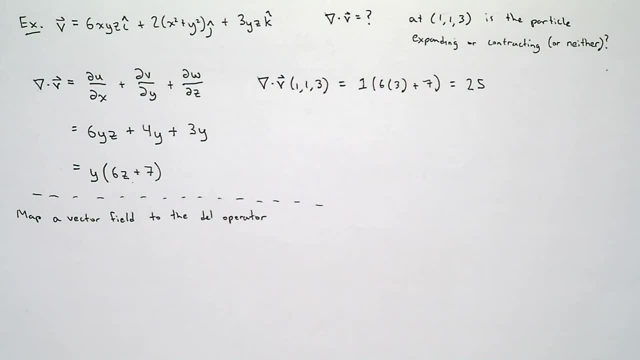 because a x, b x is the same as just saying b x, a x. however, when our vectors are not physical properties, when they are operators, just like the del operator, then we cannot say that they're commutative, because the order in which you take this operation will actually change your final 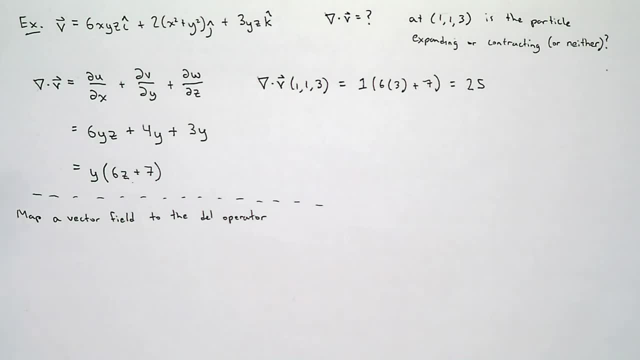 answer. so we know that if we take the divergence of the velocity field del dot b, we will end up with a scalar, because we have an operator, partial over partial- x applied to a vector field, in this case the x component of that vector field and the y and the z components respectively. 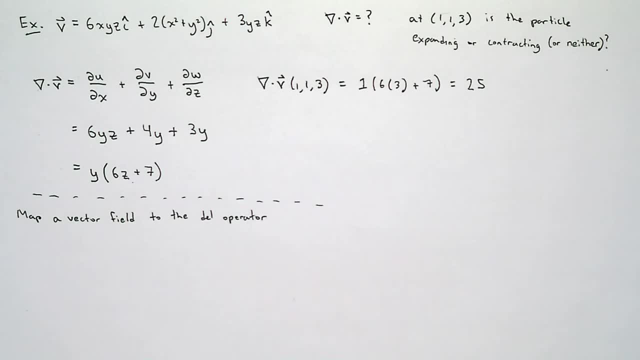 so when we map a vector field to the del operator, essentially we're taking the dot product but inverting the terms. so for example, in this case- let's suppose that we want to map a vector field f to the del operator- if i want to map the vector field f to the del operator, i would get f dot del. 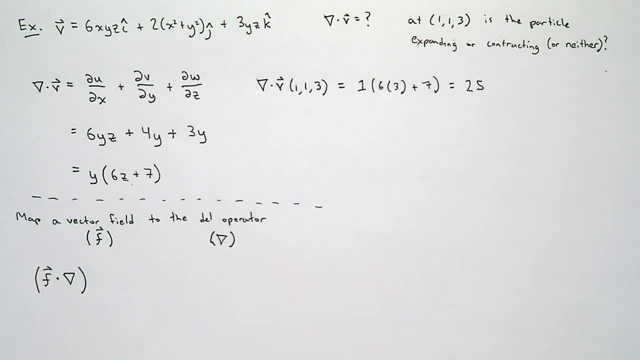 now i said that even though the dot product is commutative for physical properties, when we're dealing with operators it's not commutative, which means that the order in which you take your mathematical operations is actually going to change your final answer. so that's the problem. let's look at thequal trigonometric order. 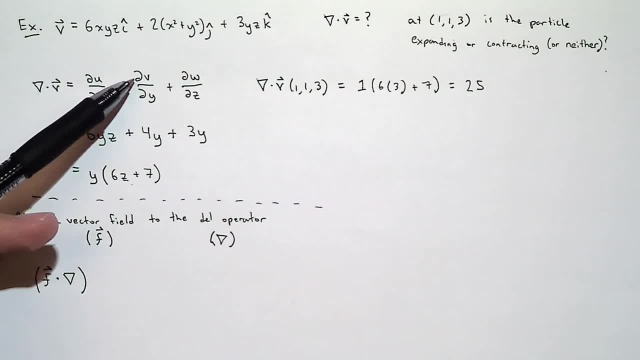 so make sure that we have the nosso. and you just fell me off j um. and you- let me start with the Alcoholics- and you have a particular expects. so earth to the world series over fiber, plus cy, plus fx, over fz, over yz, but because they're inverted, what do you think intuitively, what do you think we're going to get? 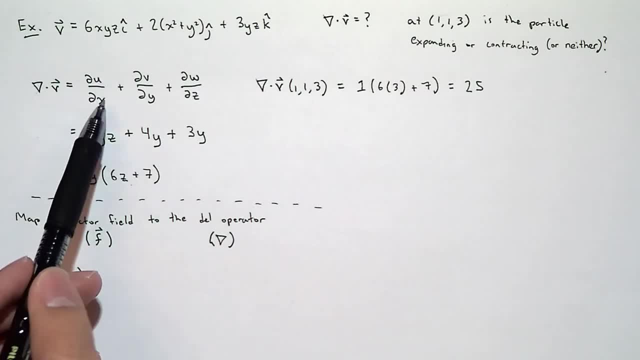 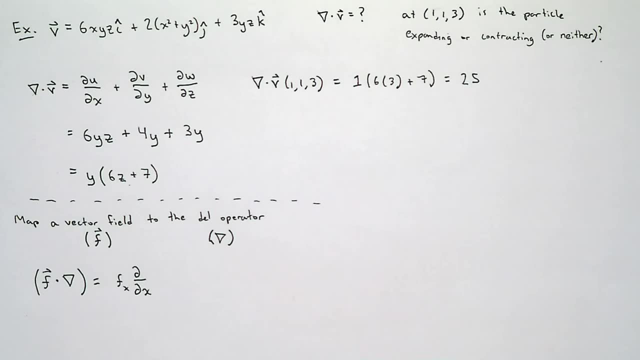 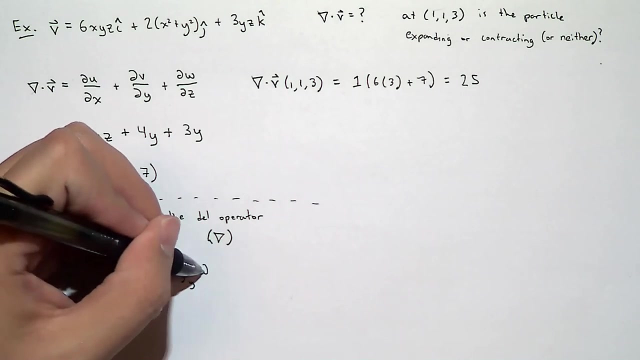 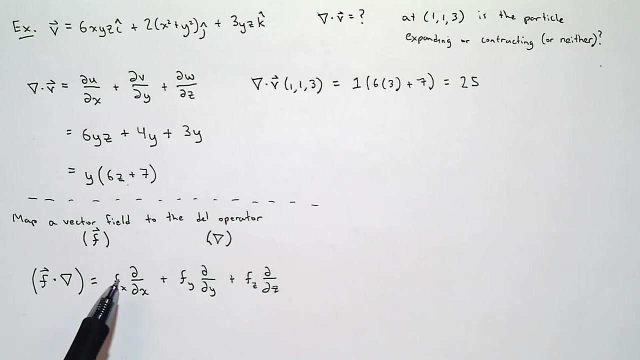 delf, we would get dou fx over dou x. but if we're taking fdel, we get fx dou x And of course we can keep mapping the remaining terms- fy, dou, dou, y, fz, dou, dou z- and we end up with essentially a scalar operator. right, It's an operator. 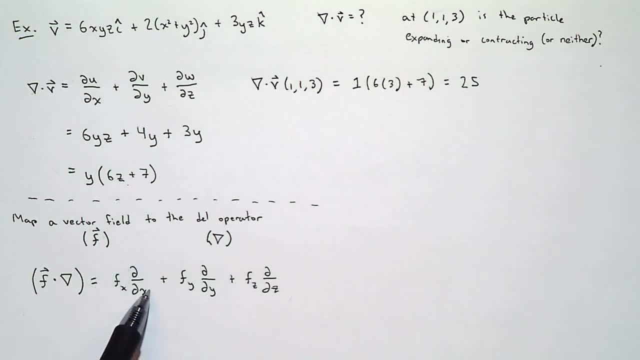 because, remember, this operator has to be applied to something. Operators do not exist on their own right. You don't have an equation that just ends with d over dt. The d over dt has to be applied to something. You're taking the derivative of something, right? 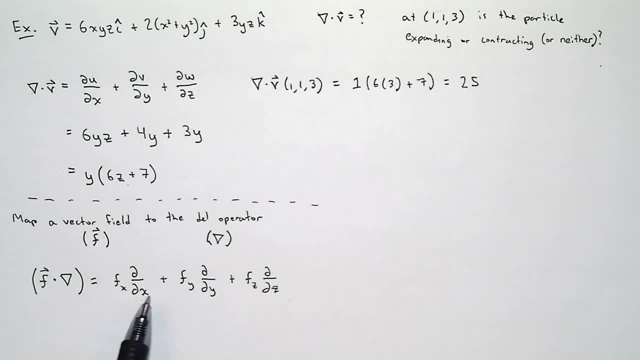 So essentially, this creates a derivative of something. So essentially, this creates a derivative of something. So essentially, this creates a new operator that also maps the x, y and z components of another vector field, and we'll look at an example. once we map a vector field to the operator, we can 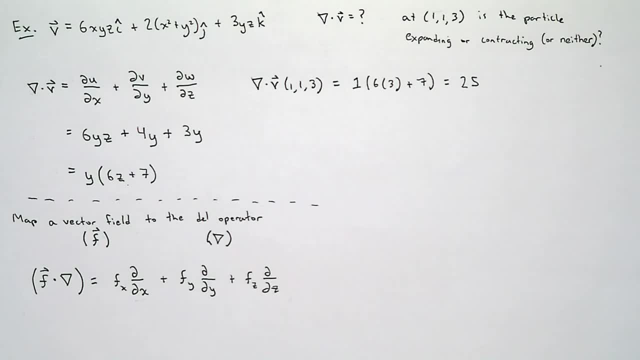 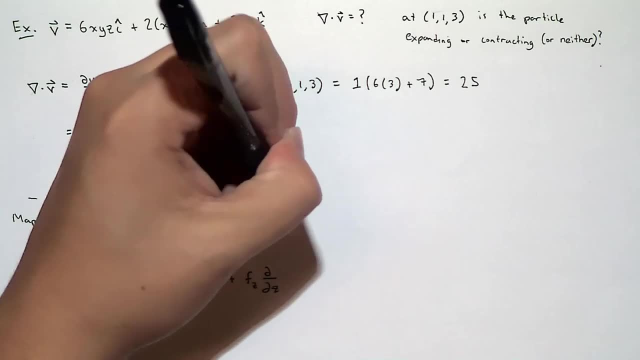 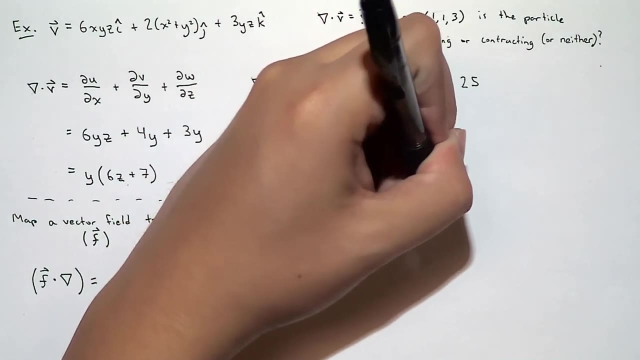 apply it to anything. we can apply it to a scalar, we can apply it to a vector. so after you map your vector field to the del operator, let's say we want to apply it to another vector field and I'm going to call this other vector field. 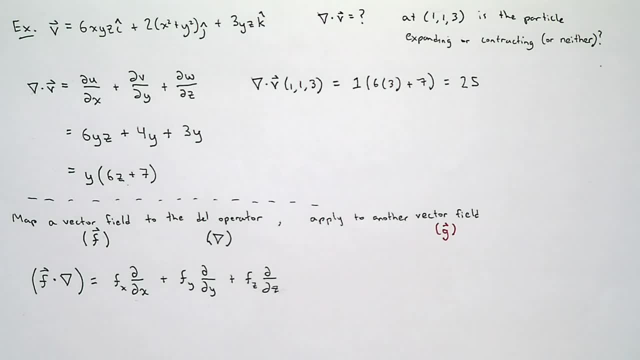 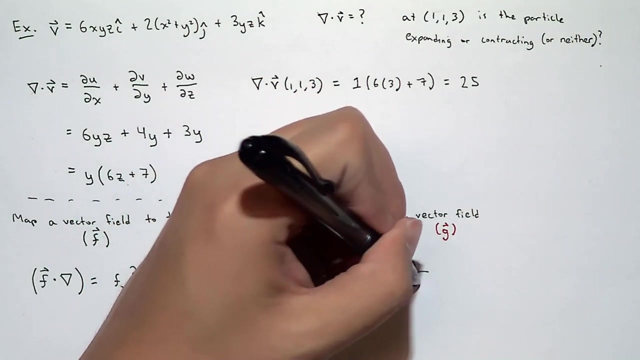 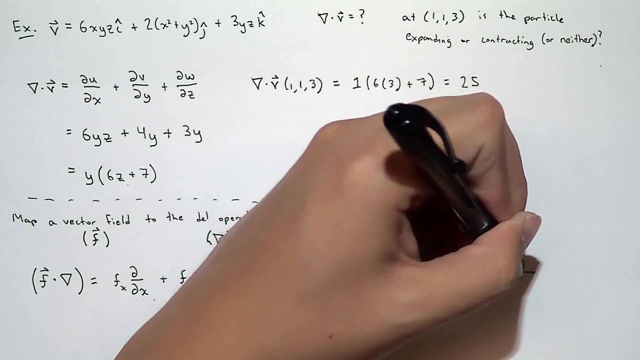 just G. in other words, I want to map f, del and then I want to apply this operation to my vector field G. essentially all that does is it applies this operation to the vector field G, operation to the entire vector field. So this would give us fx, fy, fz, and applied to my vector field g. 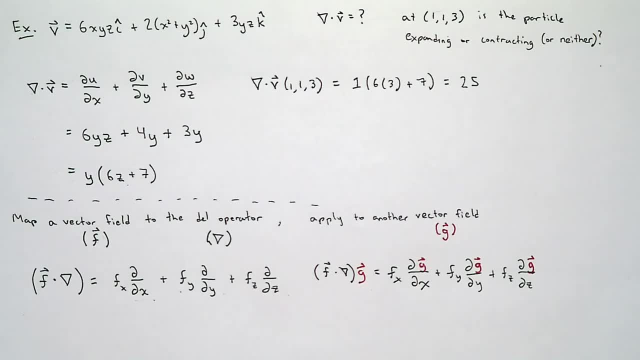 So that is how we map a vector field to the del operator And then we apply it to a vector field. We can also apply it to a scalar field. It doesn't have to be a vector. We can apply it to a scalar field, such as a pressure field. 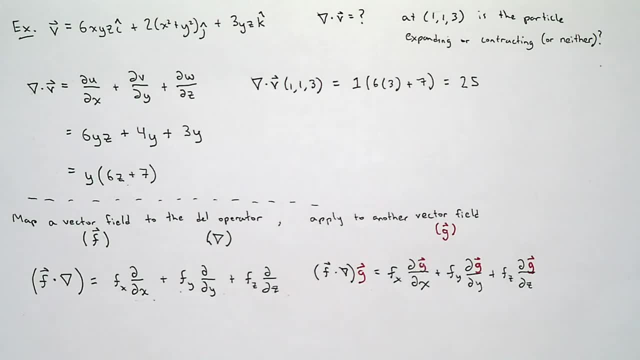 And we would still get the same results. Now, why do we do this? So there's actually some interesting math behind mapping vector fields, But the reason we care about them is because we're going to end up with an interesting relationship between the del operator and the material derivative. 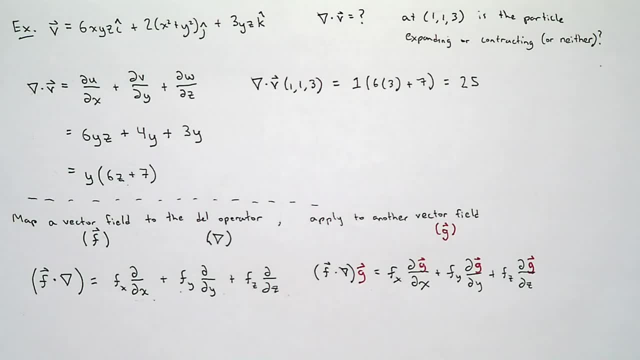 if we use these mapping functions Now. earlier Drew asked if the only difference between the del operator, or the divergence, and the material derivative was that the material derivative takes space and time. the gradient takes space, And my answer was yes and no. That is one of the differences, but it's not the only difference. 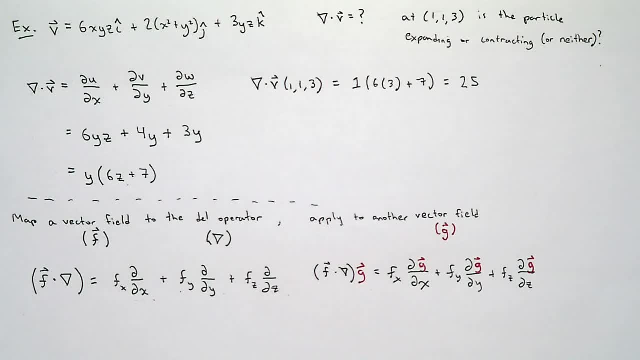 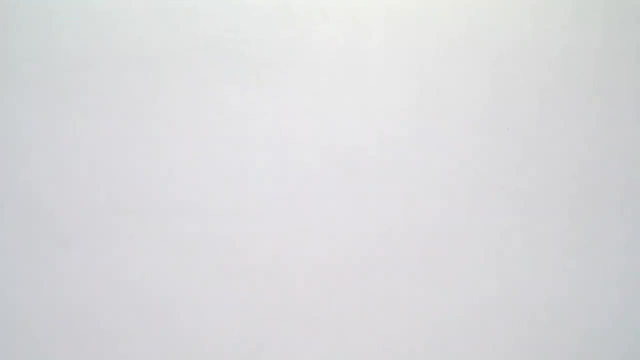 But now, using this idea, we're going to see how the del operator can be related to the material derivative. So what we're going to do is we're going to map this onto something here. He found out that look the del operator. we're looking at space. 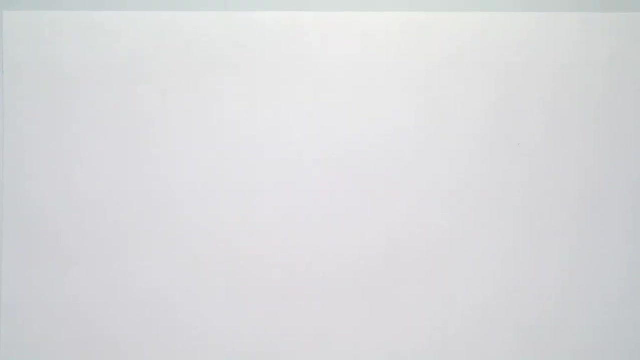 The material derivative. we're looking at time. So who knows, Maybe there is a relationship between them. So what I'm going to do is I'm going to map my velocity field to the del operator And then I'm going to apply it to the same velocity field. 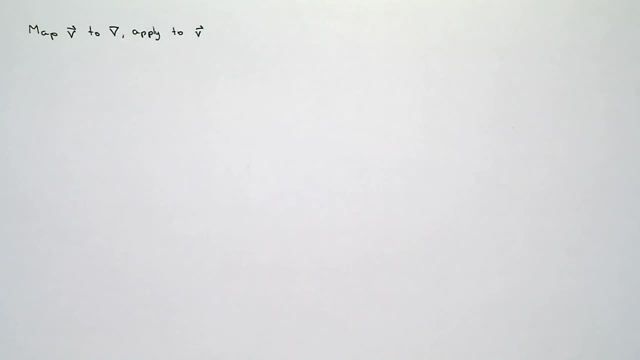 OK, So let's take it one step at a time. First, let's map the velocity field to the del operator. Now what do you think that will look like? It would be like u the partial of x, Yep Or the partial of x, then v times the partial of respect to y. 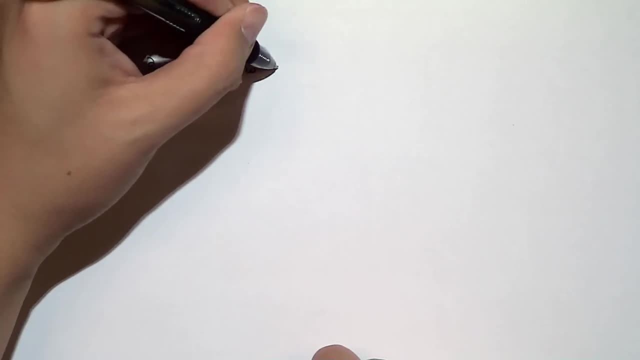 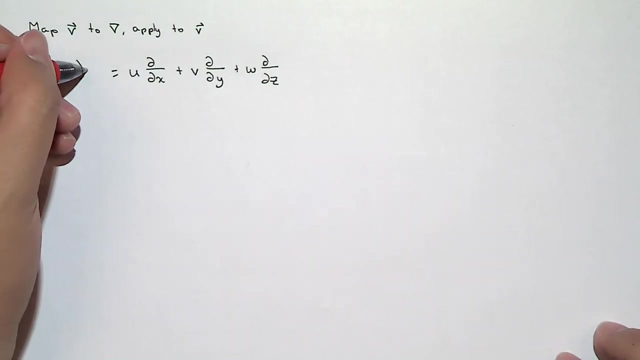 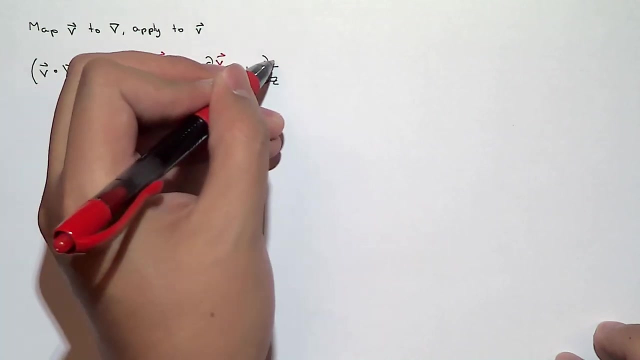 and w times the partial of respect to z. OK, Thank you. Does everybody agree? Yeah, And now let's apply this to the same velocity field. All we do is apply the operation to my velocity field. Now, why am I doing this? 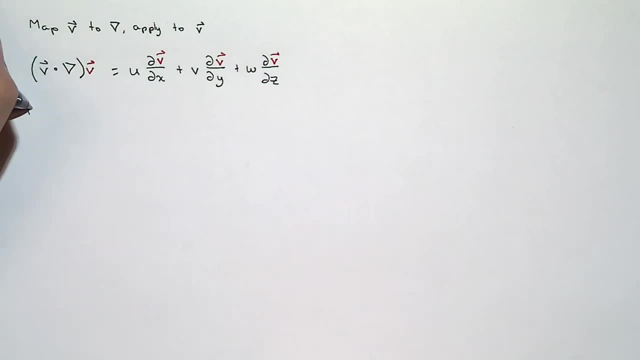 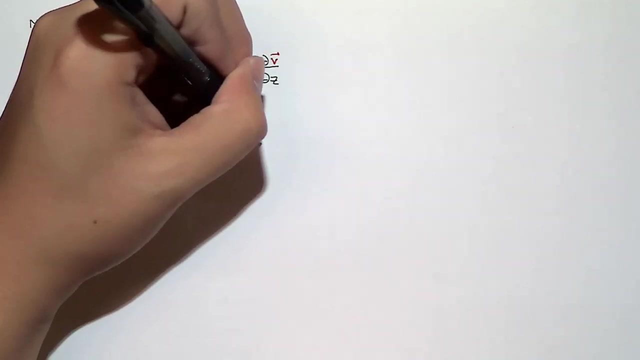 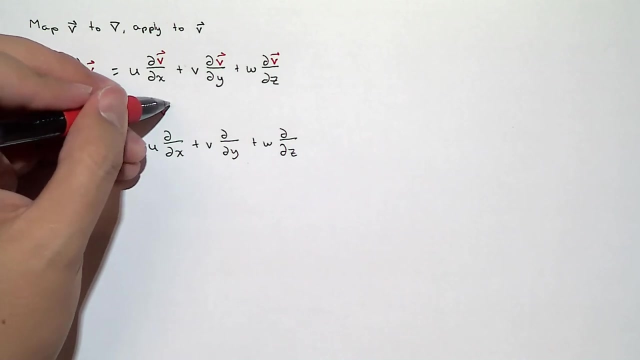 Well, what's the use of this? Well, let's recall the material derivative. The material derivative simply looks at the temporal change plus the spatial change And notice that if we take the material derivative of velocity, which is acceleration, then we get the temporal change of velocity. 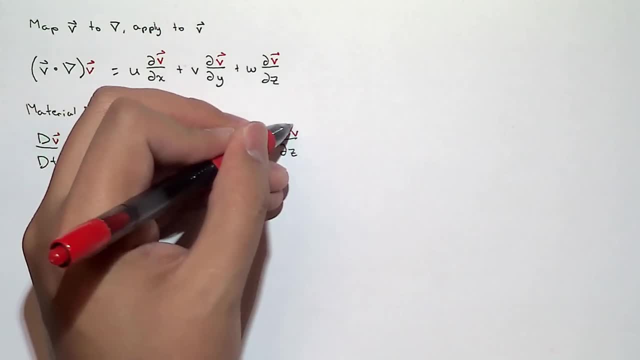 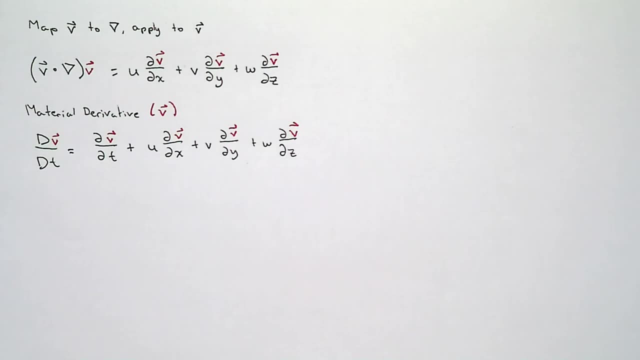 plus the spatial change. And now what can you see right there, The temporal change of velocity. And now what can you see right there, The temporal change of velocity. That's correct, right? Notice that now this spatial change is actually. 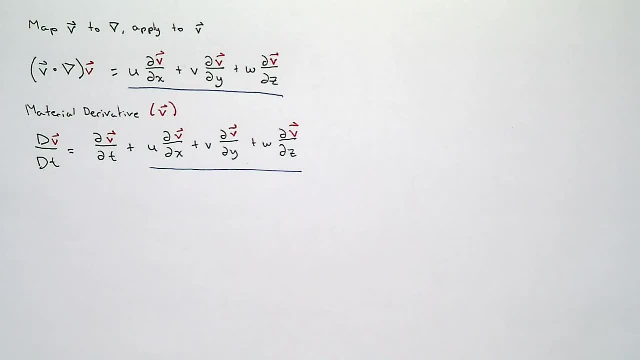 equal to the mapping of the velocity vector and the operator applied to the velocity vector. Now, because of this, you'll see that it's very common right to express the material derivative of any function as the partial change with respect to time plus v dot. 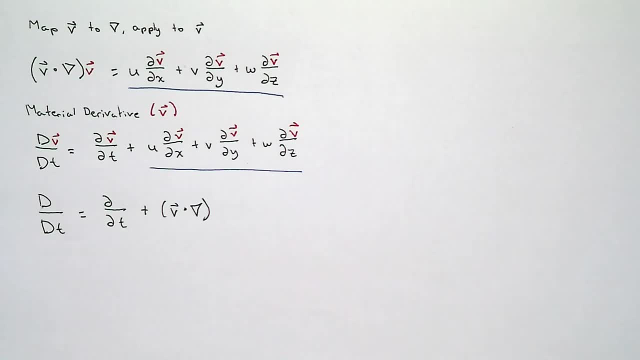 del applied to the function that you are deriving. Yeah, we're going to write it down. So it's just a material derivative, right? Just a material derivative, not applied to anything yet. So in this example, if we want the material derivative of velocity, 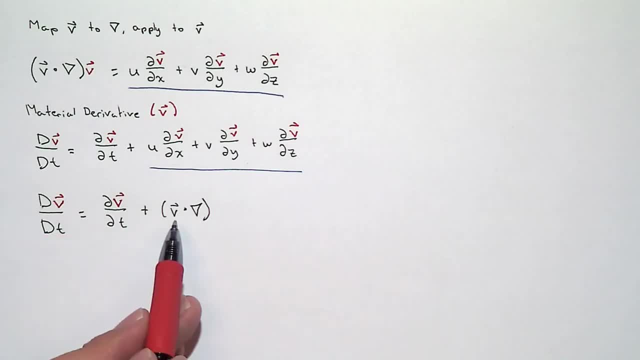 it would be the partial change of velocity with respect to time. It would be the partial change of velocity with respect to time, plus this velocity vector mapped to the del operator, applied to the velocity field. And remember that I'm trying to distinguish the red and black ink. 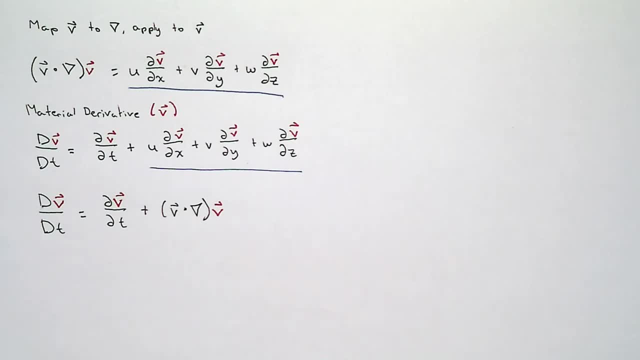 to let you know that the black ink essentially represents the operator itself. That doesn't change. But the red ink does change because you can apply the material derivative not just to velocity, but to any fluid property. Let's review this, For example: what if I want to find? 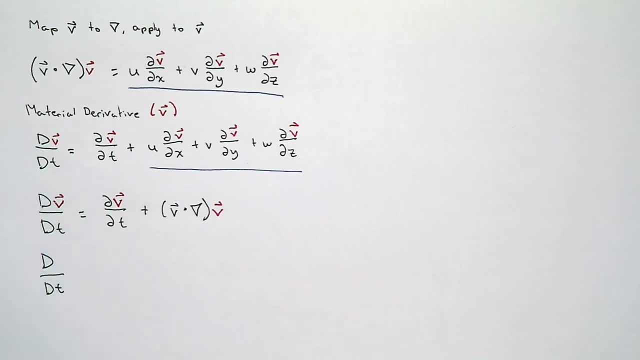 the material derivative with respect to time of density. Hannah, what do you think that would look like? Yeah, that's correct. The temporal change in density. What else? Yeah, that's correct, And that is the material derivative of density. 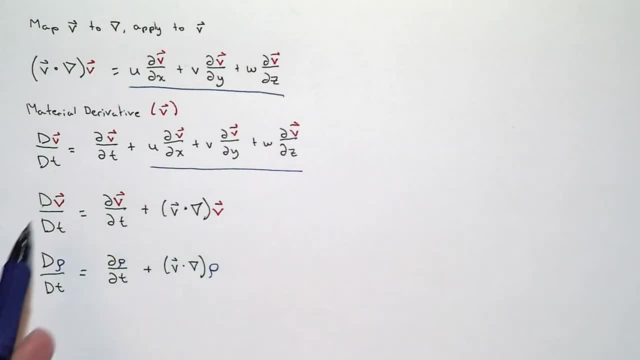 So notice that you can apply the material derivative to any And you can express it in this way: Yes, Yes, this is a mapped operator, So this will not change Because, remember, the material derivative includes this velocity flux right. 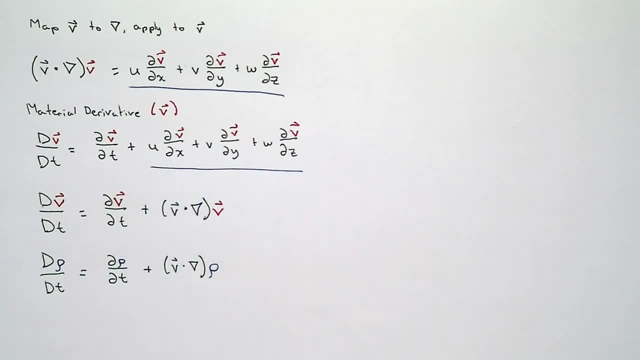 UVW, regardless of whether your properties, velocity or something else, And or something else. that's why I like to distinguish between the colors, because there are portions of the material derivative that depend on velocity, because material derivative depends on the movement of a particle right. 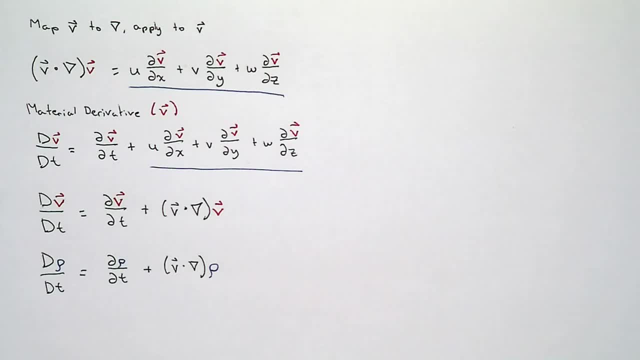 regardless of its derivative of velocity or derivative of something else. that's a good question. that's a good observation. okay, there are several vector identities that will be helpful to know, but that we will not have time to prove in this class and, frankly, we're not going to pursue them. okay, however, if you go into 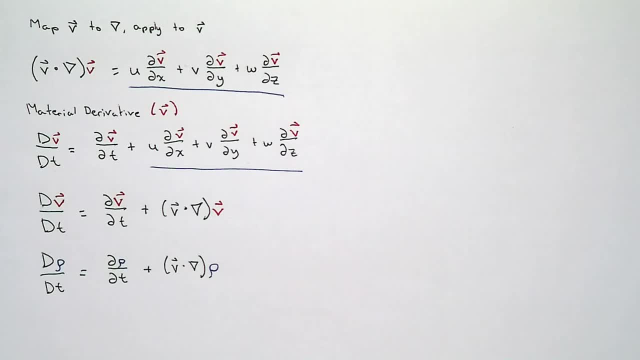 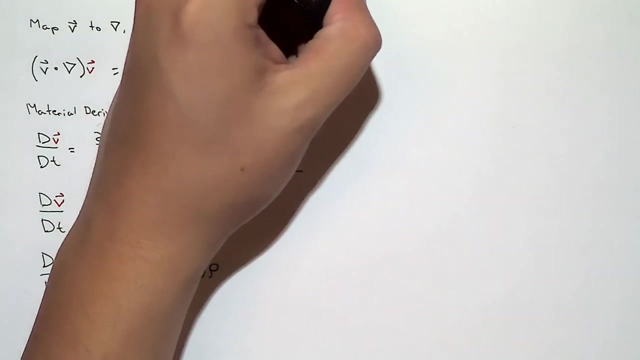 a further study of fluid mechanics beyond this course. you may see that some of your vector identities are expressed differently. so I'm just gonna give you a couple of examples and you can try the proofs yourselves, or you can contact me and we can go over the proofs. but one example is that this operator V dot del. 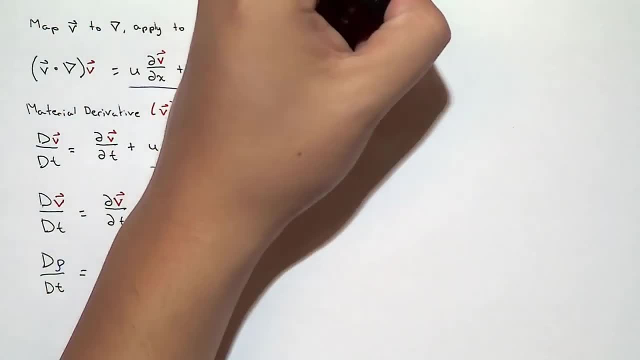 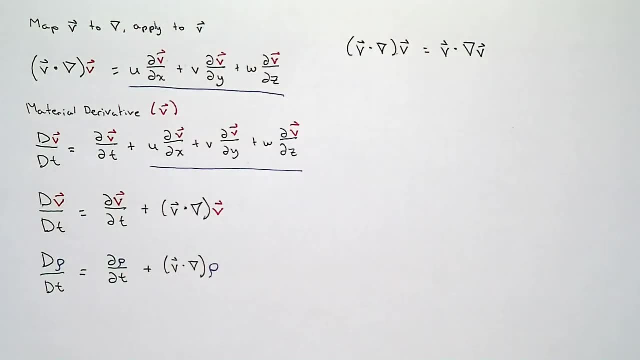 V can also be expressed and as V, dot del V. again, we can do a small proof and we'll find out that if you were to do both operations in both cases, you would end up with these three terms: U del del V del X, V del V del Y, W del V del C. so just a simple vector identity. 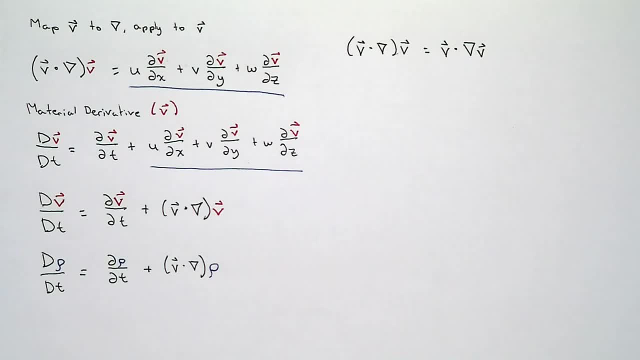 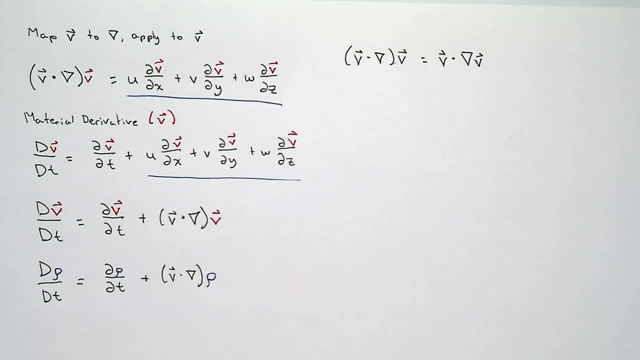 yep, yeah, you can call these two the dead piece. yeah, I was just showing a vector identity that we're gonna see, or you may see if you study fluids further. you know, beyond this class, one more vector identity which is helpful to know, but again, we're not gonna spend dedicate too much time to it in this class would be. 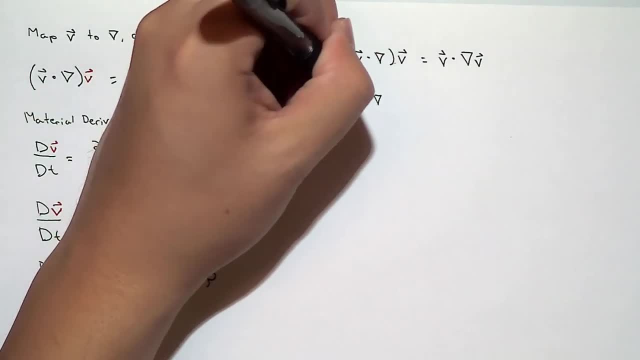 the vector identity with deal apply to V again is equal to v dot del y dot DOM for vector identity plus V to2 D always apply to v dot del when we're talking about formulation and functions vector to do. but again, we're not gonna spend dedicate to ourOur then we're not going to spend STEP up too much time to it in this class. would be the vector identitiy V dot Down, applied to V again is equal to vector identity with自 drawailed over the lower and this강athстoiffWeise Miyaga. 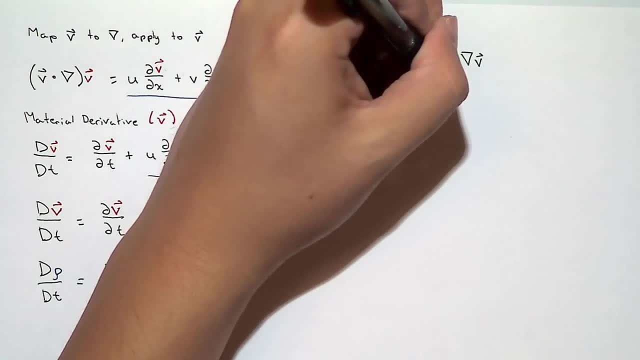 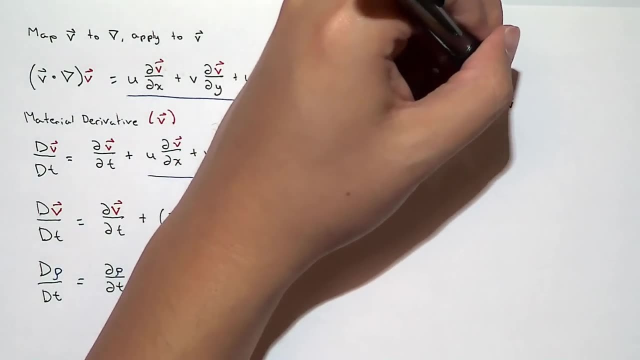 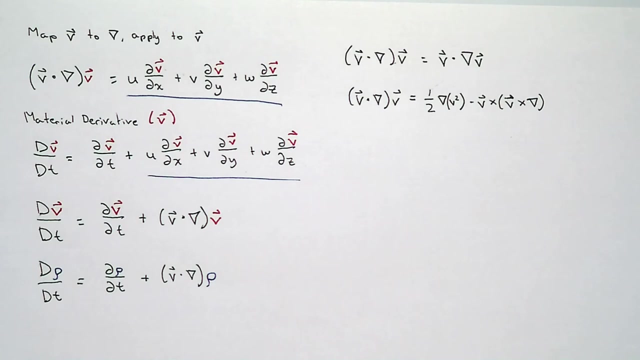 1 half of del V squared, so del of V squared. there we go. minus V cross, V cross del. And this one's a little bit harder to prove. In fact, just recently I had to prove this vector identity for a test. 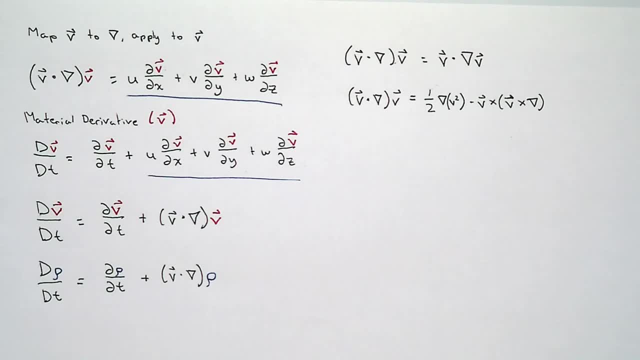 So it's a little bit harder to prove, but it's also a useful vector identity, which will help us simplify our problems in the future. Again, if you want to go over this proof, we can go over it outside of class hours. 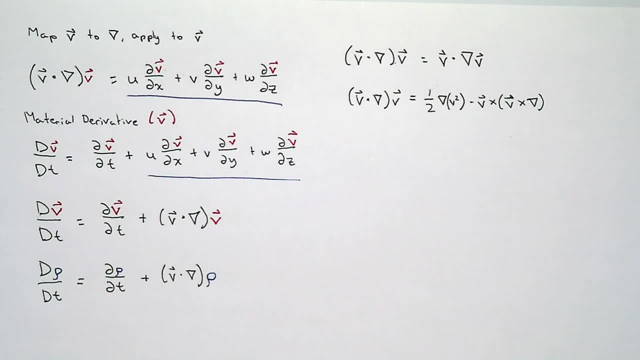 All right, Okay, So the reason I'm giving you these vector identities is because sometimes it will make our lives a little bit easier in expressing some terms in different ways, and that helps us to have different forms of our equations that we will find usable. 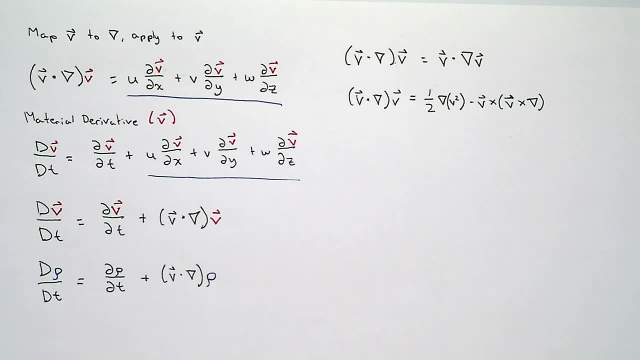 Yes, Oh, is the V squared? there is that the vector: Scalar, Scalar. That's the magnitude of V. The magnitude, Yeah, that's why I don't include a vector arrow. It's an interesting property. Like I said, we can go over it later. 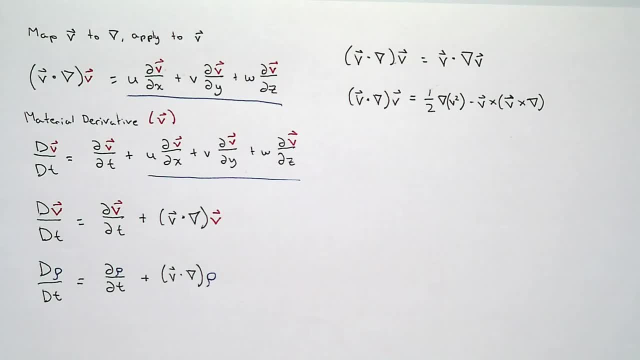 But yeah, these are some of the two vector identities that you'll see in some books. I personally don't like having to be like: okay, this is a vector identity, We can prove it later, but I'm not going to show you the proof now. 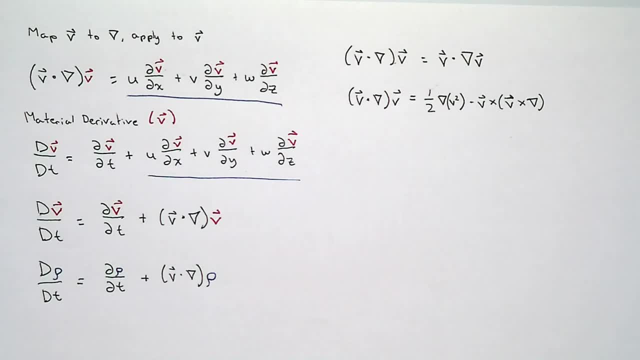 However, we're a little bit short on time. Okay, What I want to do today to wrap, To wrap up this class, because we do have about 20 minutes left. I'd like to actually derive an equation with you, Because, you see, when we did our integral analysis: conservation of mass momentum and energy. 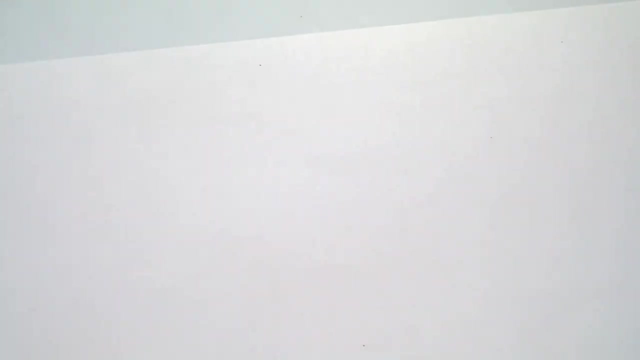 we derived a bunch of equations, right. We derived the continuity equation for mass, we derived the momentum equation and a deflector variation for momentum, and we derived the energy equation for energy. We derived the Euler and Bernoulli equations as well. 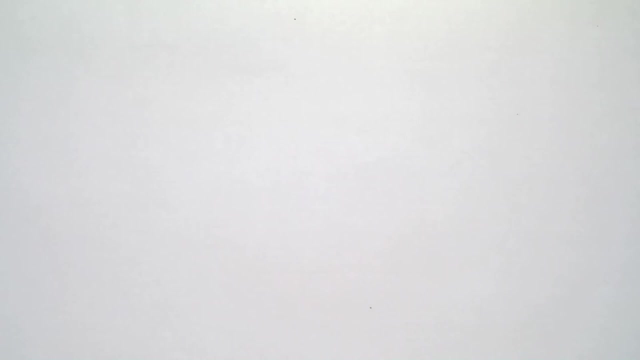 So I want you to see how the equations look, What they look like in differential form, because you'll see that there is some use for differential analysis. You see, in all of our integral equations, they all depended on us knowing the geometry of our control volume. 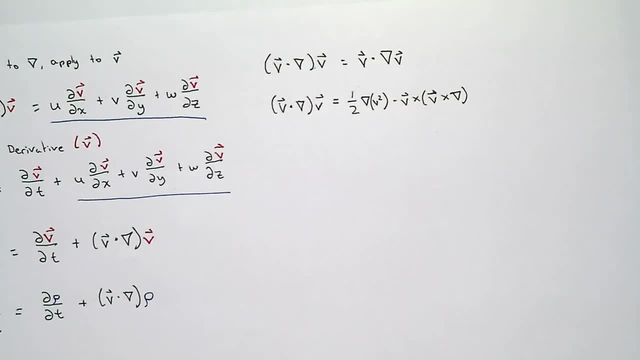 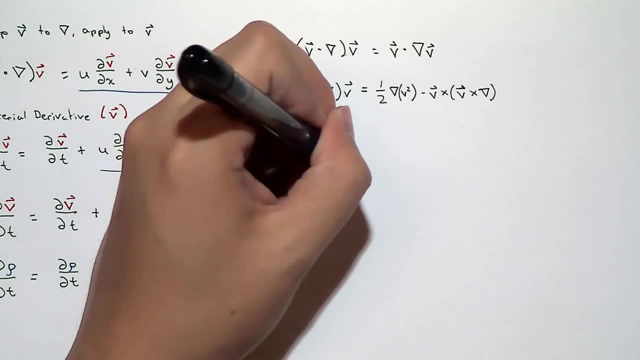 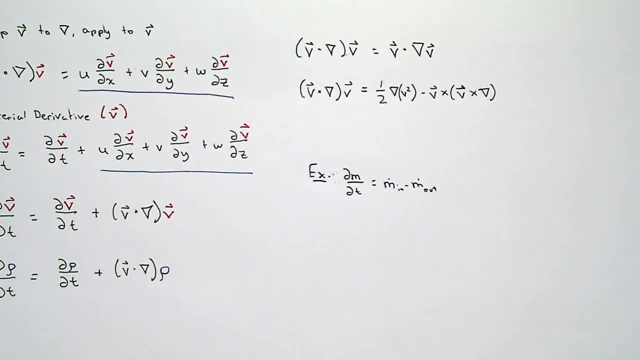 So let me go back to a quick example. This is just an example. When we came up with the equation of conservation of mass, we ended up with the equation: partial m over partial t equals mass flux in minus mass flux out. This was our conservation of mass equation, if you remember, from a few weeks ago. 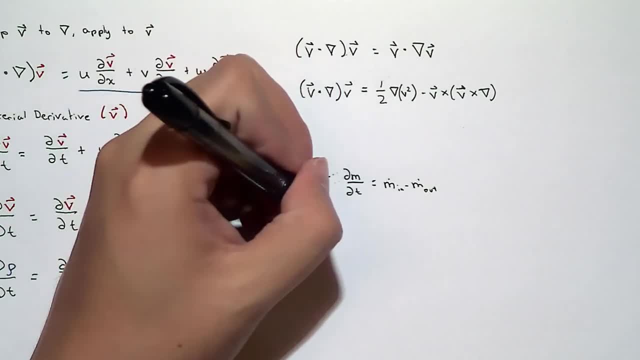 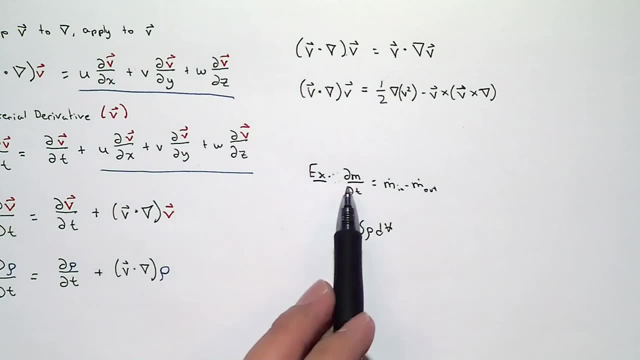 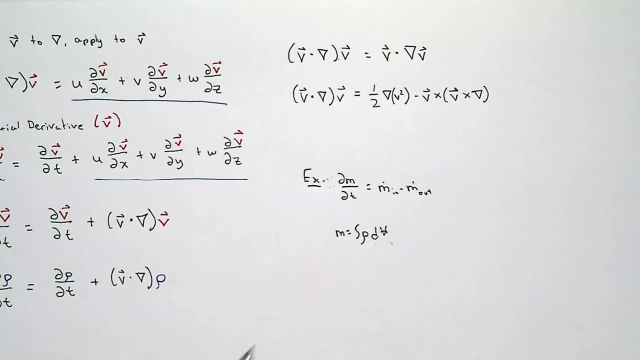 But there's a problem. Notice that mass is equal to the integral of density over volume, which means that to find the mass, in order to find this change in mass, you need to know the properties of the control volume. Of course, for most of our fluids, we assume that the mass wasn't changing with respect to the control volume. 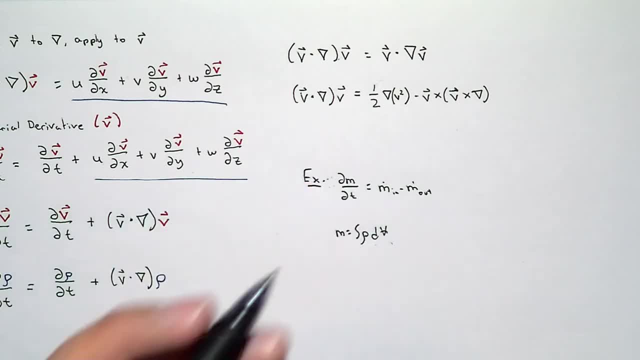 So we can just eliminate this term. But even if we look at our mass flux, if we're looking at mass flux in or mass flux out, remember that mass flux is equal to density times v, dot, a In the case of the velocity and area vectors pointing in the same direction. 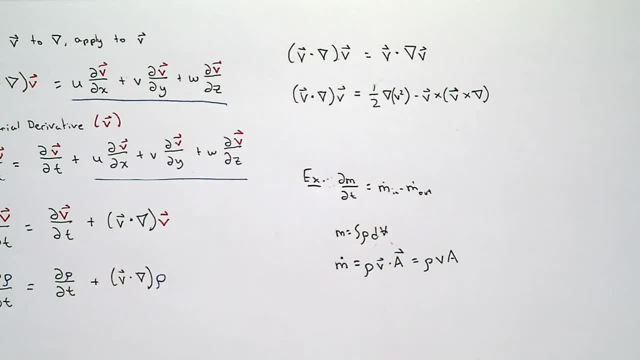 we can express mass flux as density times v times a, But in either case, we need to know the geometry of this area in order to solve this equation. So what this tells me is that the equation that I found for mass, and likewise the equation that we found for momentum and for energy, 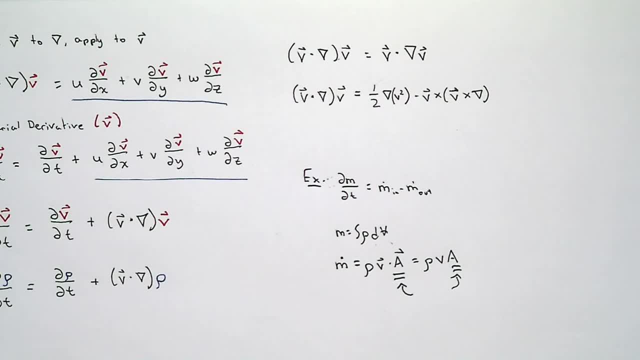 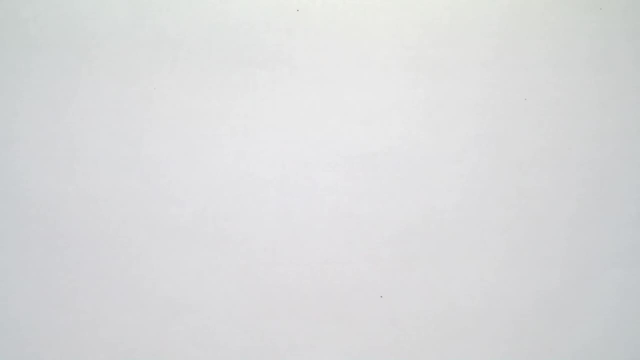 they require us to know some of the geometric properties of the control volume. Now differential analysis seeks to address this issue by deriving equations that are not functions of your volume. In other words, we want to derive equations for properties per unit volume. So in the case of mass, for example, 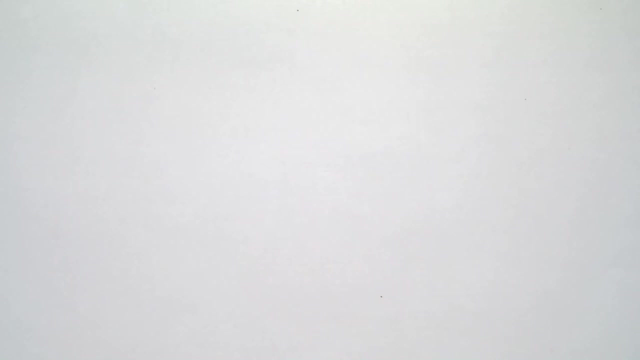 in the case of the continuity equation, you know, conservation of mass equation. instead of finding an equation that gives us the mass of a system, we would like to find an equation that gives us the mass per unit volume of a system. right? 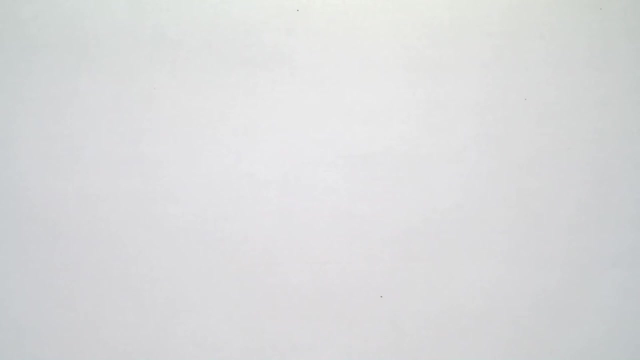 And what's that? mass per unit volume, Density, right, So what we're gonna do is we're gonna see how we can transform the continuity equation into an equation that relates to density and that we can express in different ways. Okay, and let's look at this equation. 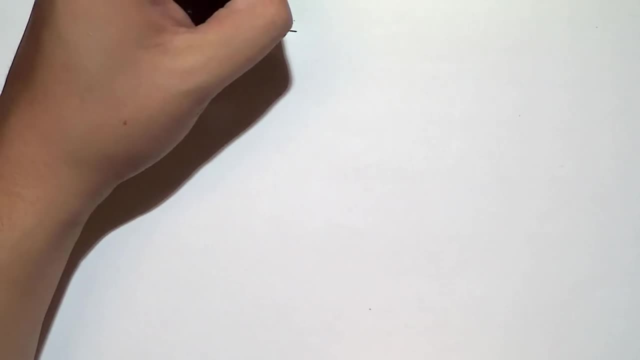 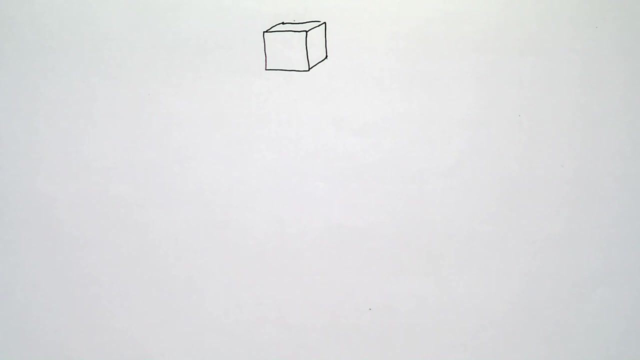 using a picturesque solution. This is okay. this is the function: a certain number. Hey G's loh. This is this ratio thing together with Sn, and it's going to have the ratio in-between D and O, 0.. So here's the ratio. 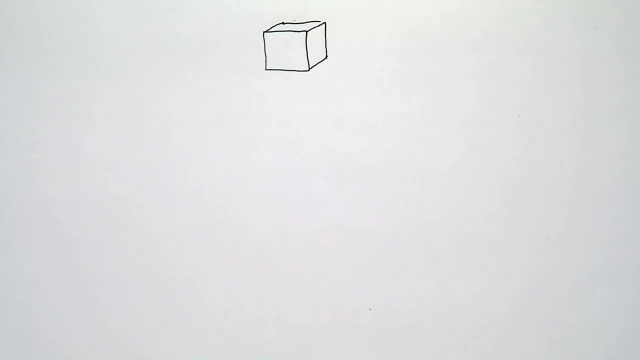 This is the finite teacher. So we're gonna use the interest value depend on the dimensions. I'm imagining it to be as small as possible, something that eventually I can get rid of that volume term. so we have a tiny control volume with fixed dimensions, right, and it's fixed in space, it's just standing. 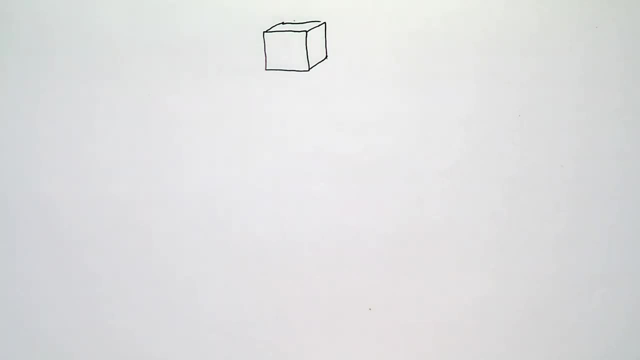 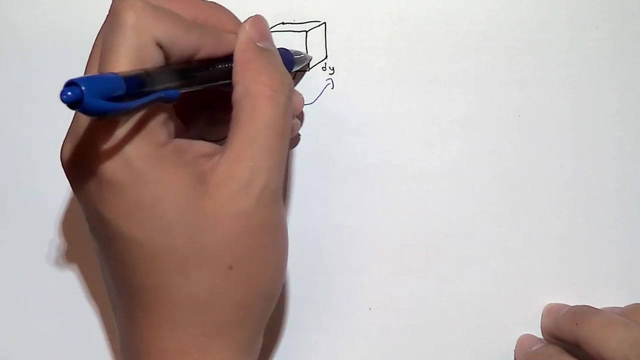 there somewhere. I'm gonna give it, of course, dimensions of DX, dy, DZ. and let's say that this control volume is right in the middle of a velocity field, so there's a fluid that's passing all through, as well as around this control volume. this velocity field is moving in some unknown pattern. let's not make it. 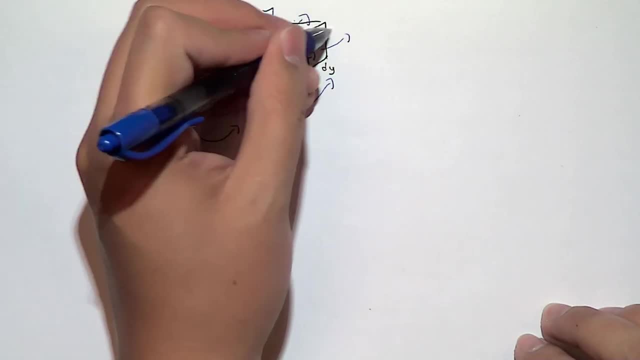 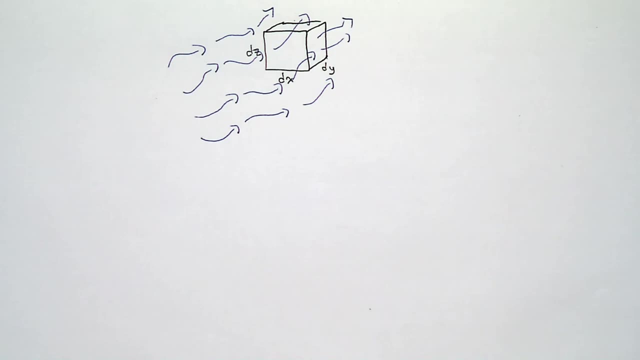 easy. let's not say that it's in the X or Y or Z direction. let's say it's in some arbitrary direction and we don't know the direction of the fluid. okay, so we have a tiny control volume. we have a fluid moving in some direction. 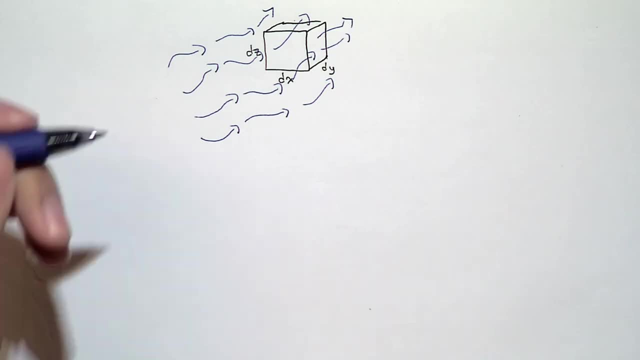 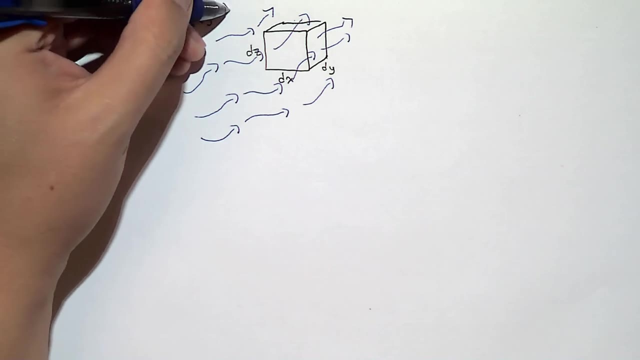 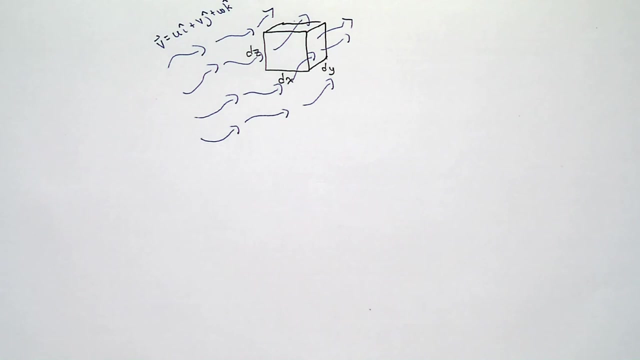 you. what we do know about the fluid is that the velocity field is defined by the vector u plus V plus W. that's the only thing we know about this velocity field. can we agree on that velocity field? you VW, which means that for the velocity of this fluid there's an X component, there's a Y component, there's a Z. 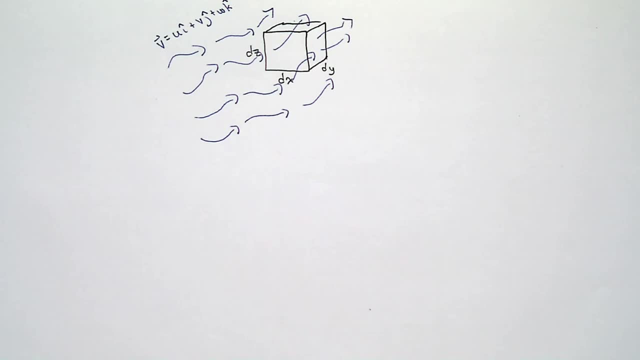 component. we just don't necessarily have to know what they are, at least not yet, okay. so now my question is: how do you know what the velocity field is and how? my question is: how can I express my continuity equation, my conservation of mass equation, in order to understand or study the fluid as it passes through? 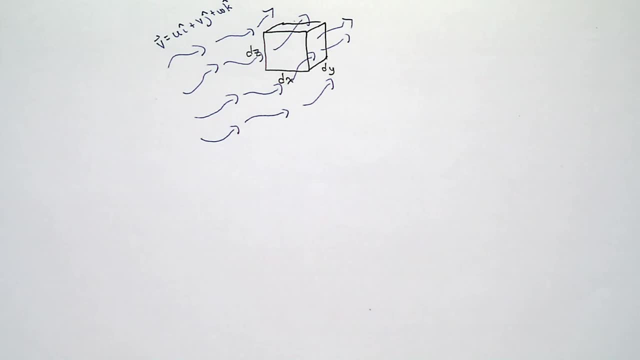 this control volume and we'll see that, even though there's a lot of equations and it it's actually a pretty intuitive approach. so let's start with conservation of mass. we know that conservation of mass tells us for a control volume. the change in mass with respect to time is equal to mass flow. 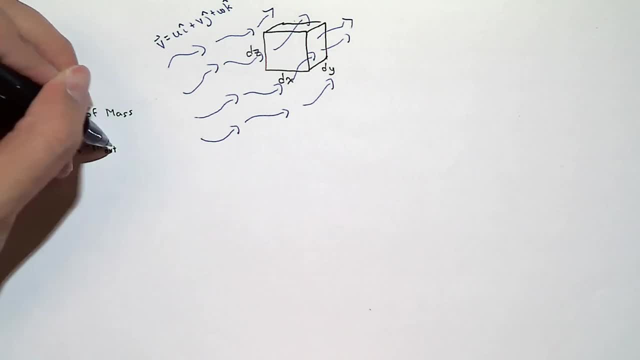 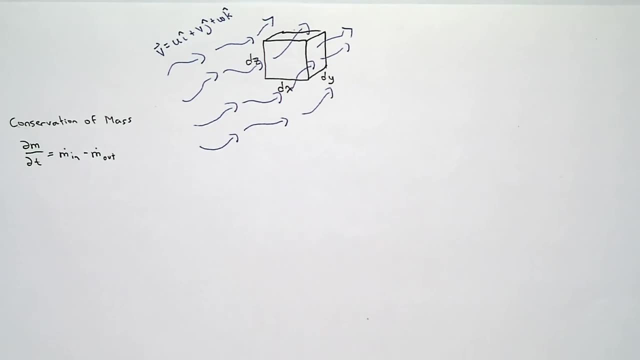 x in minus mass flux out. we've already derived this equation by using the Reynolds transport theorem, but we don't want to keep using this equation because we already said that this equation requires us to know the dimensions of this control volume and we don't want to know the dimensions of control. I want an. 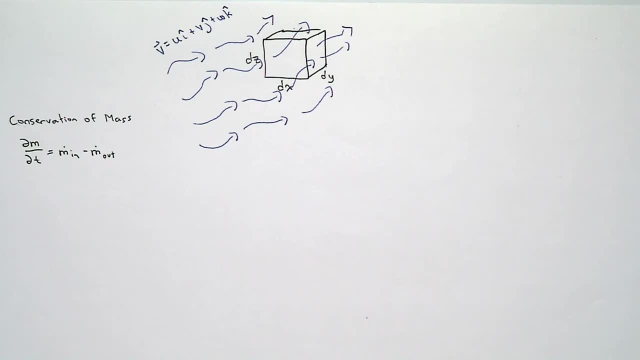 equation that applies for any control volume with any dimensions possible. so what I'm going to do is I'm going to first try to figure out how I can express the terms in this equation in terms that I can then use to eliminate my control volume. so let's start with this first term, the change in mass, with 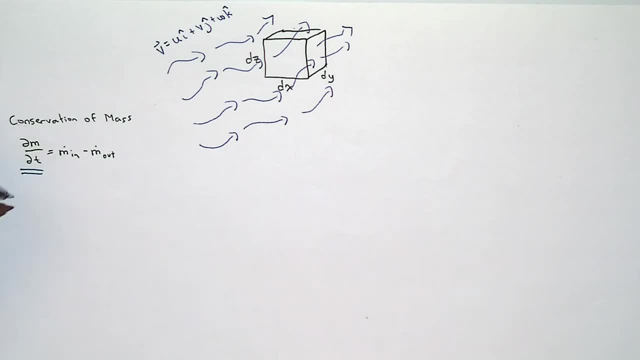 respect to time. now, the change in mass with respect to time. we don't want to express it in terms of mass. so we can express mass in terms of something else. right, if we want to express mass in terms of something else, what would that thing be? but what fluid property relates most directly to mass? density? good, 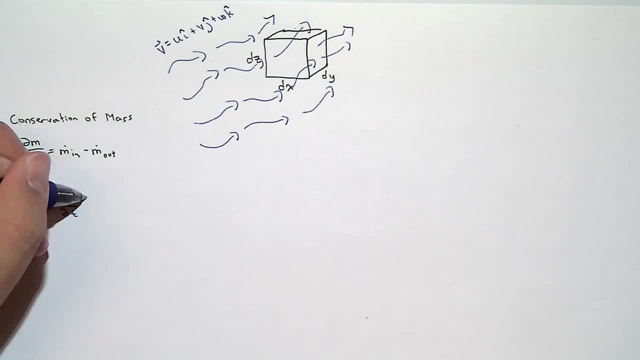 so we know this is actually equal to the change, with respect to time, of the integral density TV. right now, my control volume is really really, really small and in fact the reason we're making this control volume so small is so that there is no discernible density variation through the volume itself. there may be. 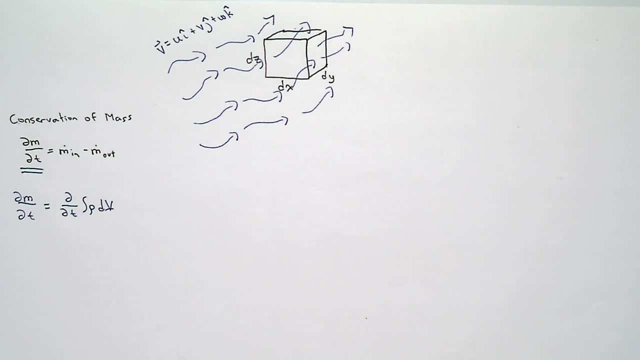 variation in any one direction, perhaps in the x-direction, perhaps in the y direction, perhaps in the z-direction, but not throughout the volume itself. think of it in terms of average velocity right. even though we may have variations in the velocity field inside a pipe, we can still study the flow as if. 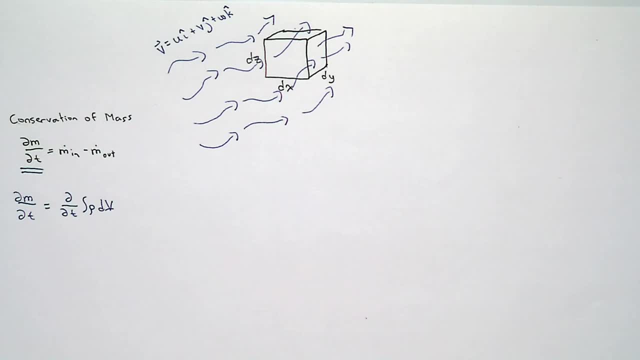 there was an average velocity throughout the entire pipe. so we're going to do the same thing for density. I don't want to call it average density because that wouldn't be a correct term, but it's essentially the same philosophy behind it. now, if we're studying density as if 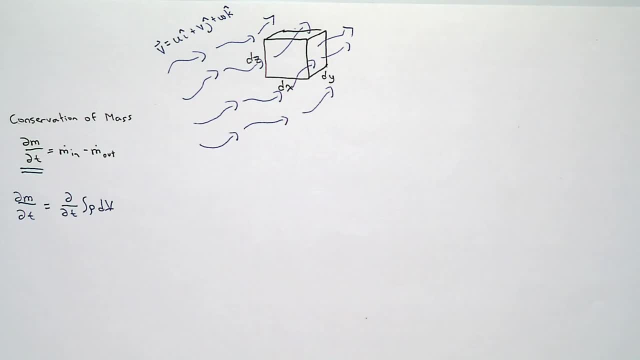 there were, only there weren't enough variations for this integral to depend on density, then what I can do is I can express this integral as the integral, as the derivative of, simply, density times integral of DV. okay now, based on what you know about this control volume- we mentioned that this control volume is 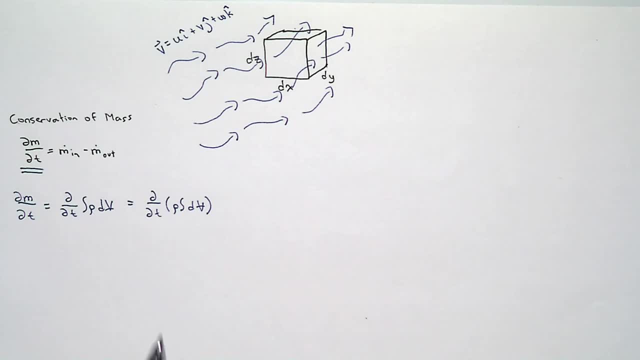 fixed. okay, and we see that the integral DV simply looks at a tiny, tiny, tiny volume expressed and added infinitely many times. and from what you know about integrals, the integral of DX is just X, so the integral DV is just what? V? right, so that means that this integral of DV represents. 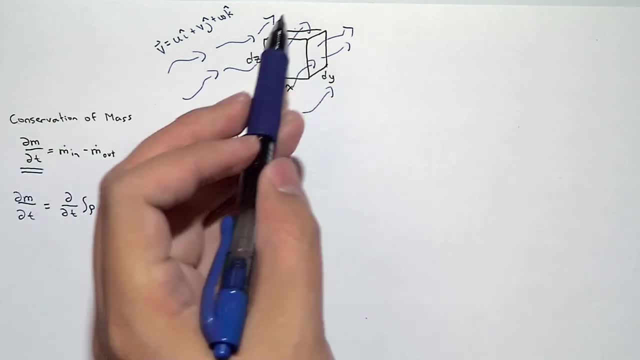 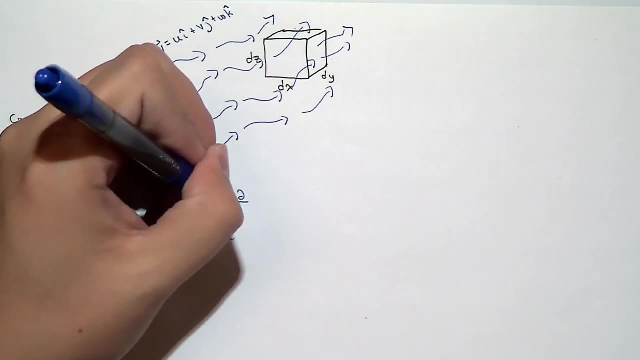 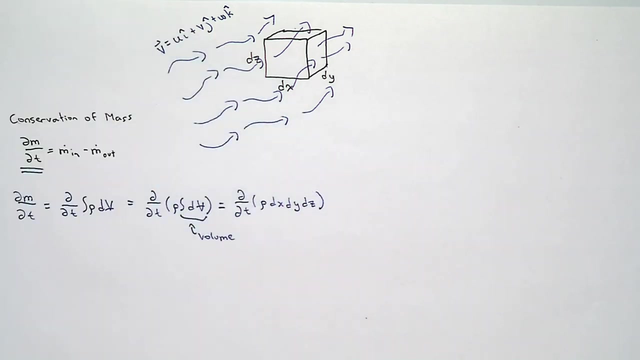 the volume of this control volume and what is the volume of this control volume? that's correct, so we get. that's correct, so we get that the change in mass with respect to time is equal to the change in density: times, DX times, dy, times, dz. with respect to time, now we have two different things. 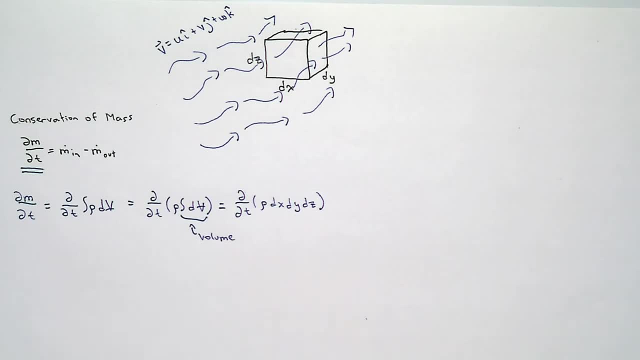 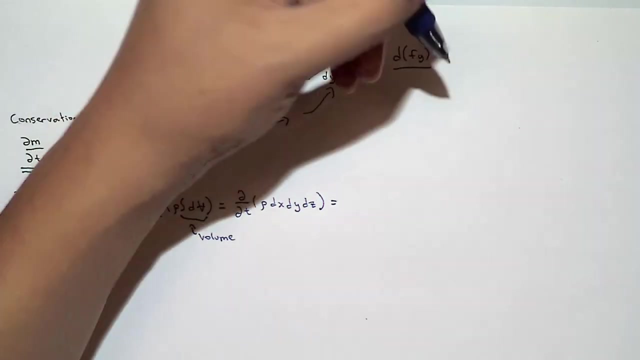 right, we have density and we have volume, so we can use the product rule to express this term. if you may recall, the product rule tells us that the derivative of two functions with respect to time- I'll just write it here- the derivative of two functions with respect to something, and let's say DT, because 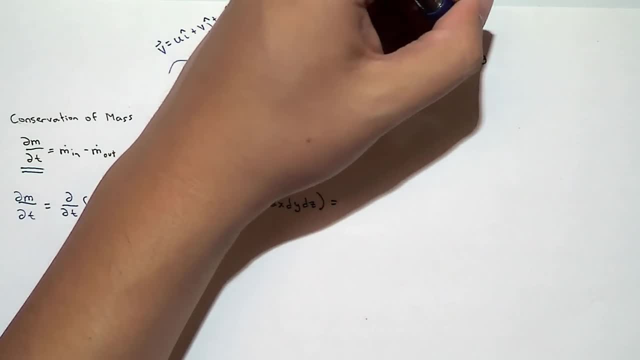 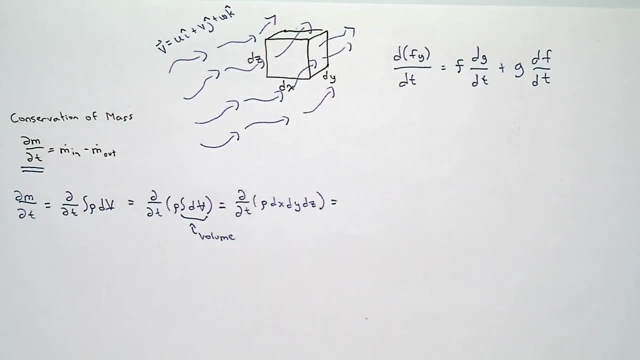 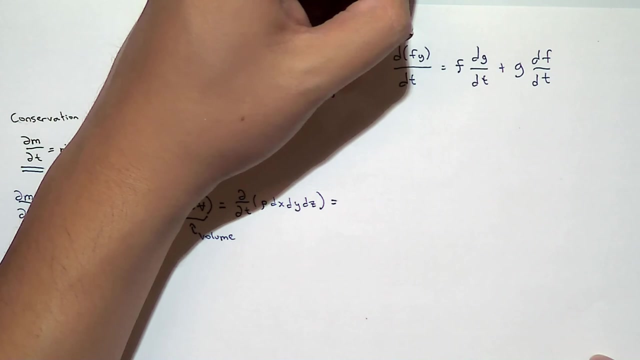 we're using time should be equal to the first function times the derivative of the second function, plus the second function times the derivative of the first function. do you, do you recall the product rule from calculus? yes, good, it's been a while, I know. I feel that I can say that as well, because it has been a while for me as 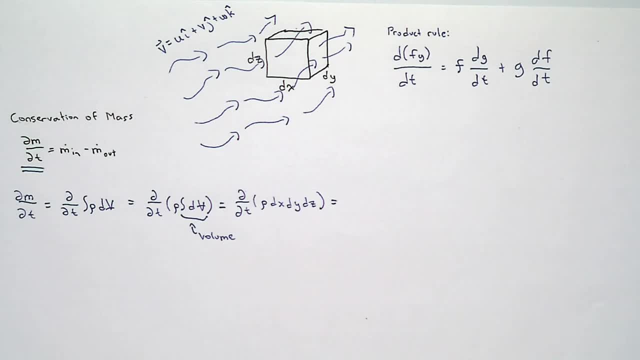 well, oh well, we already did derivative, material derivative. so that's about as much chain rule as you need for this class. so with the product rule we can express this and we can look at the first function as density and we can look at the second function as volume, because dx, dy, dz are intrinsically tied. 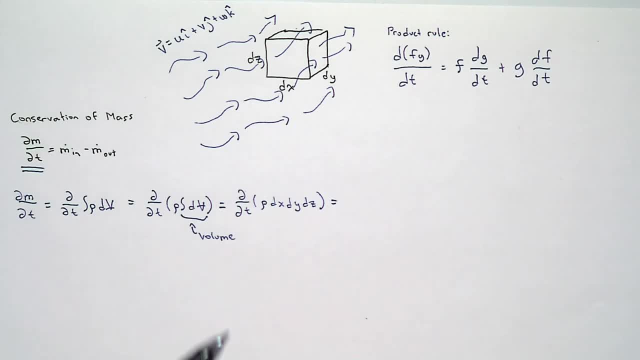 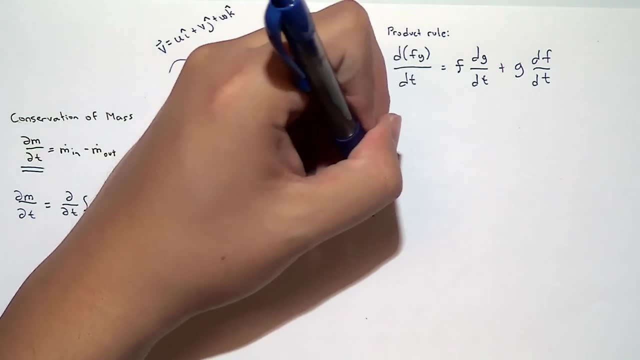 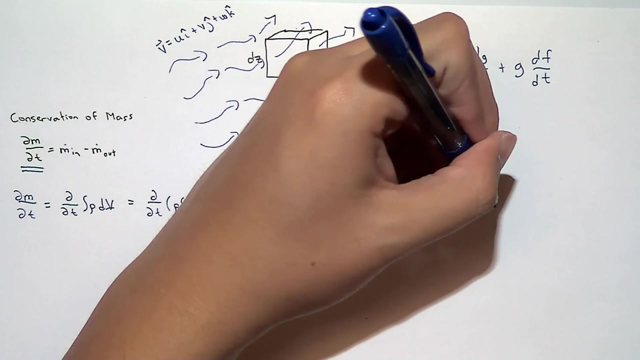 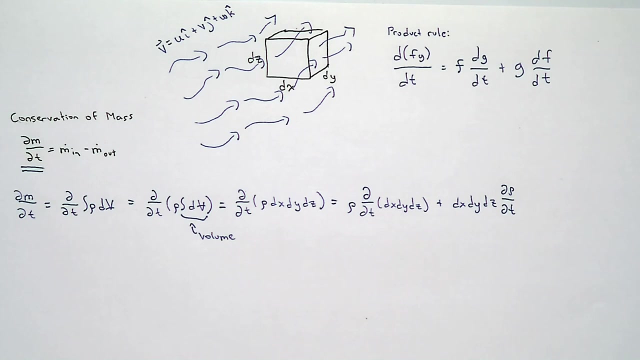 to each other their volume, right? so what do I get? I get that this would be equal to density times the change in volume with respect to time, plus volume times the change in density with respect to time. now we know a couple of things, right? my control volume is fixed in time and space. so what happens to one of 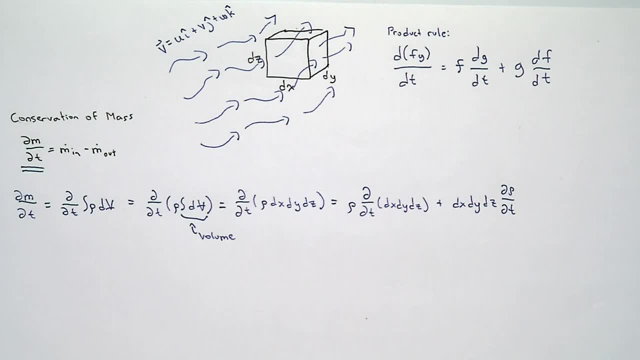 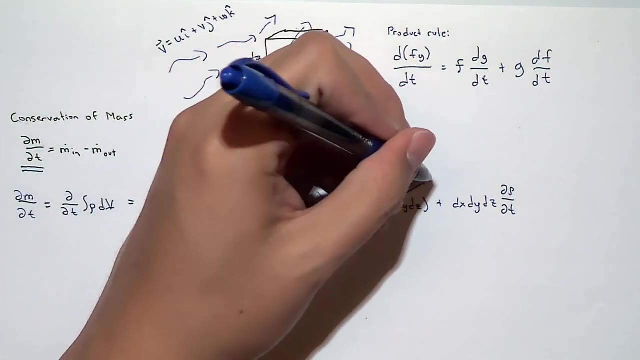 these terms: if my control volume is fixed in time and space goes to 0, right, the change in volume with respect to time is zero, because my volume does not change with respect to time, because i have a fixed volume right, fixed in time, fixed in space. so this is actually equal to zero. 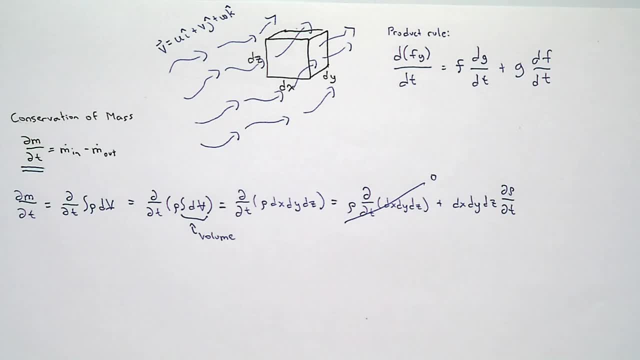 and i can conclude that the change in mass with respect to time is equal to my volume multiplied by the change in density with respect to time. up to this point, are there any questions? no good, we will once we deal with the other terms. so the answer is yes, just not yet. 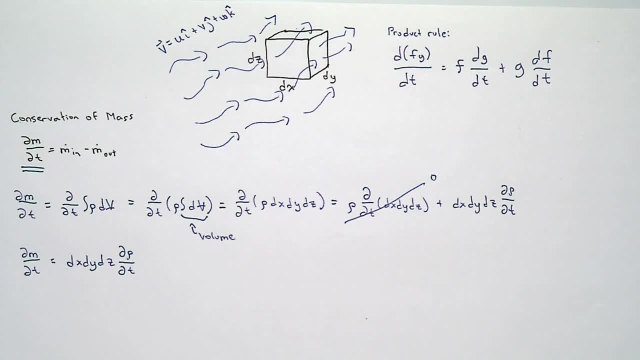 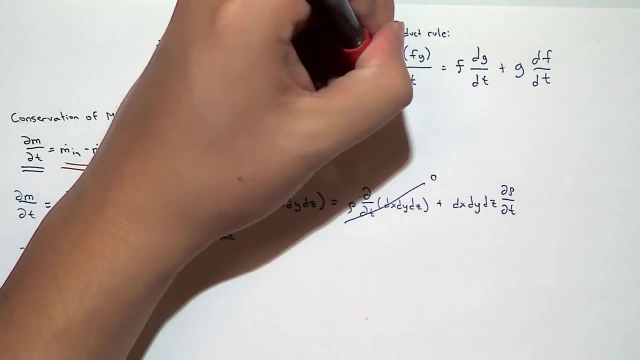 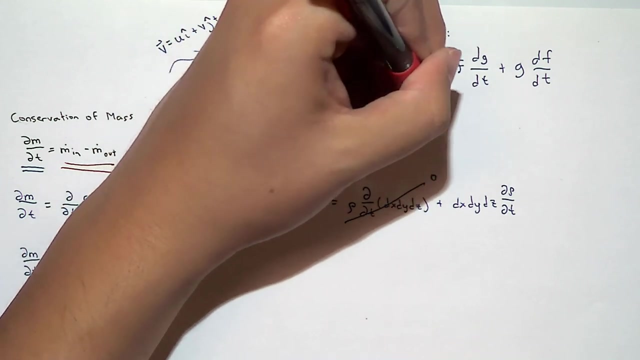 so, in order to get to what you're saying, right, we can cancel out the volume because it can be infinitesimally small. let's first see what these terms- mass flux in minus mass flux out- become. now. we had already, uh, recalled that mass flux was equal to density times velocity, dot area. 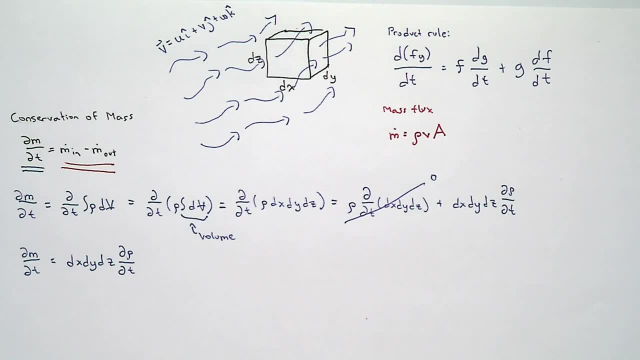 but if my velocity vector and area vector are normal to each, are parallel to each other, then i can conclude that the change in density with respect to time is parallel to each other. right velocity normal to the area. so area vector is parallel to velocity vector. then it's simply equal to density velocity area. now, because our mass flux depends on the 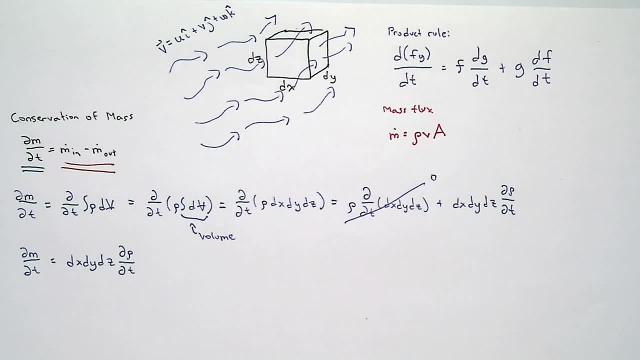 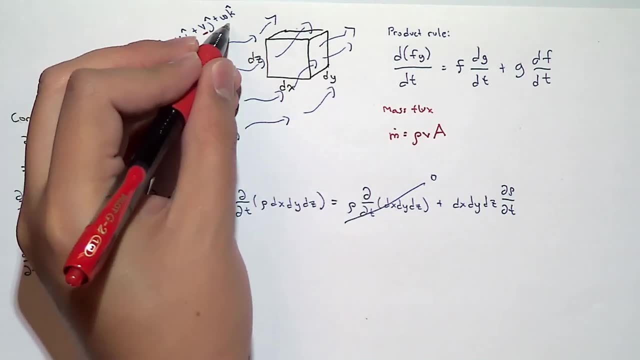 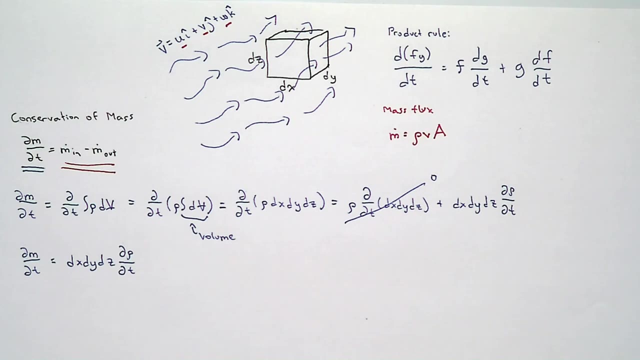 direction of the velocity field. i'm going to simplify my calculations by looking, instead of looking- at the velocity field as a whole, focusing on the individual components of the velocity field. in other words, i'm going to look at the x component of velocity and figure out what's the corresponding mass flux for the x component. likewise, i'll do the same for the y. 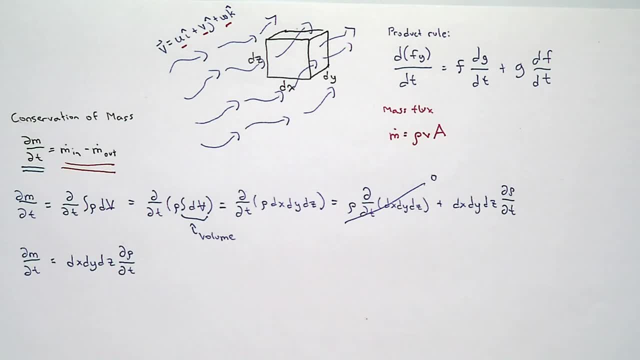 component and the z components of velocity. so in the x direction, okay, in the x direction we got to figure out what is my mass flux in and what is my mass flux out. so in the x direction, we know that mass flux in right represents the density, velocity and acceleration of the fluid as it enters your control volume. 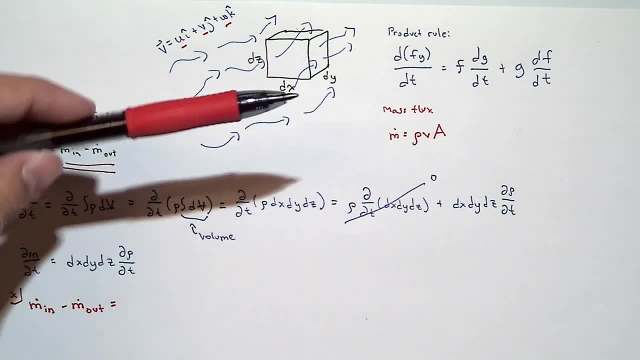 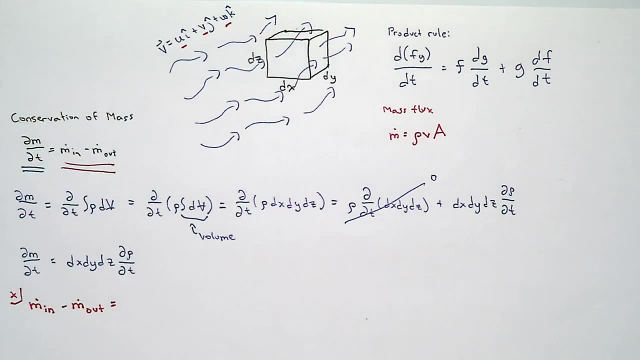 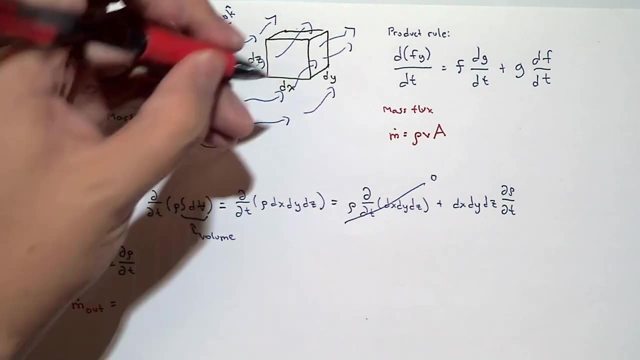 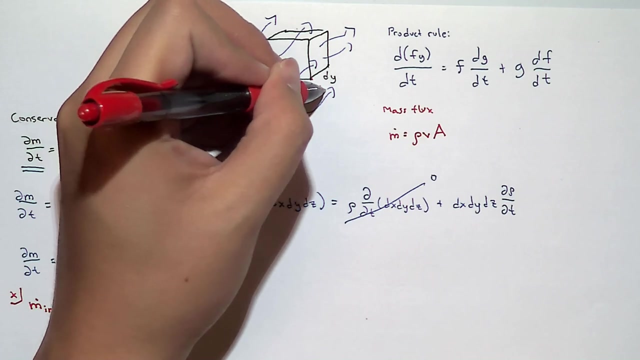 now, because there's only the X component of velocity. we only care about any velocity moving in the DX direction right, and this will actually make our calculus a little bit easier. you see, I can give this point a coordinate X, which will make this point a coordinate X plus the X. is that correct? we're just setting. 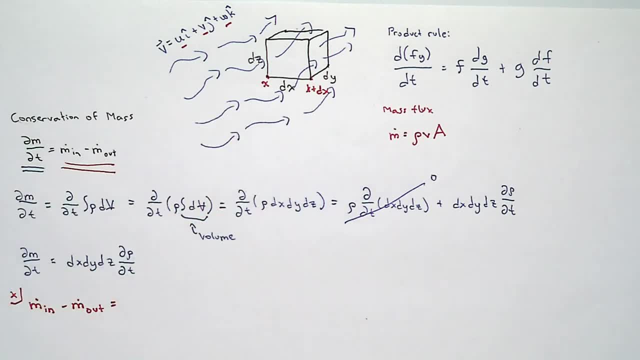 this control volume on an axis and this is just X and this will be X plus DX. doesn't have to be X, you can call it whatever you want. they can be zero, it can be one, whatever you want. okay now, because my fluid traveling in the X 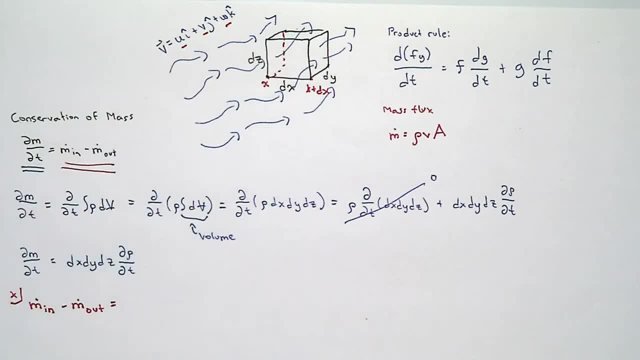 direction will enter the control volume through this face. then we will have the density at point X multiplied by the velocity at point X. but remember, we only care about the X component of velocity. so what should we write here, instead of writing the whole velocity vector? what do we write here? you right, so you at point X. 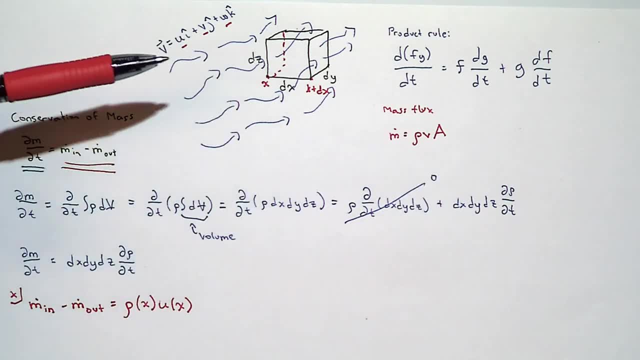 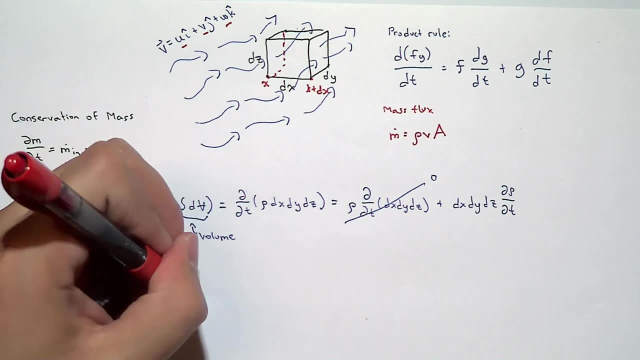 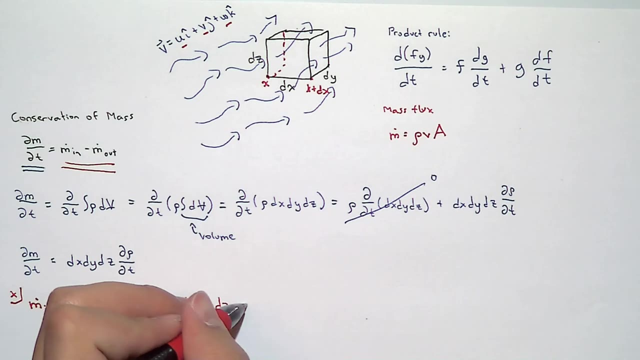 and then multiply by the area through which this X component of velocity is entering my control volume. what's that area? that's correct y, d, z, And that's my mass flux into the control volume. Likewise, I have the mass flux of the 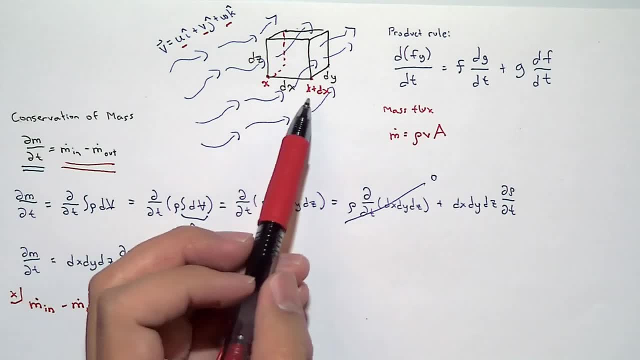 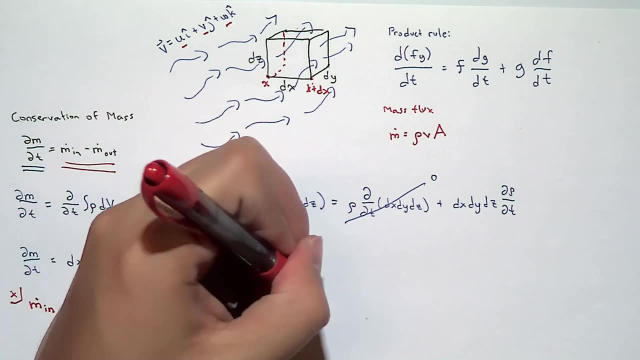 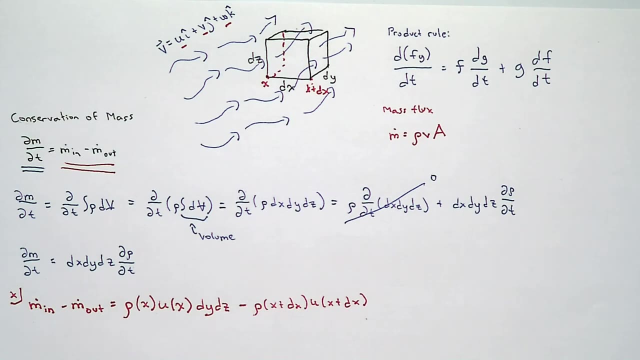 fluid leaving the control volume. We have the density at where it leaves the control volume, which will be x plus dx. We have the velocity at x plus dx. And again, this x can be anything you want it to be: It can be zero, It can be fish, It can be whatever, Just something. and 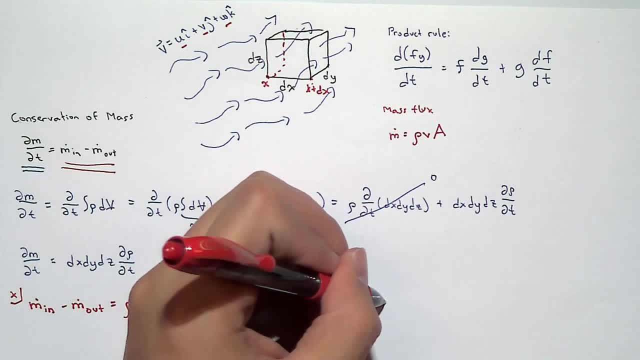 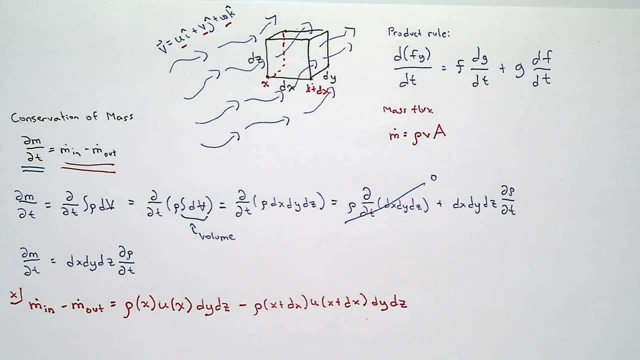 then something plus dx. I will take that as a challenge And I will accept that challenge. okay, So we have the mass flux in and the mass flux out of the x component. We can repeat this process for the y and z components And then we can express our conservation mass equation in: 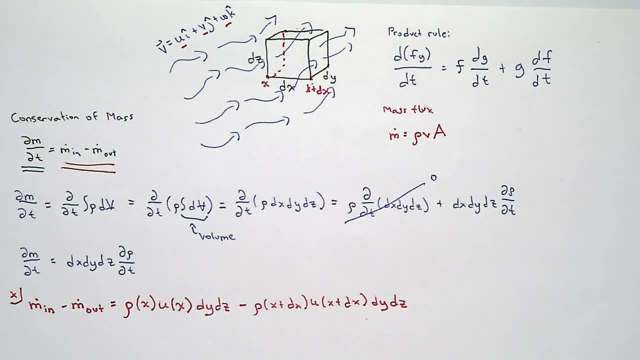 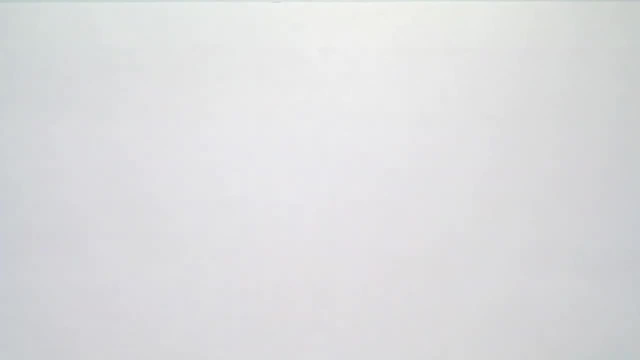 terms of these elements. So let's go ahead and do that. You ready, KC, Don't worry, It's not that bad, It'll be okay, You'll be fine. So what do we have? We have our conservation of mass equation, And we know that this was equal to the volume times the change in. 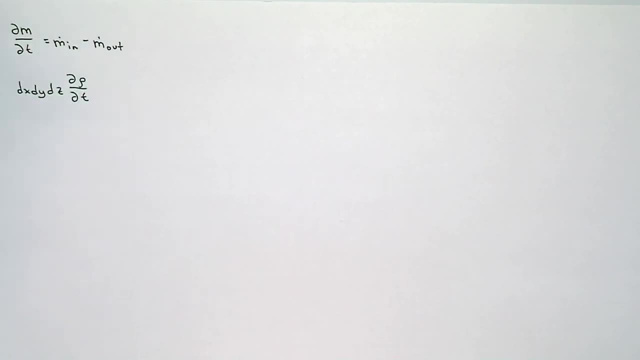 density, respect to time, and this is equal to mass flux in minus mass flux out. now i'm gonna, instead of keeping all my mass fluxes in on one side, mass fluxes out on the other side, i'm going to divide them by x, y and z components, just because it makes my equation a little bit neater. okay? so if i look, 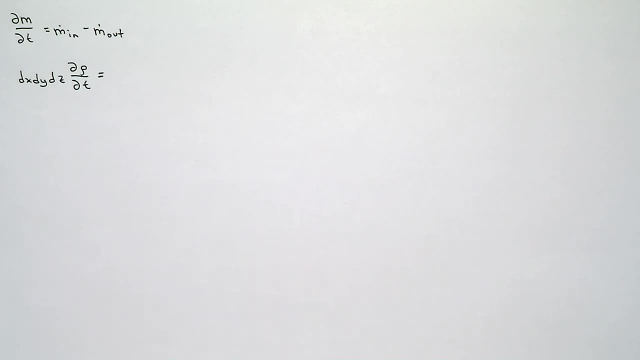 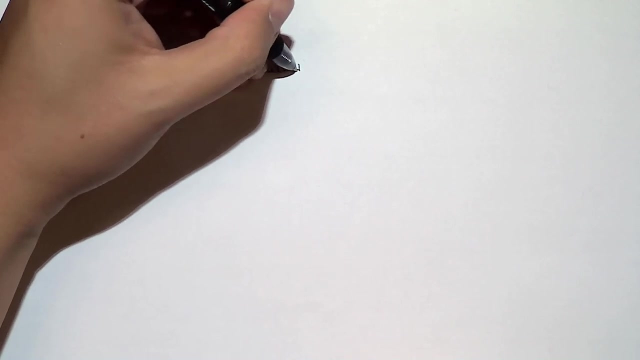 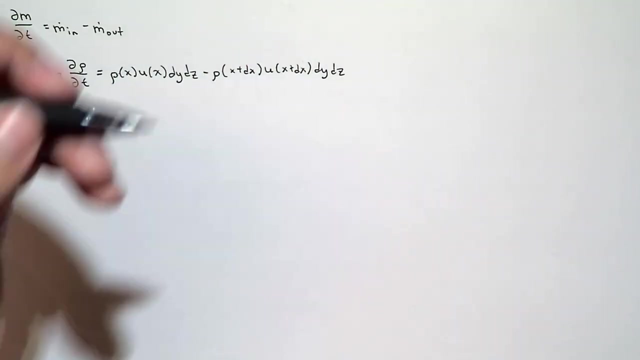 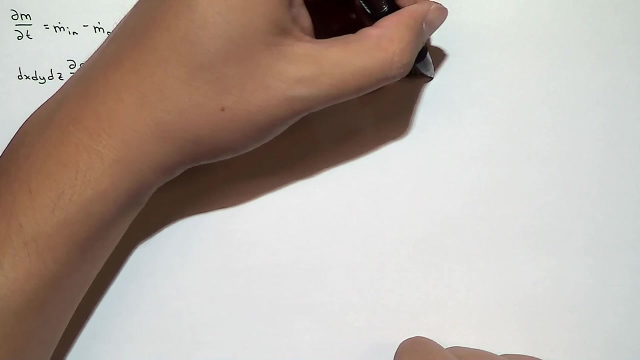 at my x, y and z components. we already had an x component for mass flux in which was: density at x velocity at x dy dz minus density at x plus dx. velocity at x plus dx dy dz. now that is for the x components. we can look at the y components: density at y velocity at y dx dz minus density. 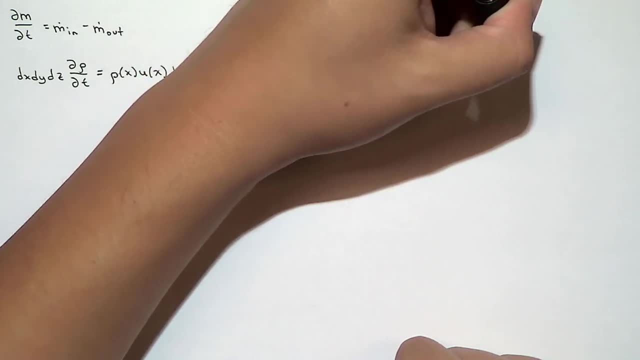 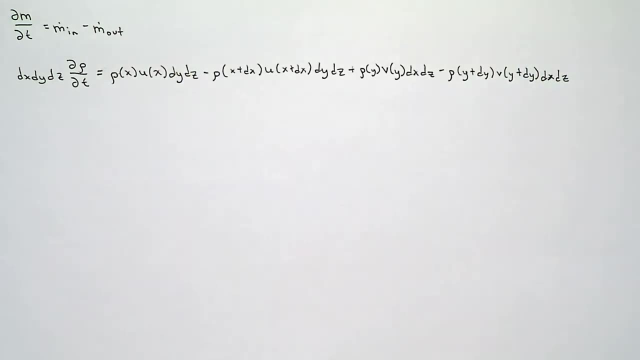 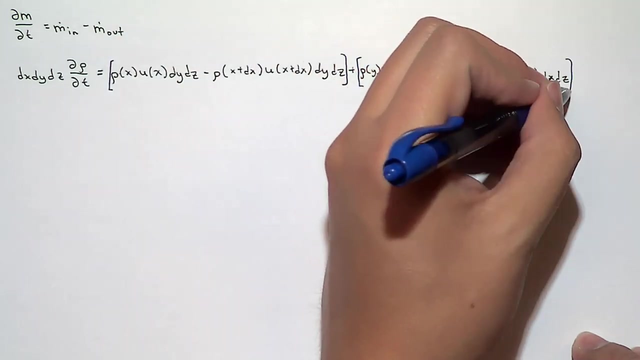 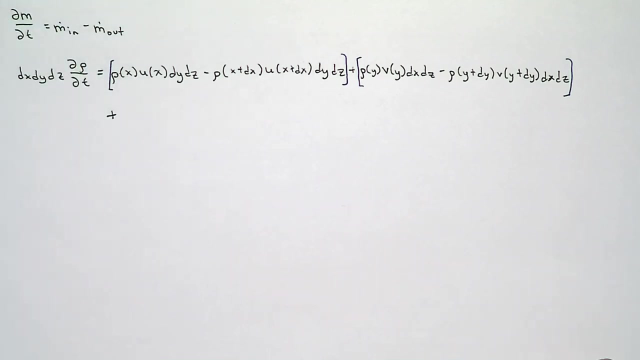 at y, y plus dy, velocity at y plus dy, dx, dz. does everybody follow where i came up with the y components so far? i do not mind, we have the x component, then we have the y components, okay, and of course we can't in and out work on some sort of complex flow and our dynamic component, and here, for example, we can. 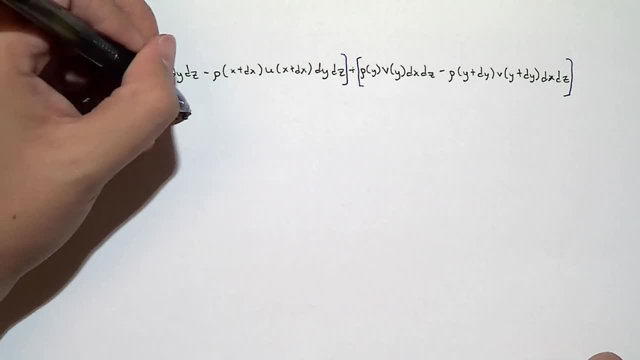 get minus x velocity at x plus z and minus x density at z plus dy, dx, dy, so you can have a z component, get, add up a z component, theoten, and you can borrow x and z phenol and that's basically it: minus x velocity at x plus z, dx dy minus z and – this is minus 1 upon plus sub 4 at. 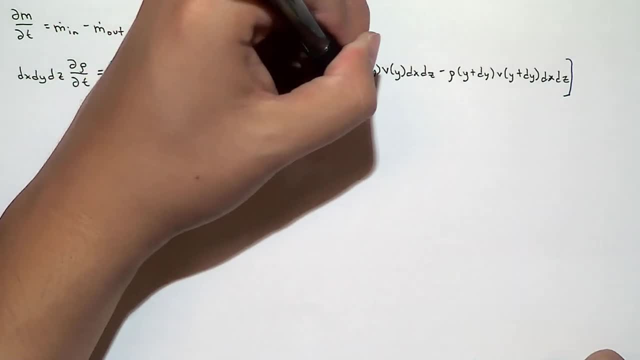 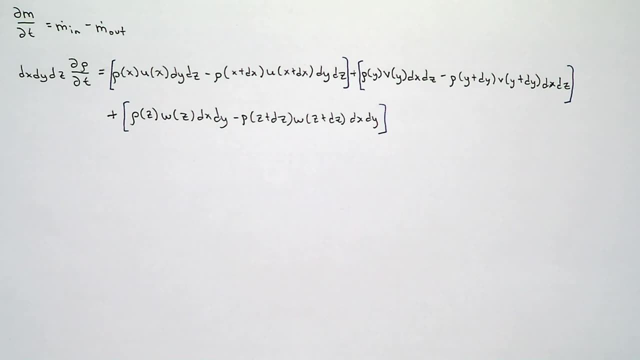 z and – we'll have two more at x and z, so we need 2.ểm at each of them. x and z components get density at z times velocity at z dxdy minus density at z plus dz times velocity at z plus the z. 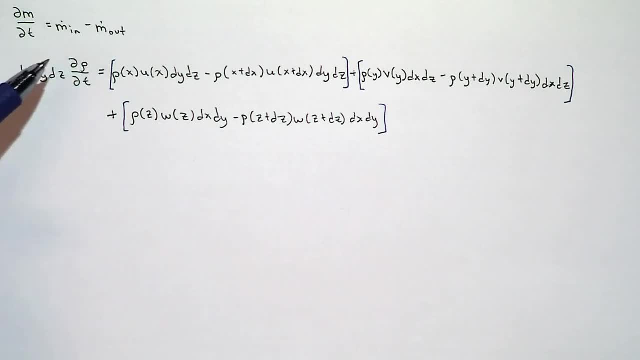 obtagnexed: y, y minus density at z plus dxdy minus density at z plus dz. times velocity at z plus ughjoey difficulty x, dy. look at how easy i made this equation. we had a very, very arbitrary equation that we have now simplified into something we 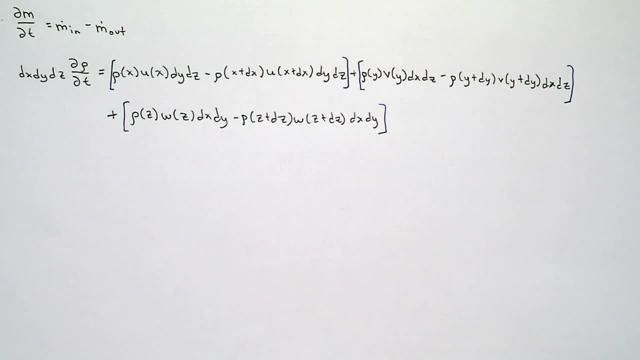 can use what, haha. so why do I do this? the whole point of this exercise is to create an equation that doesn't vary with the volume. we don't want to care about the volume of the control volume, so what can we do to this equation if we 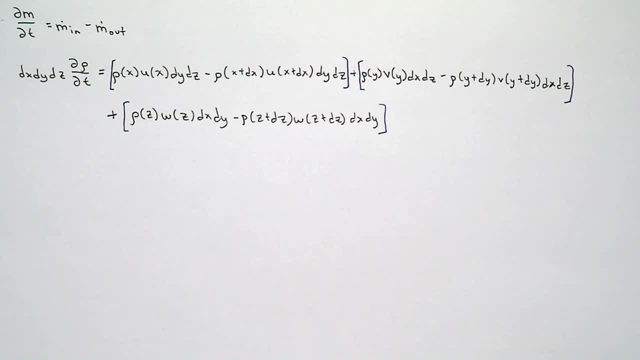 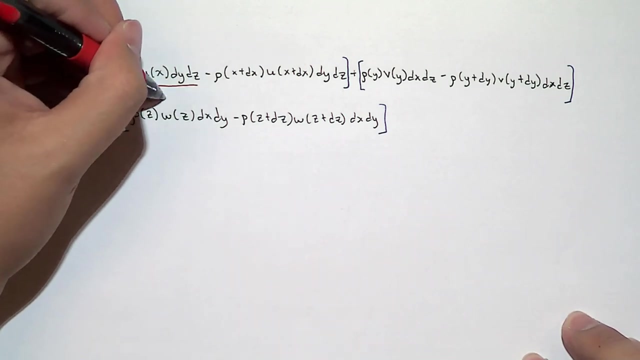 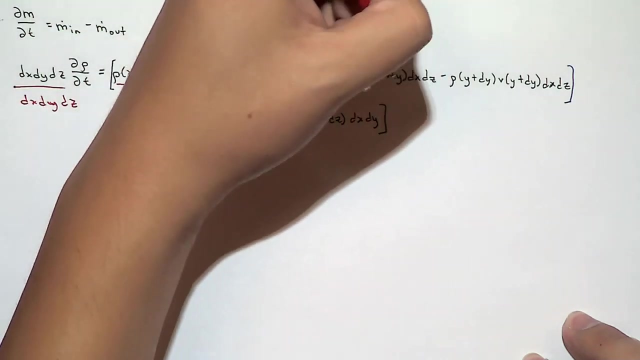 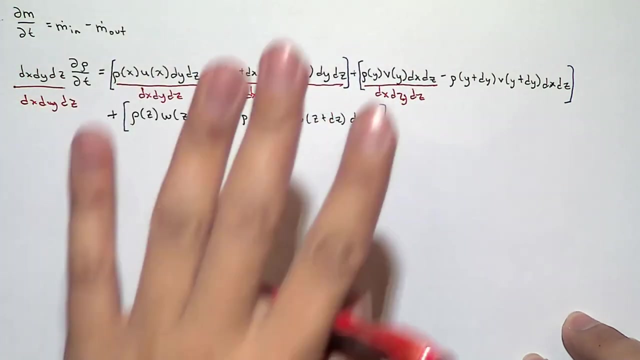 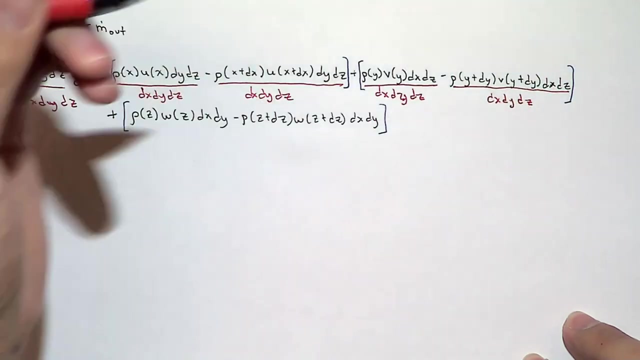 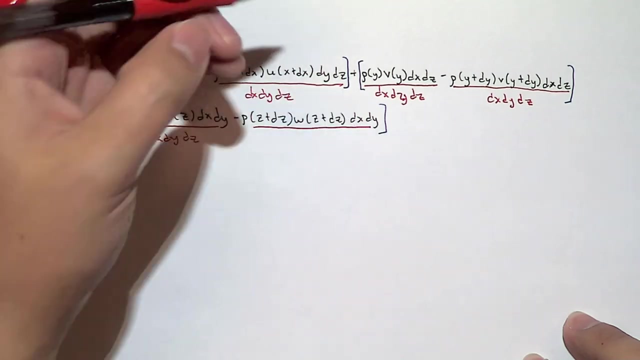 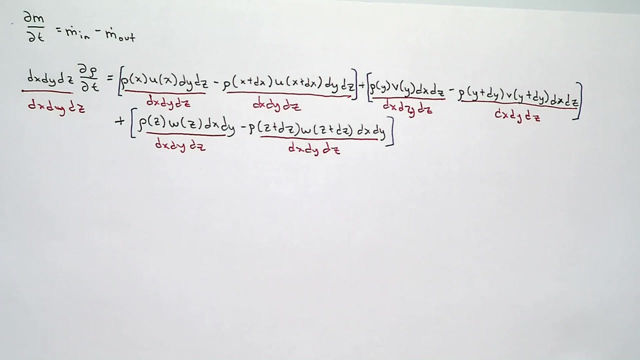 don't care about the volume exactly. we divide both sides by volume. okay, hmm, I forgot my wedding ring. I'll have to edit that. in the video you'll see a very badly edited CGI wedding ring. okay, and what happens here? well, look at this. we have volume divided by volume. 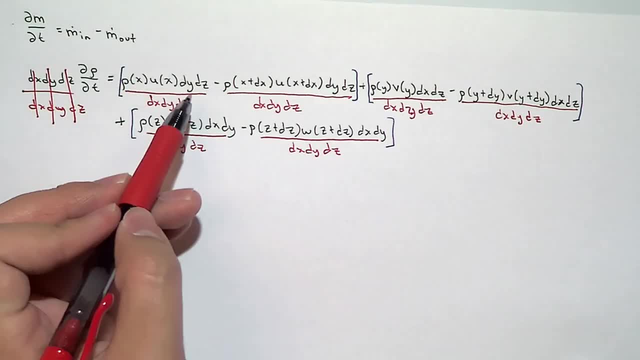 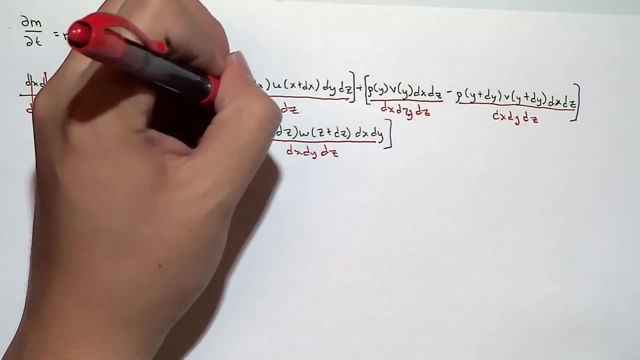 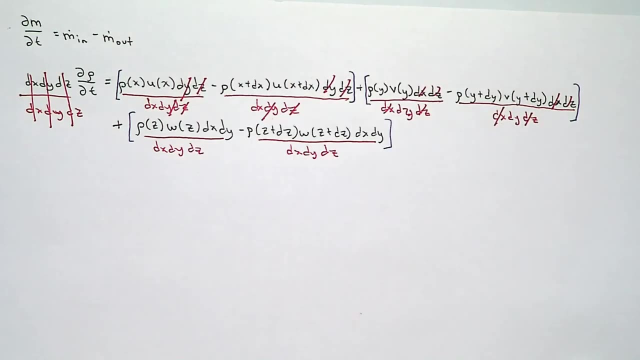 it just cancels out. we have dy and DC. okay. and what happens here? well, look at this: we have volume divided by volume, which cancel out. we have dy and DC, which cancels out. we have DX and DC, which cancel out, and then we have DX and dy, which cancel out. and now you'll see that. 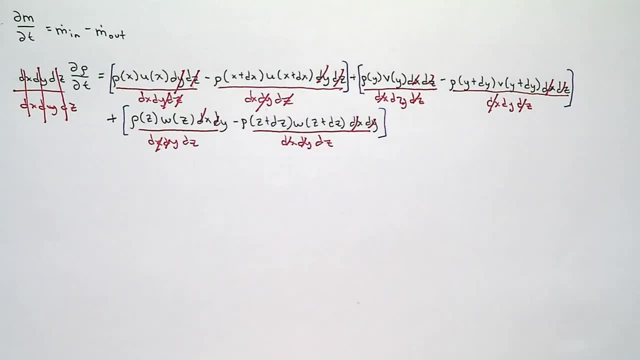 my equation will start to look a little bit easier to manage. we get that the partial change in density with respect to time is equal to, and actually notice that because both these terms have DX in the denominator, I can combine them right, so I'm going to do that. this will be equal to density at X times velocity at. 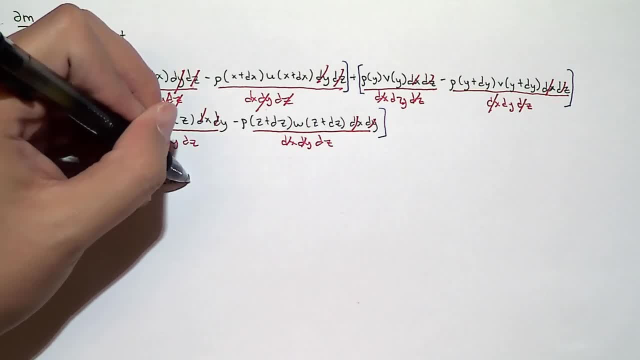 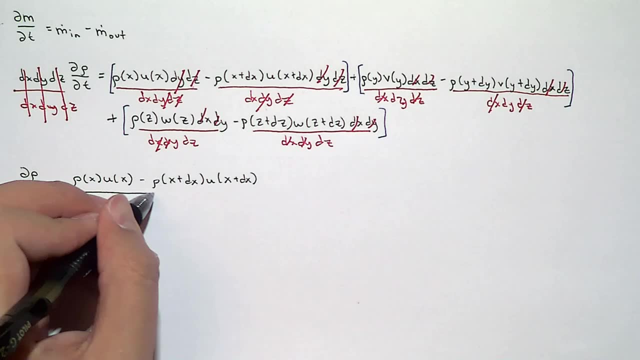 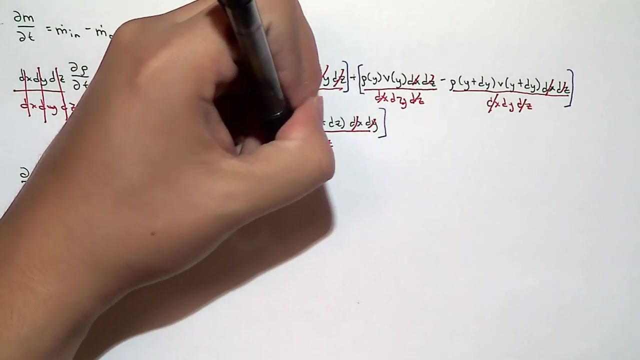 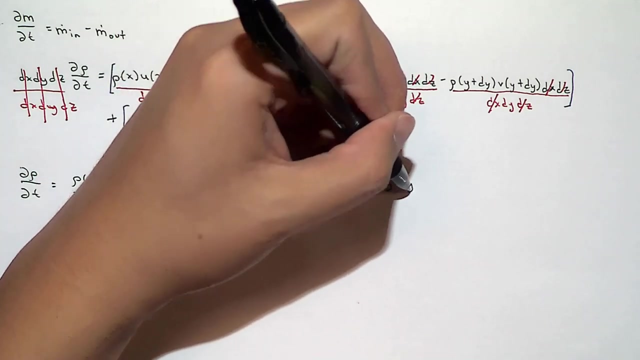 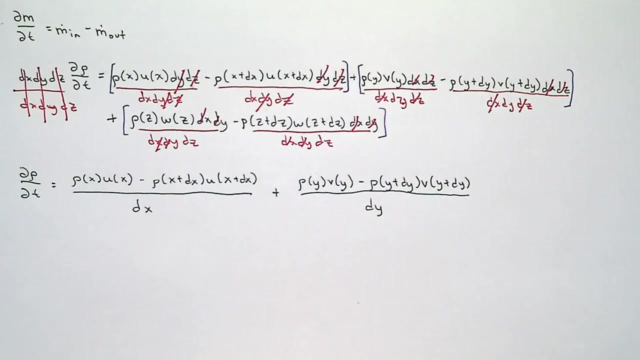 X minus density at X plus DX, times velocity at X plus DX, and all of this is divided by you, I DX. likewise, we have density at Y, velocity at Y minus, density at Y plus dy, velocity at Y plus dy, and all of this divided by dy. and finally, density at Z. 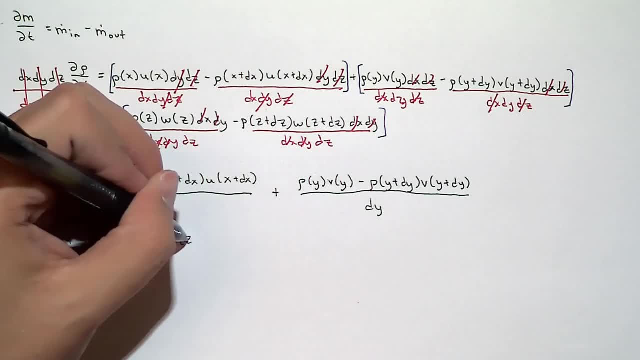 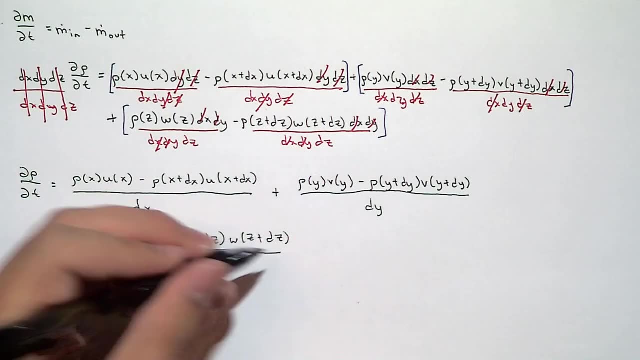 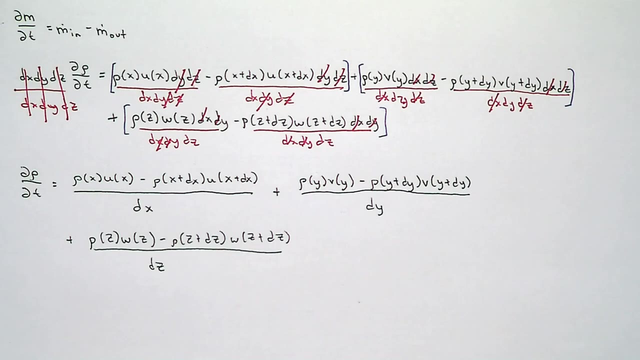 velocity at Z minus density at Z plus D Z. velocity at Z plus D Z. and all of this divided by Z. and why am I doing this? look at each of these three terms and perhaps ignore that we're talking about density and velocity. let's just think of density and velocity as some arbitrary function. what 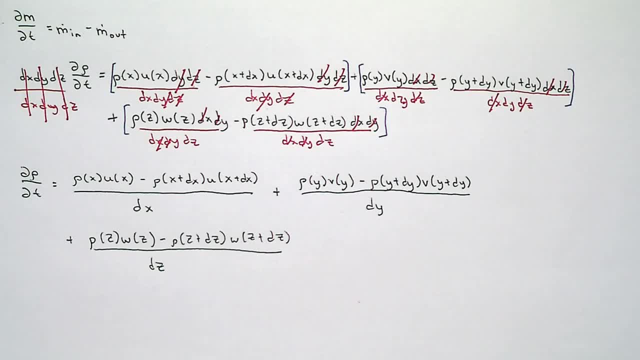 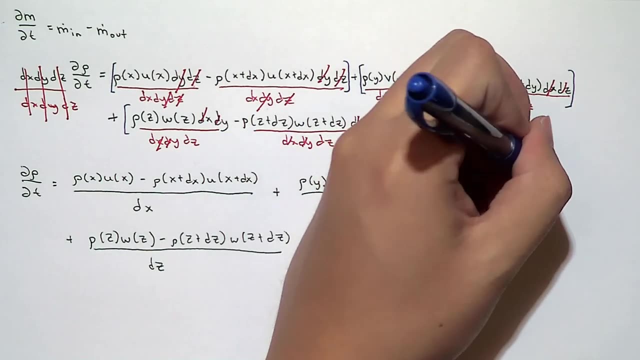 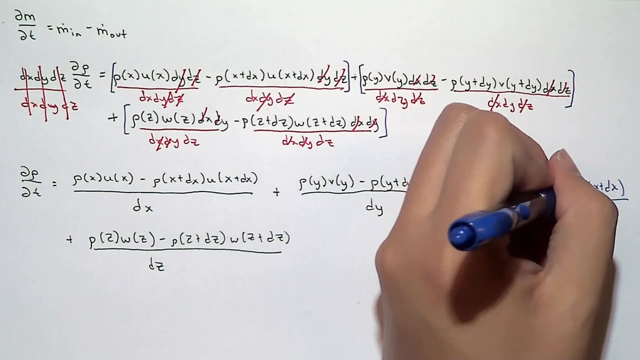 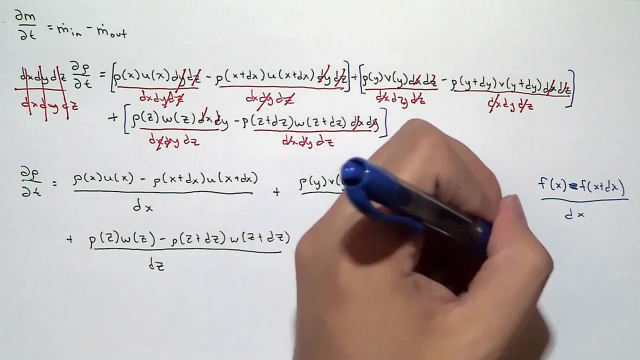 do you think these terms represent, so- density and velocity- as some arbitrary function? what do you think these terms represent so that we can't just call it a function? let's just say that, in ignoring that this is density and that this is velocity, let's just call it a function. right? so we have a. 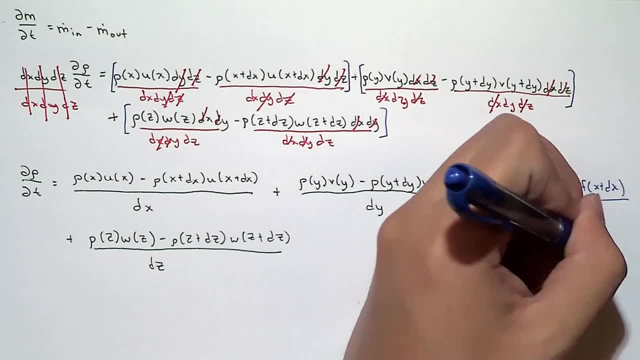 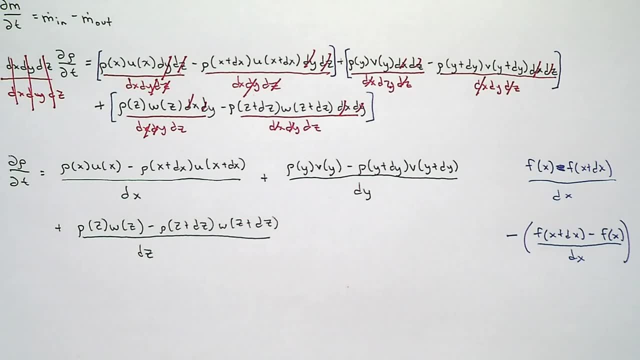 function of X plus a function of X plus DX, divided minus divided by DX. in fact, of x divided by what exactly? and what do we call? change the derivative. notice that this is just a derivative of X, F with respect to X and notice that: what is this? what is this function? well, the function is just density times velocity. 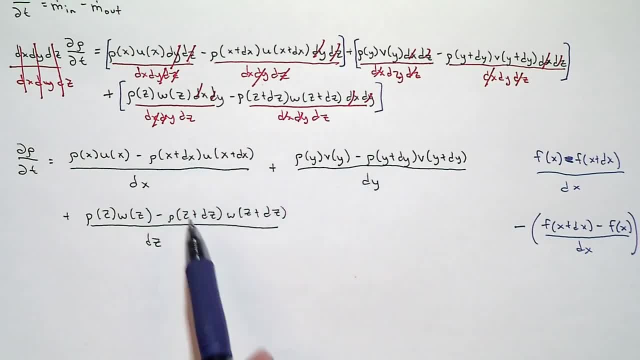 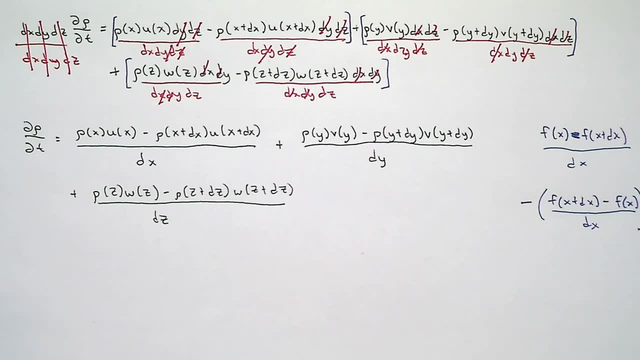 so what we're looking at here are three derivatives: the derivative of density and velocity with respect to X, density and velocity with respect to Y, density and velocity with respect to Z, so we can write this equation as simply negative. the partial derivative of Rho u with respect to X, minus negative. the partial 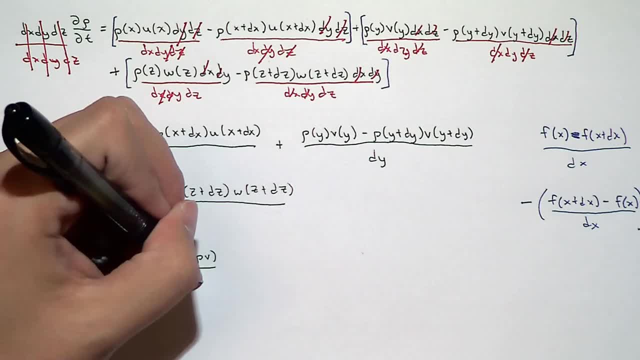 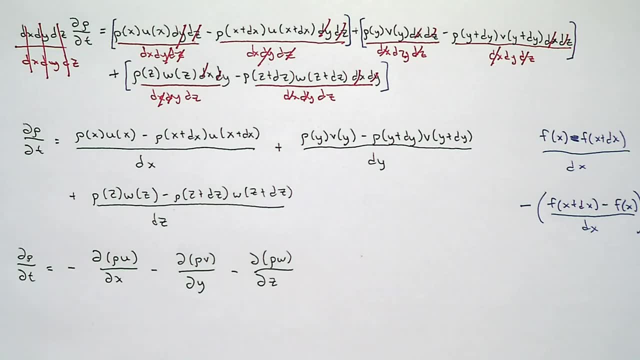 minus the partial derivative of Rho B with respect to Y, minus the partial derivative of Rho W with respect to Z. and what is this? what have we seen this before? the derivative of something with respect to X plus the derivative of derivative of something with respect to y, plus the derivative of something with respect to z is: 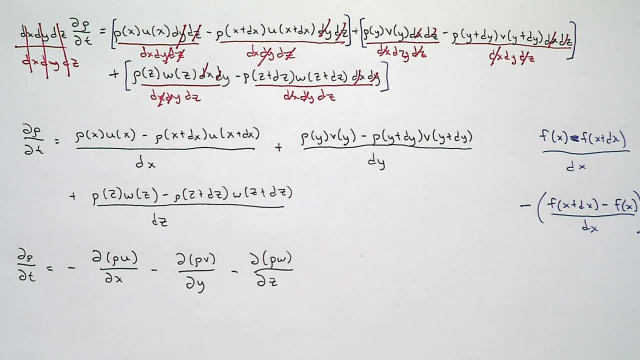 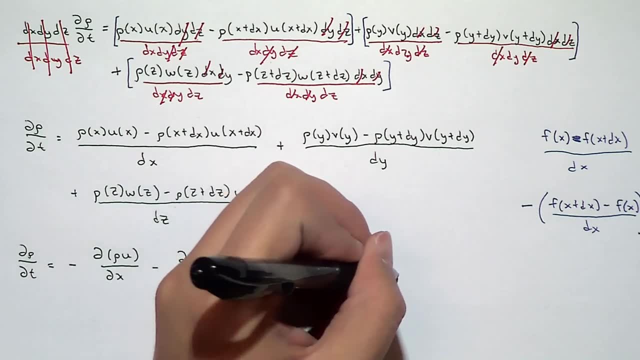 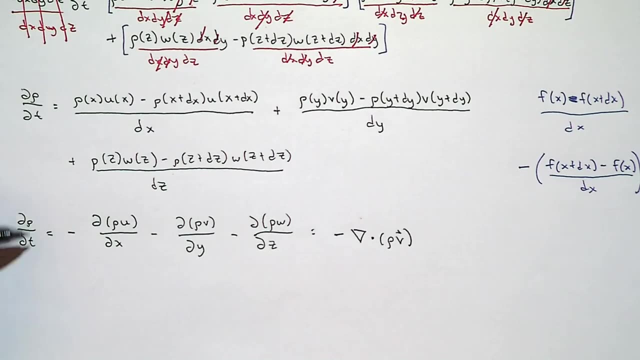 what the divergence? right? yeah, so this is actually equal to negative. the divergence of density times, my velocity vector. i can rearrange by moving this to their side and i end up with the change in density with respect to time plus the divergence of density times, the velocity vector equals what?